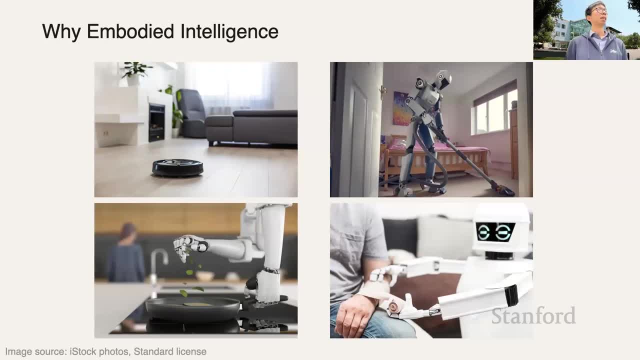 us or taking care of our aging family members. So we are not quite there yet. In fact we are quite far from it. So we might see bad reproduce today. 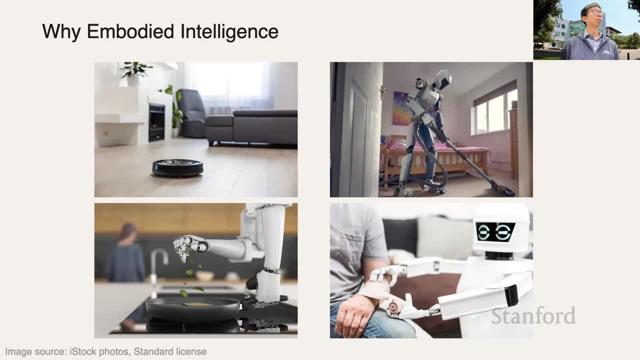 On this day. alien intelligence is currently mostly in the virtual world. So we have an AI agent that can help us draft emails or write eloquent essays, But they are not super good at interacting with the messy real world, unstructured, complex environment that human. 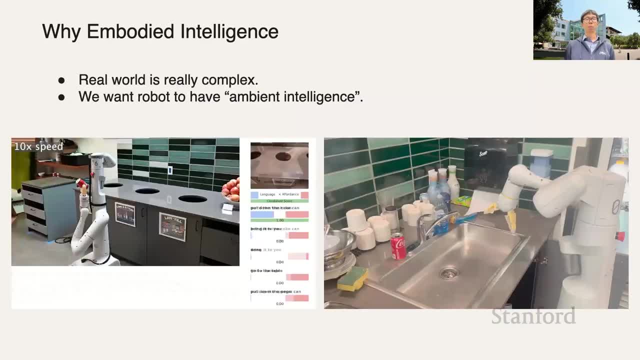 resides in. So just to give you guys a couple examples of how messy the real world can be and how hostile it could be to robotics, I want to show you a curious mystique or a curious error within the robotry Cena application. So first of all, I think it's worth mentioning that 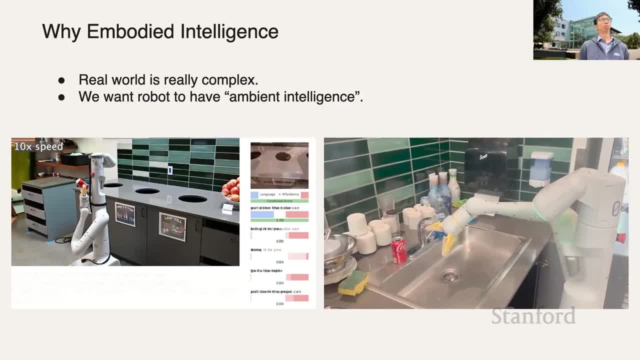 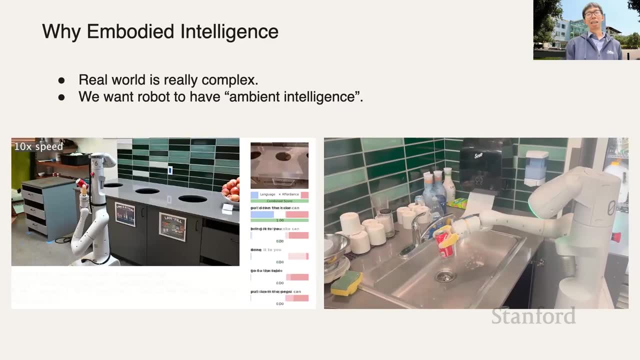 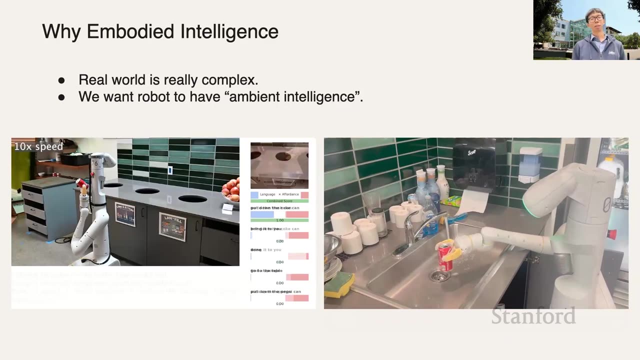 error from one of our robots. So the task is to put the Coke can in the sink and watch what the robot do. The robot grab the Coke can and open the tap. So this is kind of dangerous, but it's kind of interesting. 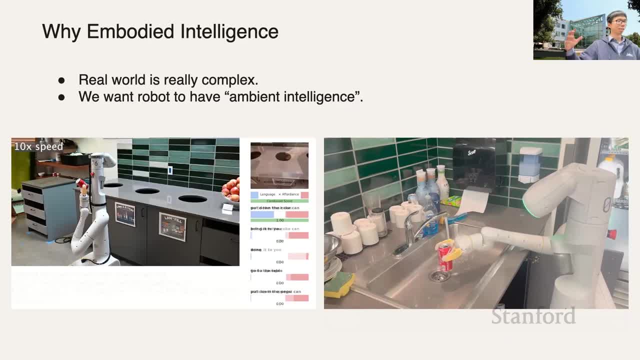 because we never expect it would do something like that. It's just from random noise. it starts to open the tap and the water starts to come out. So for an agent to have this type of physical intelligence, they need to understand the effect of its actions. 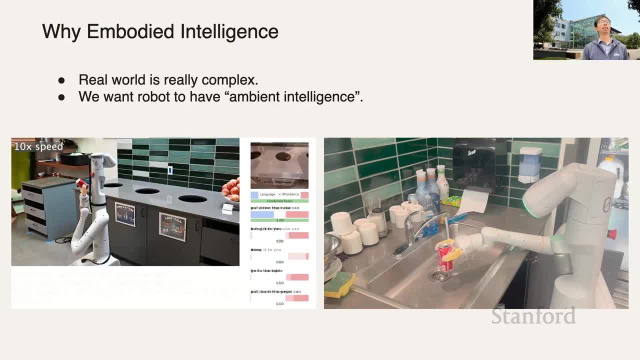 and what is so-called a world model. So people have been complaining that language models so far don't have a world model. So it doesn't understand geometry. It doesn't understand the spatial relationship of objects or the effect of actions, basically how objects will move according to physical laws. 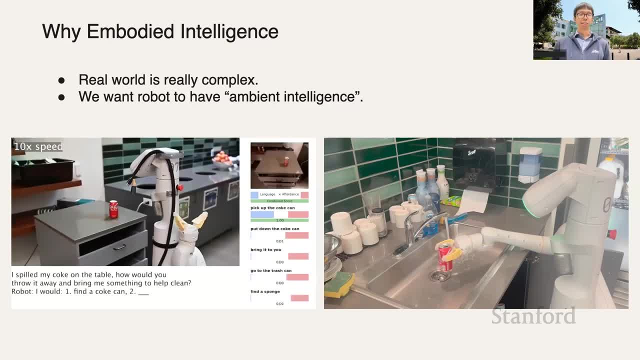 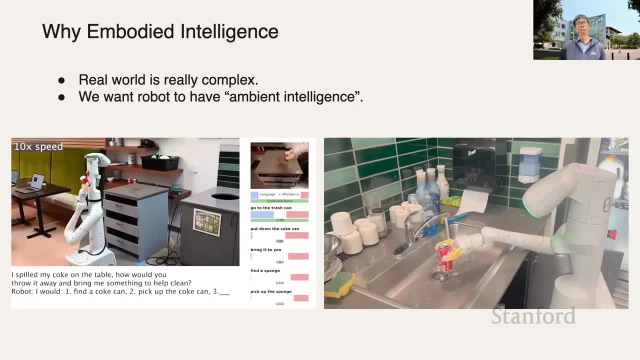 So we are not quite there yet In another case. so this is our robot that is ready to deliver a can, or actually throw away a can, But, as you can see, we have this pre-programmed behavior of tucking the arm behind. 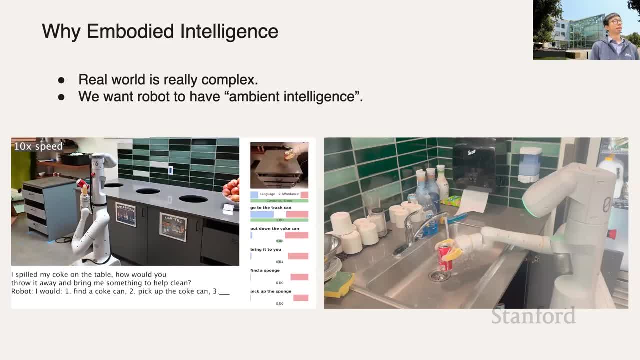 And in doing that the can is upside down. So if there is any liquid in the can it will spill and damage the robot. So it's another example of real world is really complex and there are a lot of things to model. 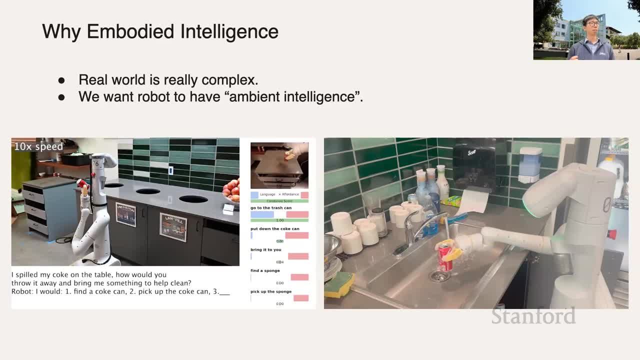 And in order for our robots to have this sort of ambient intelligence, it really needs to understand a lot of very nuanced details of the environment and understanding the physics, physical laws and understanding effect of its actions. How do we do that? There are many ways to achieve embodied intelligence. 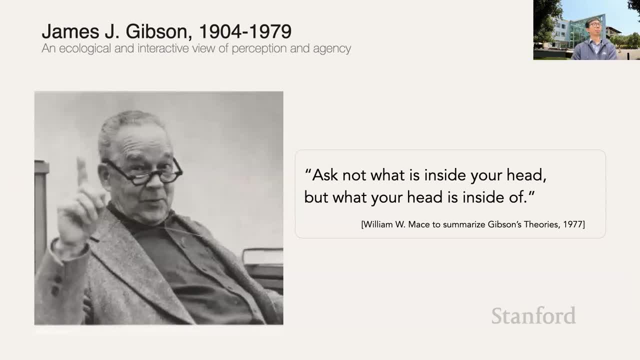 Actually, throughout my PhD study, I've been fascinated by this idea of creating interactive environments. basically let agent explore in this interactive environment, basically Create environments that are complex enough so that if the agent needs to survive in such an environment, it must develop intelligence. 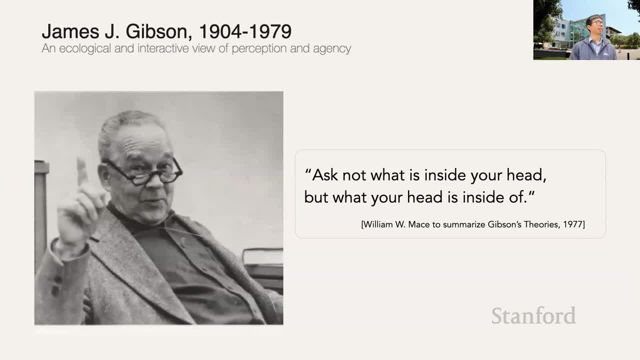 So it's an ecological view of perception and agency, and it's popularized by American psychologist James J Gibson. So he has a famous quote: ask not what is inside your head, but what your head is inside of. So humans learn this type of embodied intelligence. 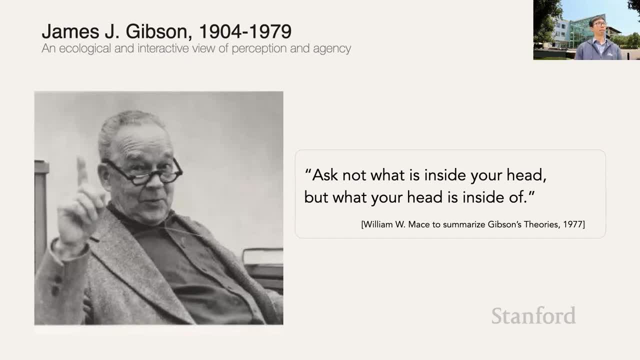 A human is able to manipulate the object, to manipulate the object effortlessly. one because of evolution. second, because the childhood experience. We have been playing with this toy. We have been interacting with this toy and watched the physical effect so that we learn. 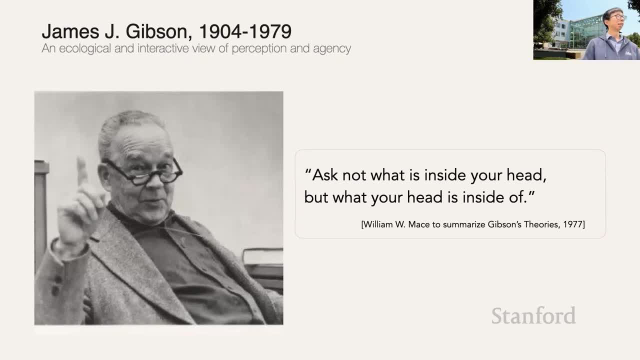 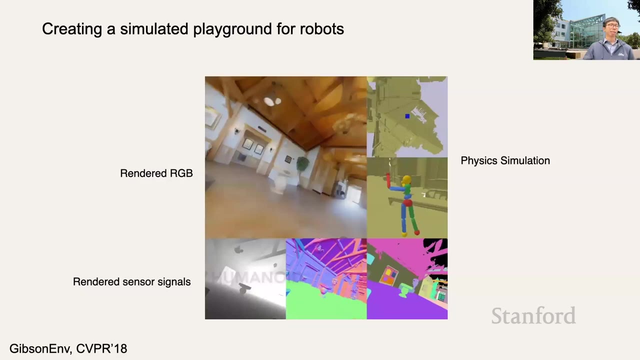 And similarly we can give robots a safe playpen so they can explore in those environment and interact with the environment and play and watch the effect of actions and effectively understand how to manipulate those objects, So developing these simulation environments, one of which is called Gibson Environment. 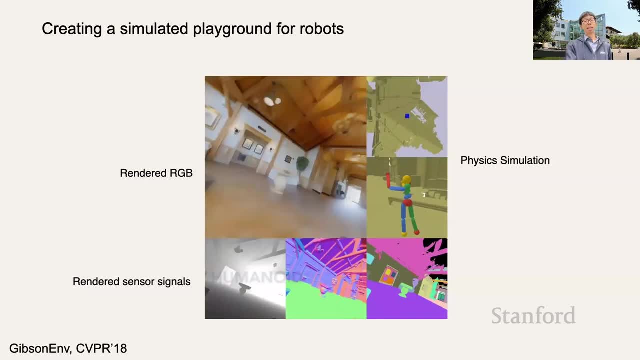 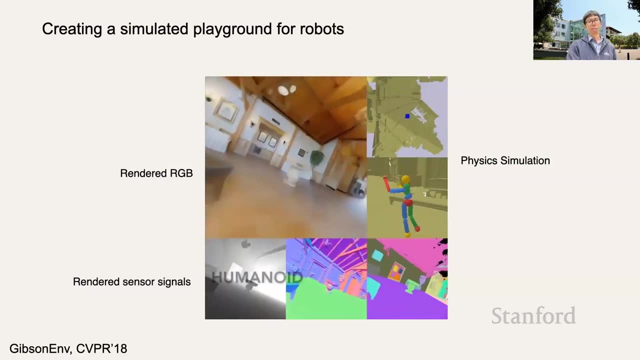 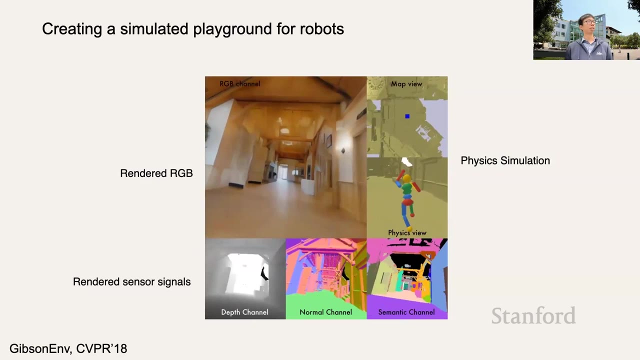 which is published as CVPR. it's mainly aiming at simulating the visual world faithfully and also simulate physical world to some extent. So we built this environment, which is a scanned environment from a lot of houses, And then an agent. we can spawn an agent in that. 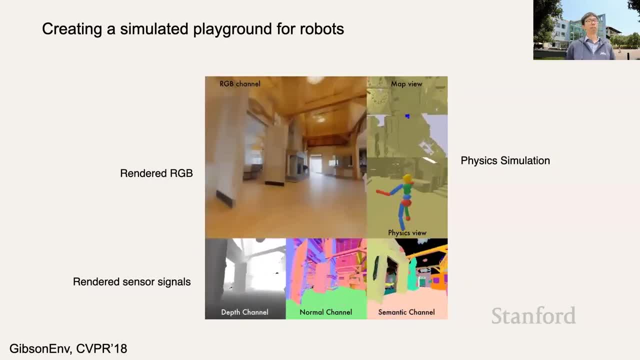 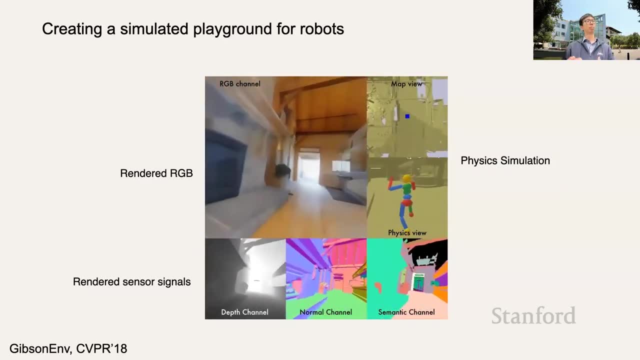 in this case a humanoid agent, and the agent can learn, learn, learn, learn, Learn to walk or to run in this environment- and simulate all this perception information So we can create a perception action loop for this agent And similarly we can put other types. 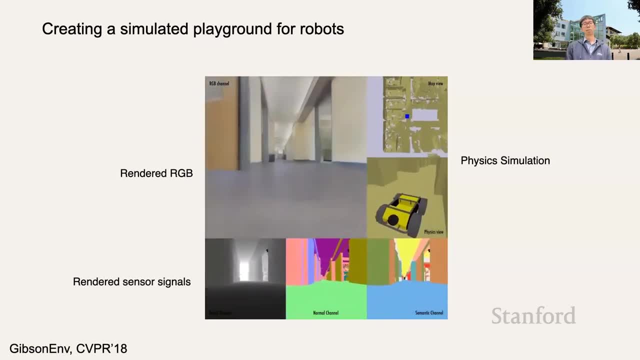 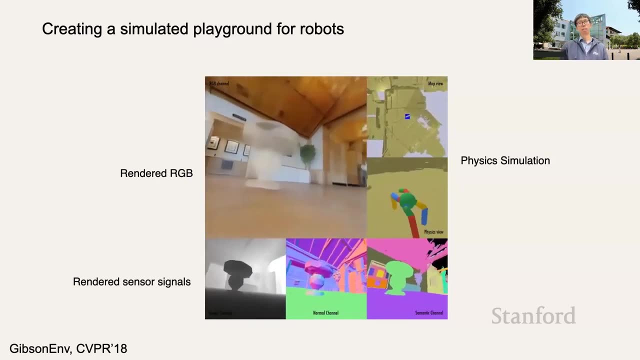 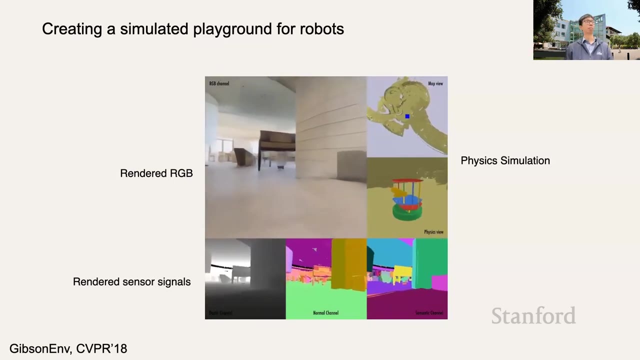 of agents in this environment, in this case a little cart, And we can also put quadruped or this ant into this environment. So essentially we create an environment where we can simulate perception for the agent And then we can, We can create a neural network to map the perception to action. 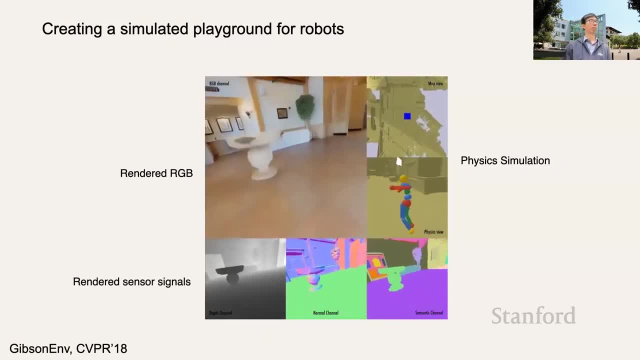 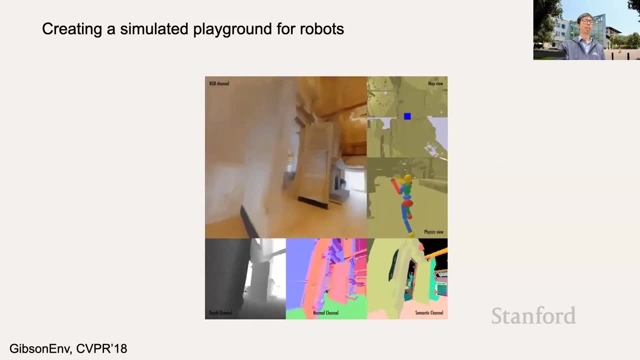 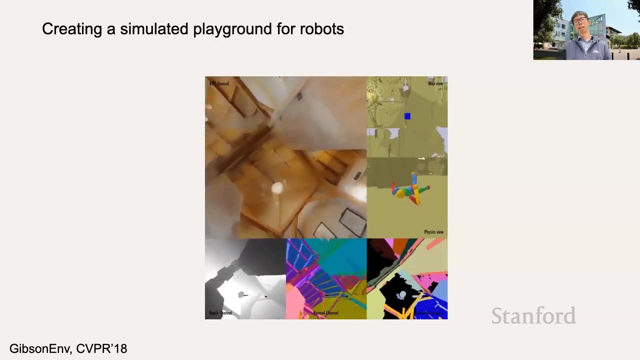 And this way we achieve some sort of physical intelligence. It's mostly for navigation and locomotion. This is not enough. So in this case the environment is one monolithic piece of mesh. As you can see, the agent run into the wall and it bounce back. 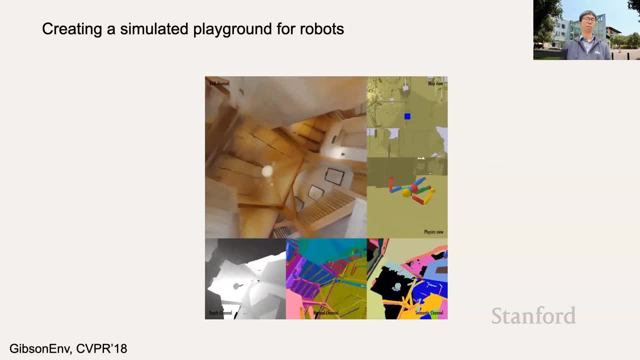 So there is no articulation in this environment, So it's not simulating the full complexity of the environment. So it's not simulating the full complexity of the environment. So the things that we can do with our agent is rather limited. So that's why we create other simulation environment one. 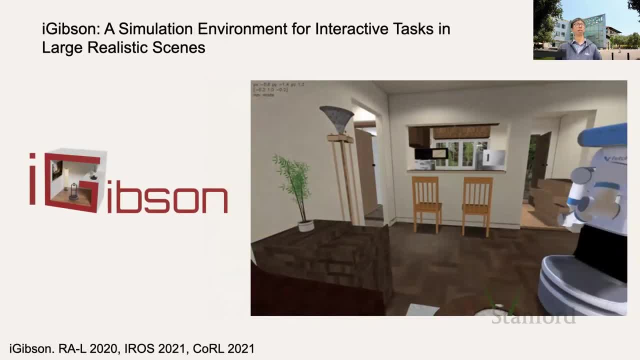 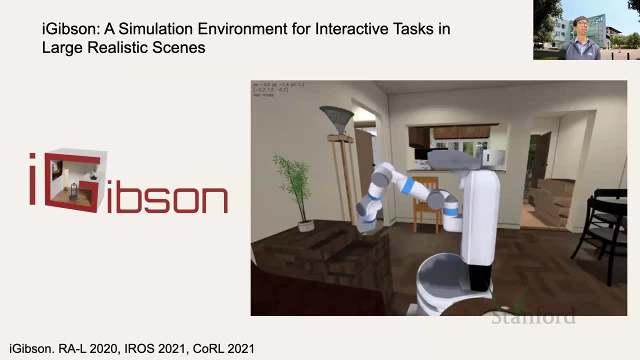 of which is iGypsum environment, which is called InteractiveGypsum. So what we do is we create, again scan, a lot of real world houses And then we convert them to CAD assets, basically mesh assets that are interactable. In this case we have a simulated agent. 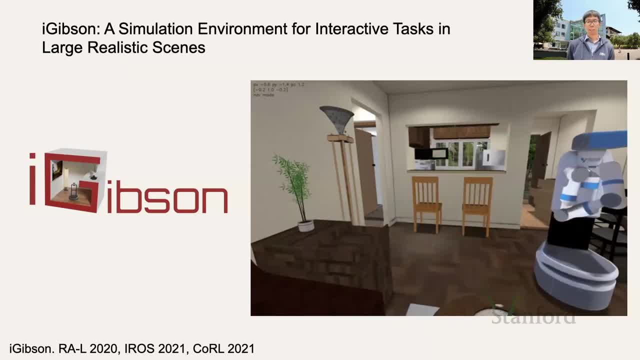 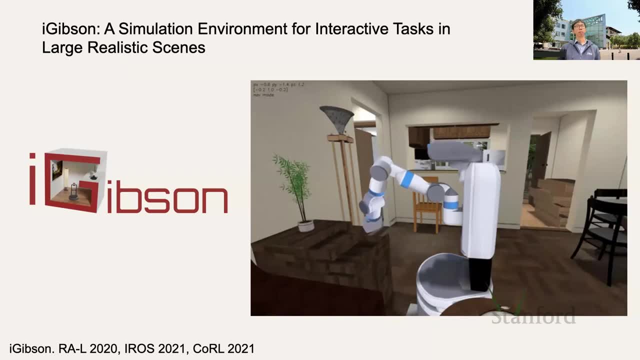 that go into the environment and then close, Close all the doors. So we are able to do that because we model the complexity of the world a little bit more. We go beyond just modeling the visual world. We start to model physics a little bit more. 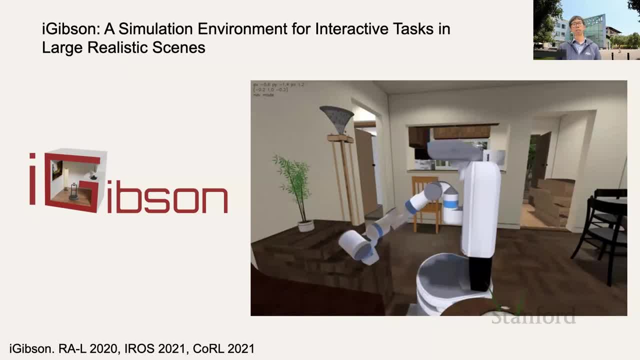 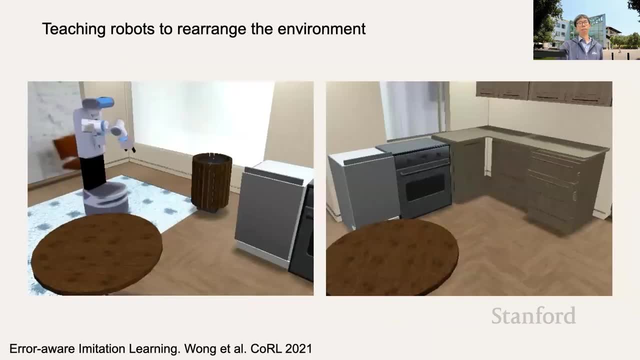 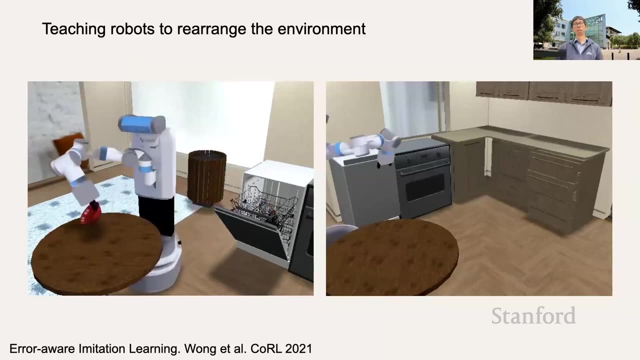 basically modeling the degree of freedom in the environment, And our agent can do more than just navigating around. So we can go even further. So we can even model more degree of freedom, And our agent can develop more complicated behavior, such as unloading a dishwasher and find a bowl. 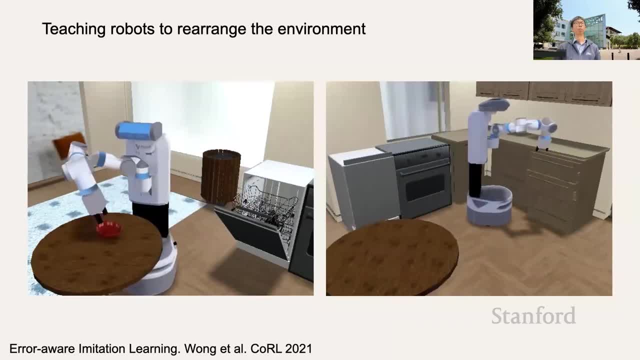 or take out the bowl and put it on the table. So as we scale up the complexity of the environment, we are able to learn much more complicated skills in simulation, And that's one way to achieve embodied intelligence, which is to build complex enough simulation environment. 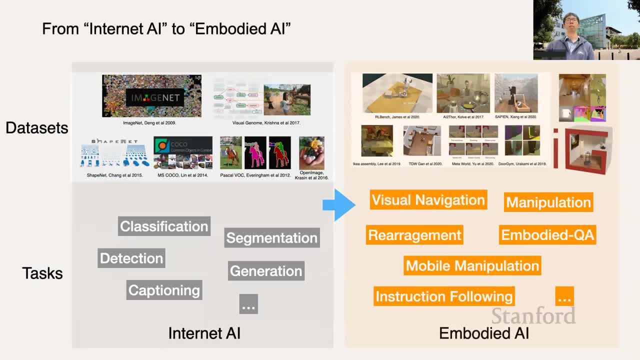 Not just in my research, but the entire field of computer vision is undergoing A paradigm shift. So previously we are focusing on internet AI. We curate a lot of internet data sets to study problems like classification, segmentation and detection- basically all these computer vision problems. 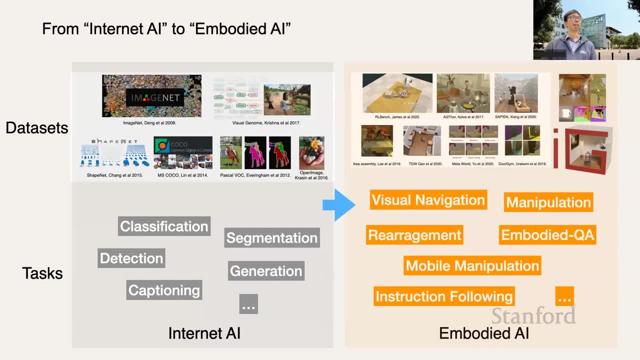 Now we focus a lot more on embodied AI, which is adding the action dimension to the problem. We are studying problems like visual navigation, manipulation, rearrangement, embodied question answering, instruction following, And the simulators in some sense replace the original role of data sets. 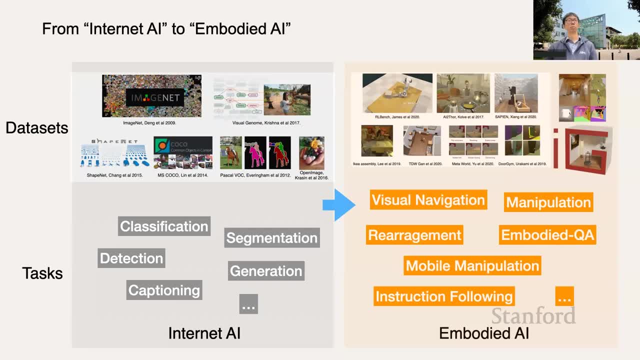 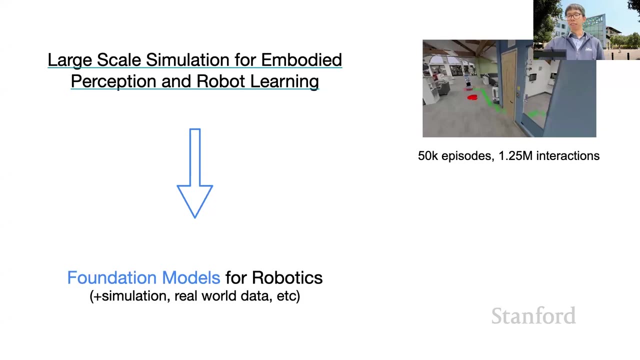 One thing that doesn't change, which is the data is still super important. We are still relying on a large amount of data to learn this intelligent behavior, no matter if it's from a static data set or from a simulator, So learning in simulation can take a lot of interactions. 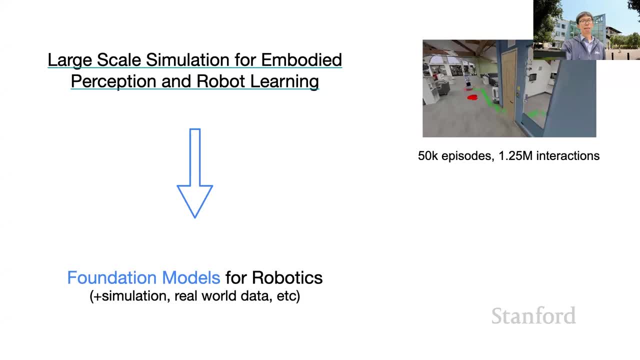 So, just to give you an example, we create this iGypsum environment and we want to learn a behavior called go into a room through a closed door. So this is a rather simple behavior which I can show on the top right of the screen. 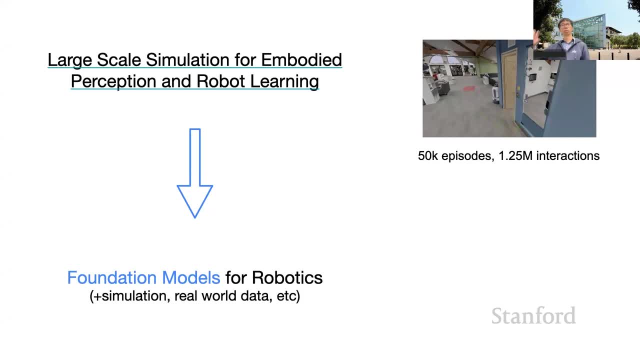 So the agent needs to stop in front of the door. It needs to stop at the right distance. If it stops too close to the door, it cannot extend its arm. If it's too far, it cannot open the door. And then it basically opens the door. 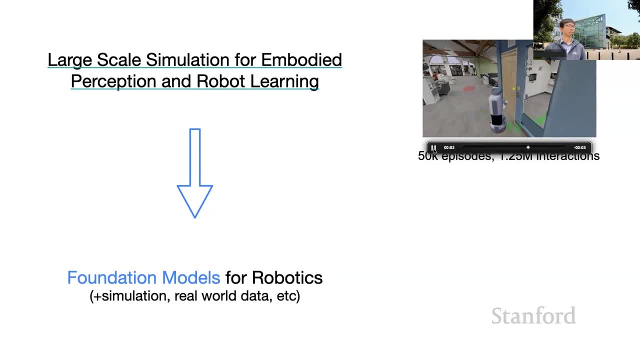 Let me play this again: Open this door. When there is enough clearance, it will go into the door. However, it takes about 50,000 episodes or 1.25 million environment interactions to learn this type of behavior. This is because we are using model-free reinforcement. 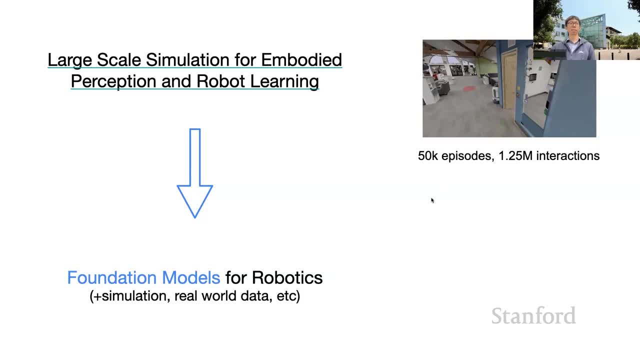 learning. The agent is exploring this environment. It could really push any point. It could rather stop at any point. So we give it a rewards function to go into the room, but it's very rare that it will stumble upon this behavior. I would like to argue with foundation models. 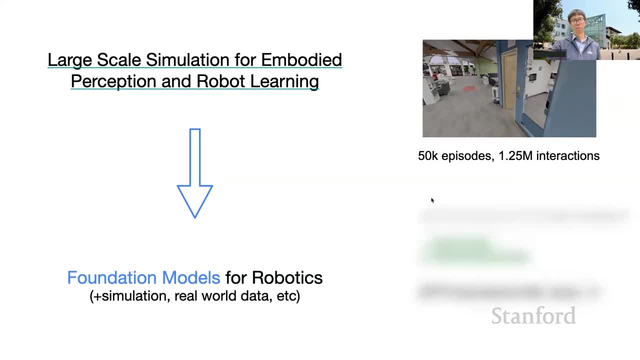 we can do a lot more different, right? So what do you do nowadays? You just ask a chadgbt: How do you go into your rooms through a closed door? And it will say: open the door, walk through the door. 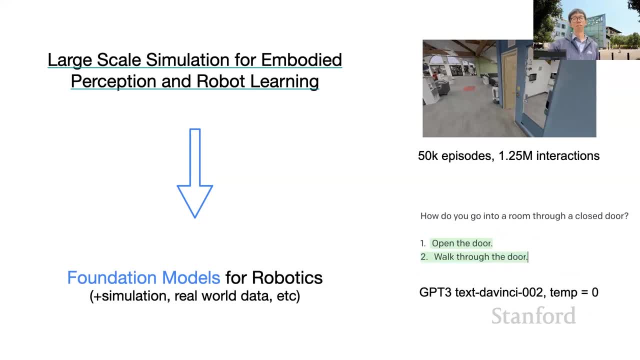 So this is a gross simplification of the problem. Of course, the problem is not that simple, But what I'm just saying is that we can leverage a lot of semantic prior from the foundation models. So if we really like data, if we really need a lot of data, 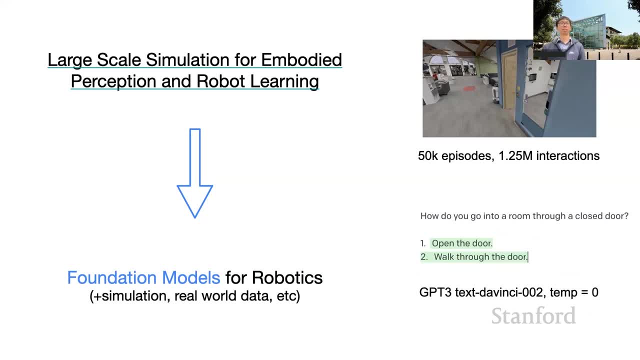 the foundation model is a compressed version of the entire data and it's a knowledge base that you can query and to accelerate the development of robotics. Of course, simulation and real-world data is still super, super important, but maybe we can get the best of both worlds. 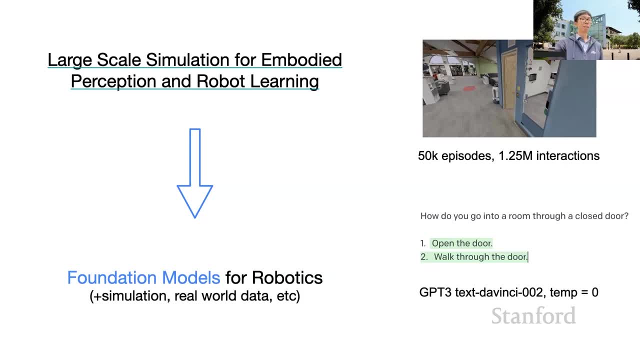 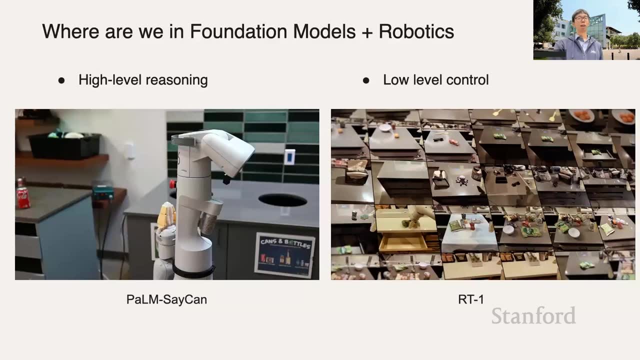 We can use foundation models plus a limited amount of simulation or real-world data. So that's what I'm going to talk about today. Okay, so where are we in terms of foundation models plus robotics? So our team at Google DeepMind has been piloting. 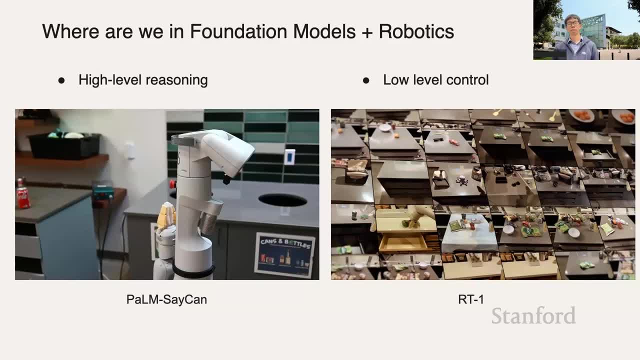 in foundation model plus robotics. So we developed advanced planning, high-level planning algorithm. One of the first is called POMSACAN. It is an algorithm that can parse a user command. So here is a demo, Here is a scenario. 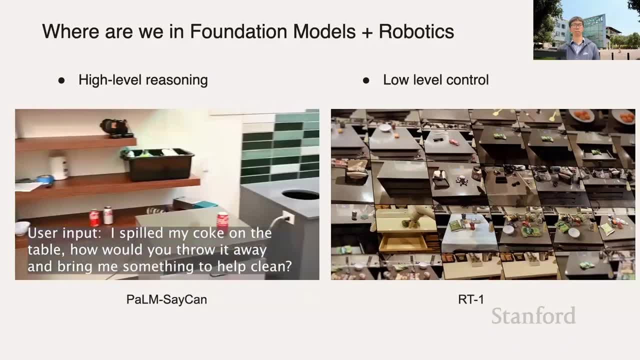 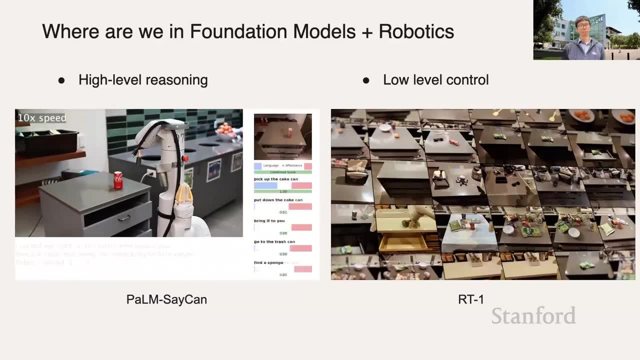 Here is a user command. I spill my Coke on the table. How would you throw it away and bring me something to help clean? And it's querying a large language model which is given a score highlighted in blue, And there is also a fordance score. 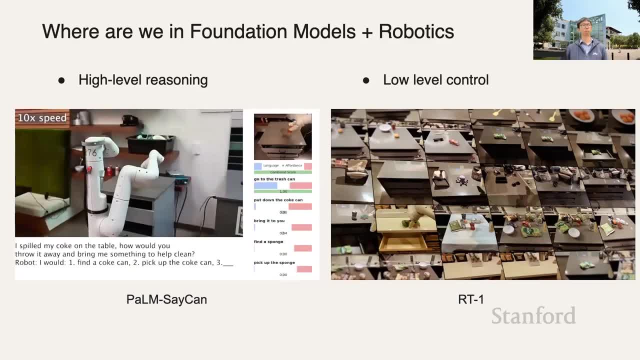 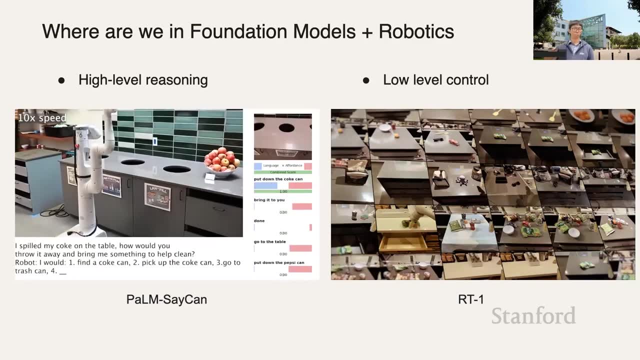 The fordance will tell you whether an action at a given state is possible. It's augmenting the language model to give you only possible things. So essentially it is doing the planning, doing the semantic planning with a language model, but it's also taking into consideration what it can do. 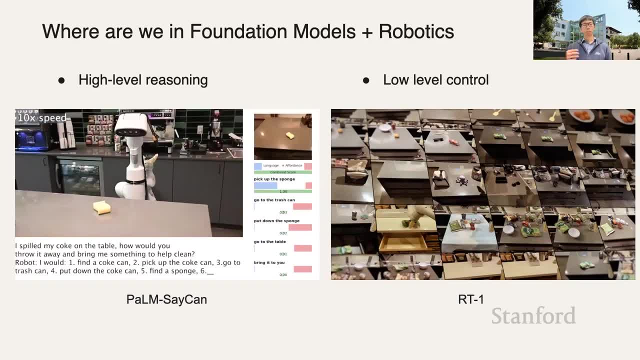 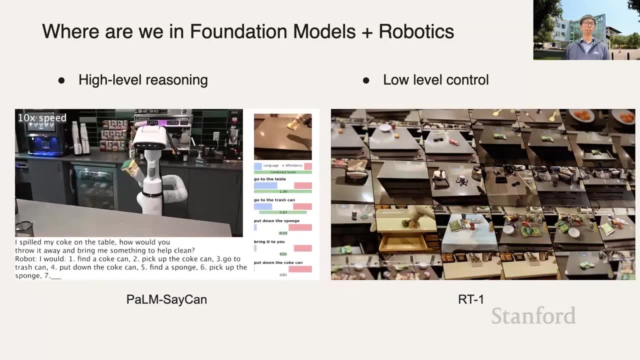 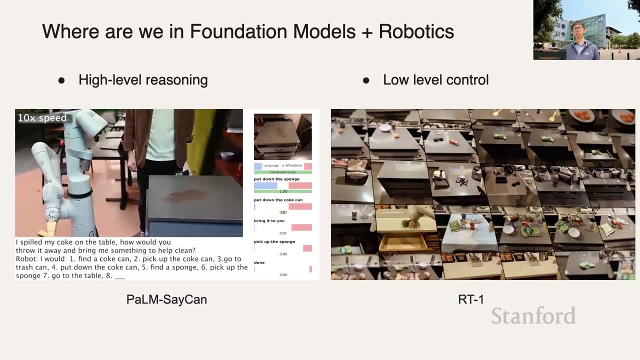 So it's not just outputting the language like language model are tend to hallucination. It doesn't hallucinate, It only give you what is possible for the robot to do and what is actionable for the robot, And the robot is doing the thing that is, advancing the long horizon task progress. 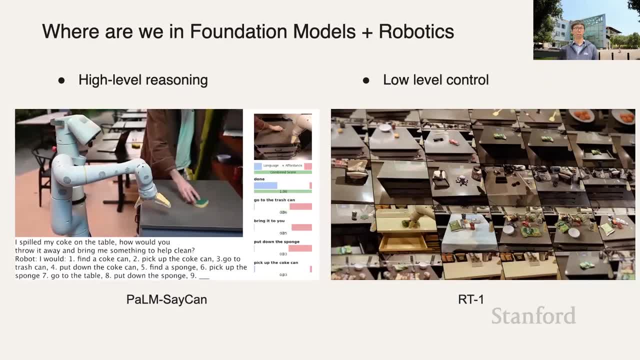 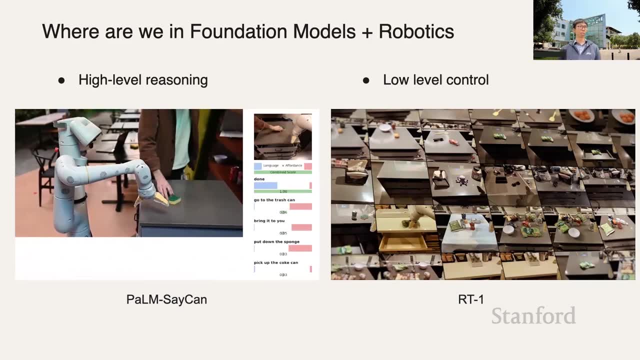 And also each task is executed by a low-level policy. Here it doesn't quite clean the table because we haven't added this to the low-level skill, But imagine there is a low-level skill to clean the table. It will finish the entire thing. 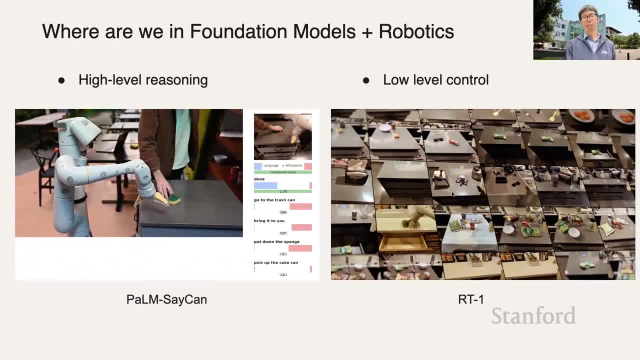 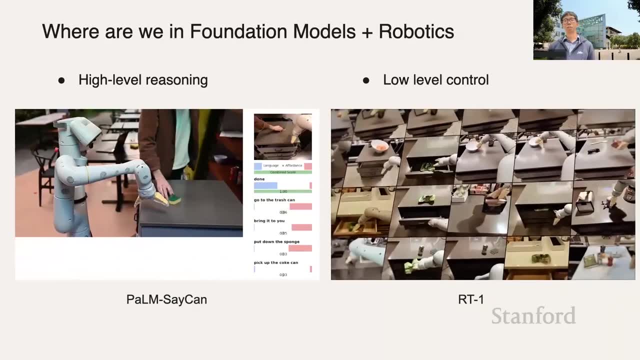 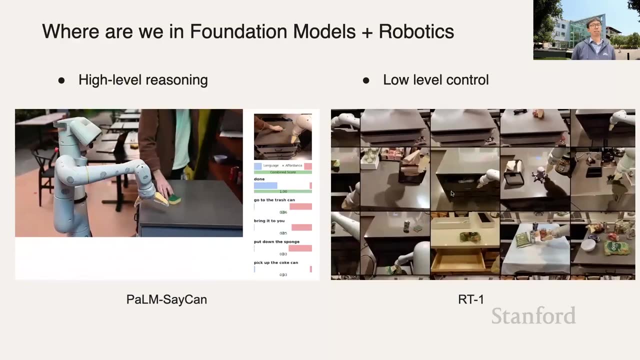 What is a low-level policy used to here? The low-level policy used to here is Robotic Transformer 1, RT1.. It's our team's homegrown transformer. Essentially, we collect a large data set of human demonstrations. We put a transformer and we train it on this large data set of expert trajectories. 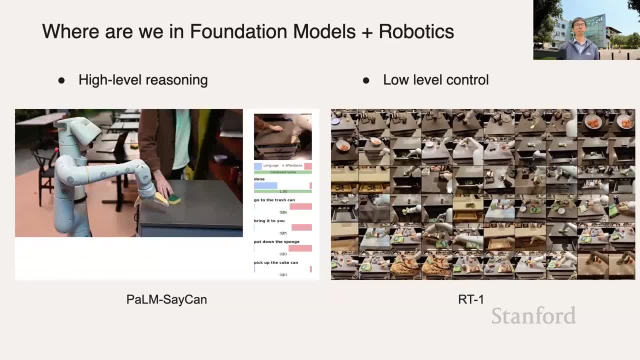 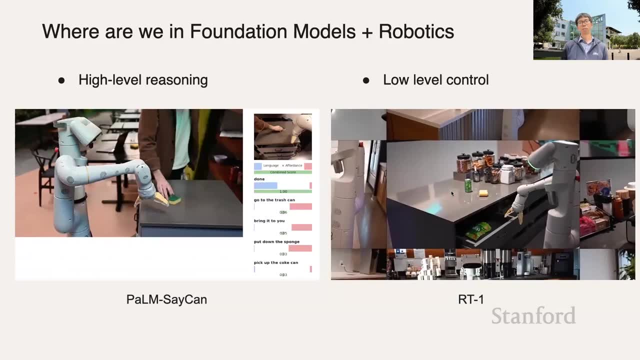 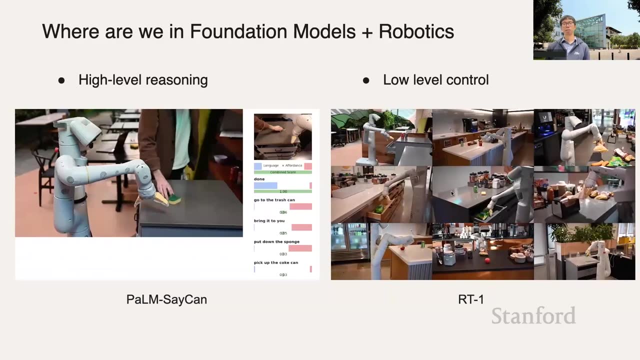 It is able to do about 700 tasks with 97% success rate, So it has interesting generalization behavior. It can operate in a new kitchen it has never seen before, which is showing there is a successful recipe to apply foundation models in robotics. 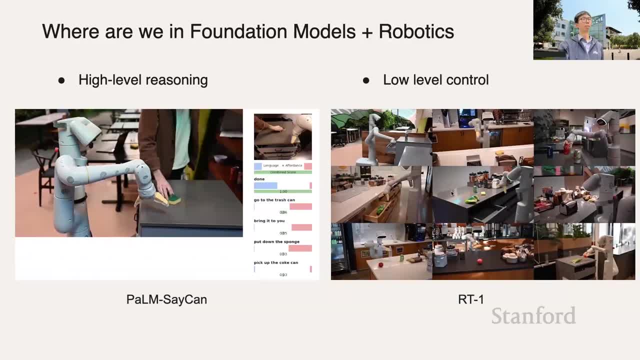 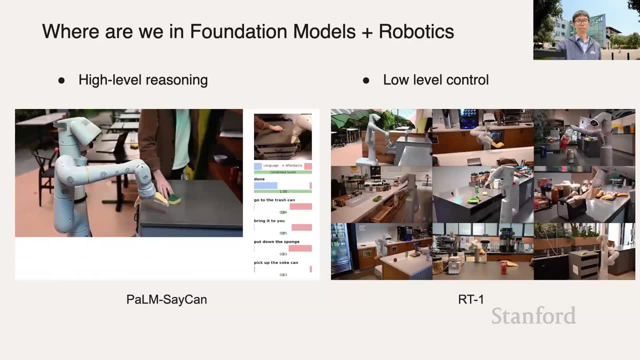 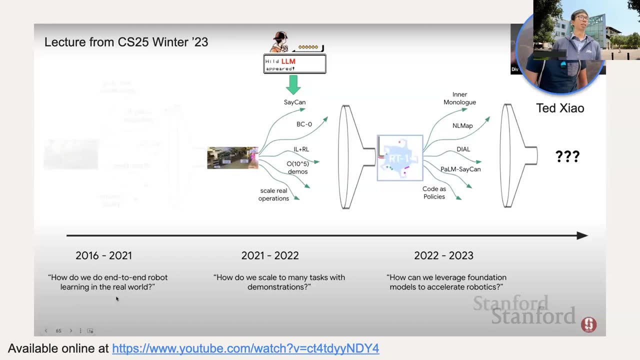 So that's roughly where are we in terms of foundation model plus robotics, And I will talk about a few new works. that is bringing this to the next level. So actually, my teammate Ted gave a talk of foundation models plus robotics at the beginning of this year. 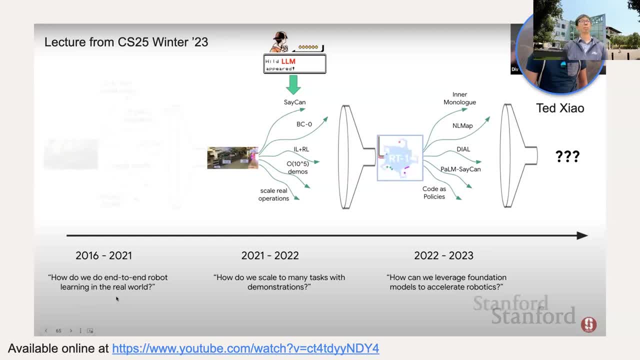 It's also this class, CS25.. I highly recommend it. It's available on YouTube. I actually watched it last night so that I don't repeat some of the contents. But what he basically mentioned is that he revealed our team's progress in terms of building this robotic foundation models. 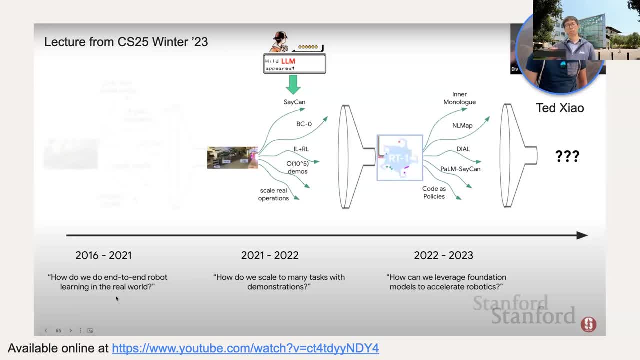 And we have had a lot of somewhat detour And now we sort of figured out a recipe. So in 2021 to 2022 is how we scale to many tasks with demonstrations. How do we collect a large amount of data? 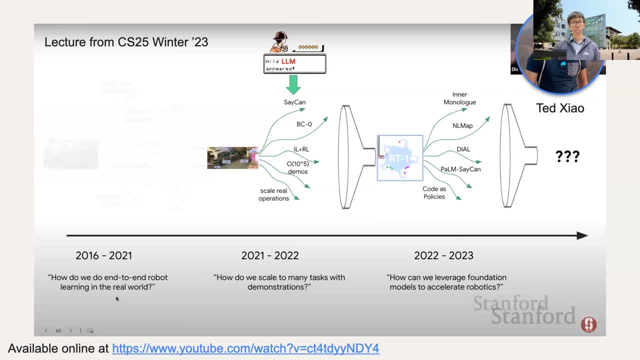 In fact, about 100,000 demonstrations, And we tried different ways to do it. We tried behavior cloning, We tried imitation learning plus reinforcement learning and some other ways, Or combining them with language models. such as SACAN In 2022 to 2023 is about how we can leverage foundation models to accelerate robotics. 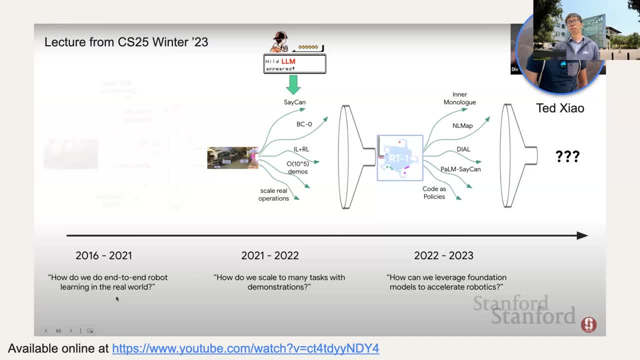 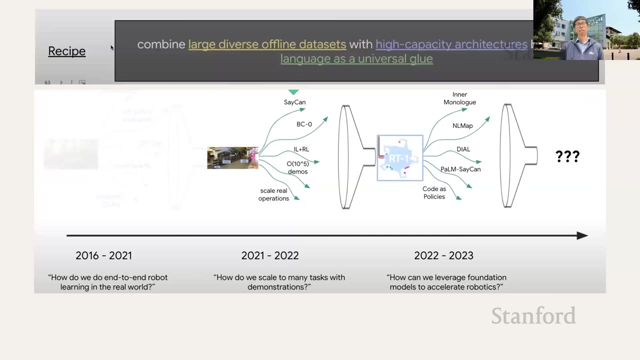 We really see a proliferation of using foundation models to accelerate robotics, Both on the high-level planning and low-level control, Probably leaning more towards the high-level planning. So if the recipe works. So the recipe is essentially combine a large-scale diverse offline data set. 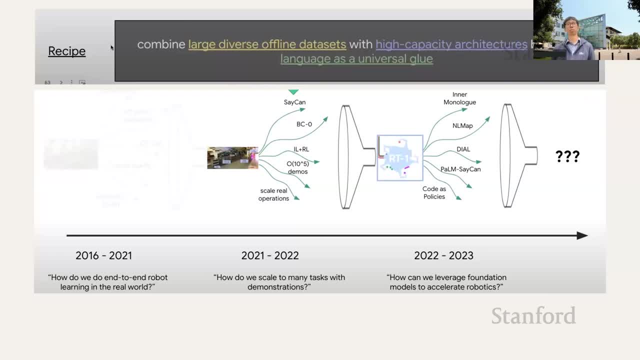 with high-capacity architecture, Such as a transformer, And using language as a universal glue. So this will be the recipe to build foundation models for robotics. So if this recipe works, what do we do next? Essentially, let's just scale everything to others of magnitude. 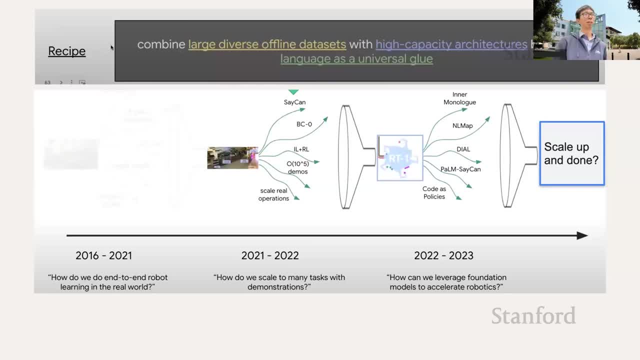 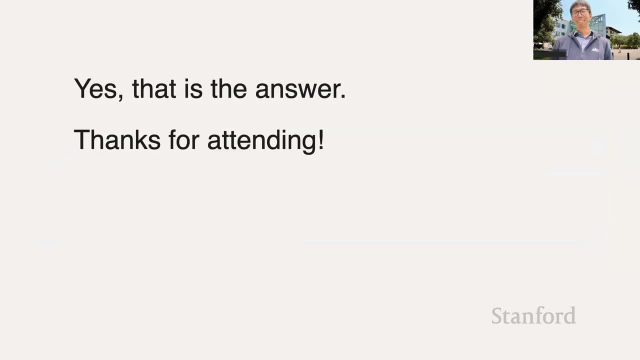 And be done with it And solve robotics And guess what? That's what we did. So that's the end of the lecture. Maybe we can cut this a little bit short. And that's a joke, That's not happening. 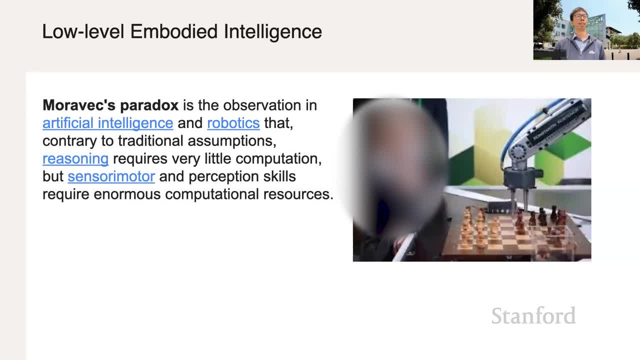 So we are still on our way On our quest to solve low-level embodied intelligence. When I talk to people that you can use foundation models to do robotics, Their reaction would be: It's mostly doing high-level reasoning, It doesn't do the low-level manipulation really well. 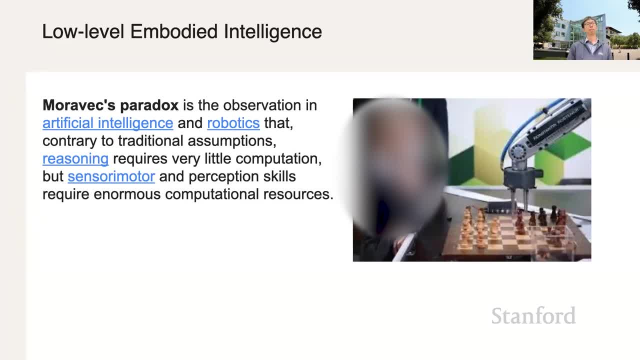 And that's for a reason. One of the reasons is there's a Moravec paradox. Moravec paradox is It's observation that in artificial intelligence and robotics, Contrary to traditional assumptions or our intuitions, Reasoning requires very little computation. 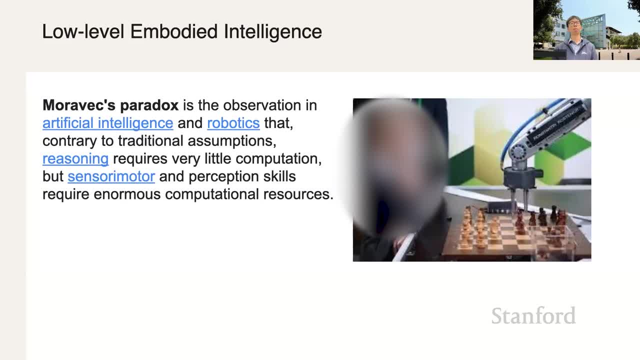 But sensory motor control and perception skills require enormous compute resources. That is because, as biological creatures, We acquire the sensory motor skills through evolution. This is very different, So we might not be able to reason Or do large-scale computation, But this sensory motor control is integral to our survival. 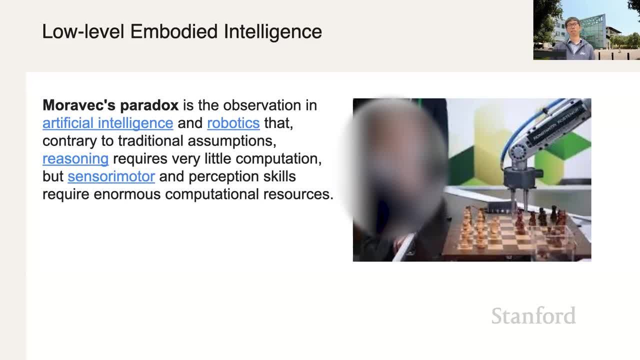 So it's essentially already learning our DNA, But in robotics it's a little bit different. So the chips are very good at doing reasoning and computation, But they are not super good. They haven't experienced the world, They haven't acquired the sensory motor skills. 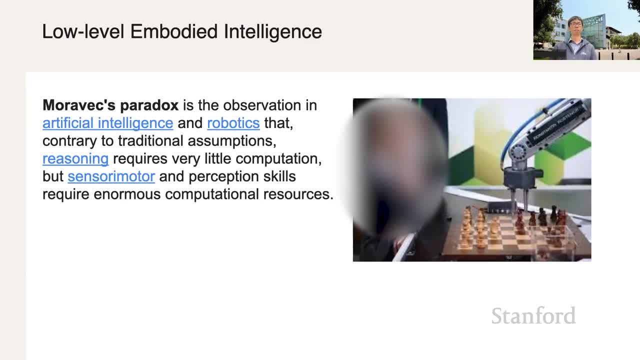 That is necessary for them to do tasks in the real world. Here is an example: When the computer beat Kasparov, Basically the human champion in chess, There is another robot arm moving the chess piece. It can beat the human champion in chess. 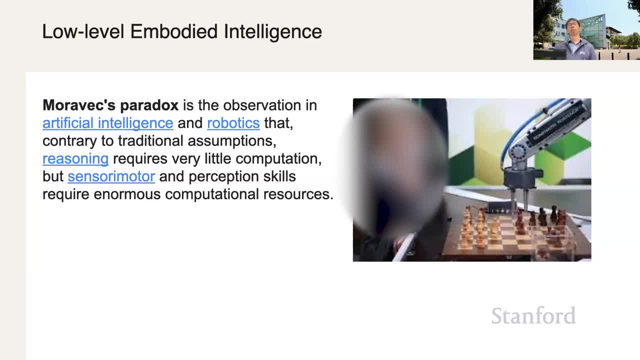 But there is still someone who needs to move the chess piece. Similarly, in the AlphaGo moment, When Lisa Doe was beaten by AlphaGo, There is still someone who is moving the chess piece for them. It's not a robot doing that. 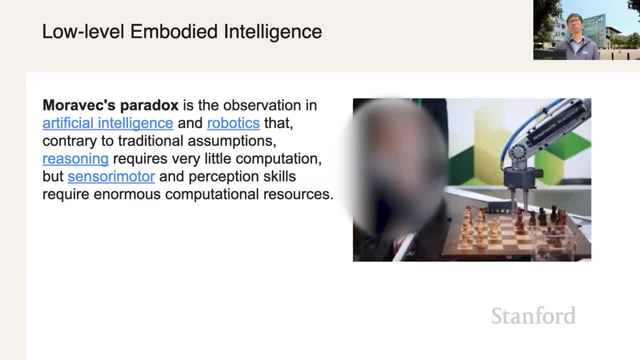 So this is showing the reasoning: The hard things are easy And the easy things are hard. There is another thing that prevents us from using foundation models more prevalently, More in a larger scale, in robotics, Which is the training data bias. 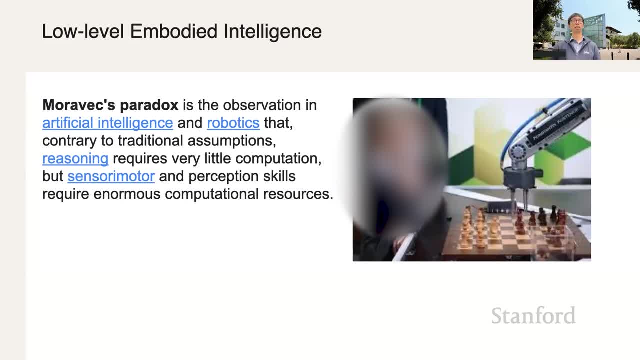 The training data of foundation models or large language models are mostly language tasks, So it's perhaps not that surprising it knows how to clean up a kitchen, Because maybe there are wikiHow articles teaching you how to clean up a kitchen Or to do something in a procedural way. 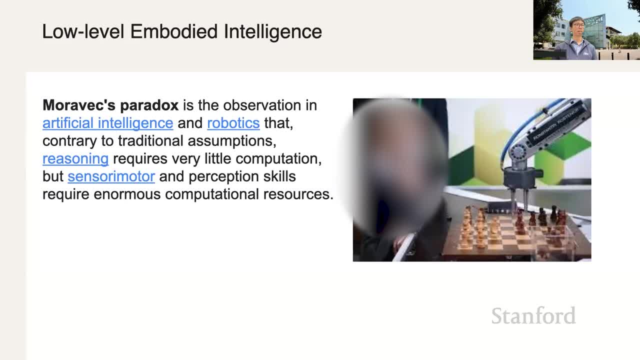 But there are no wikiHow articles teaching you how to move your finger five centimeters to the left, Because people just don't say that. People don't write that down. So there is a very limited amount of this low-level control data in large language. model training corpora. 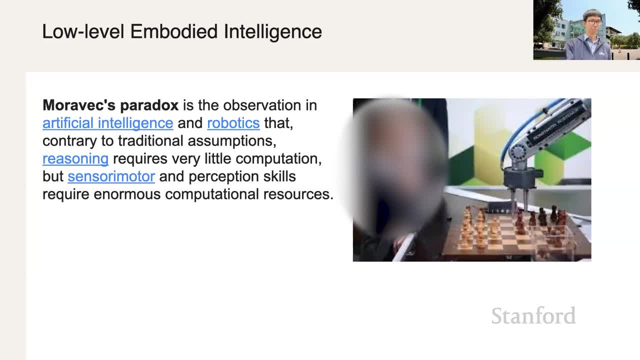 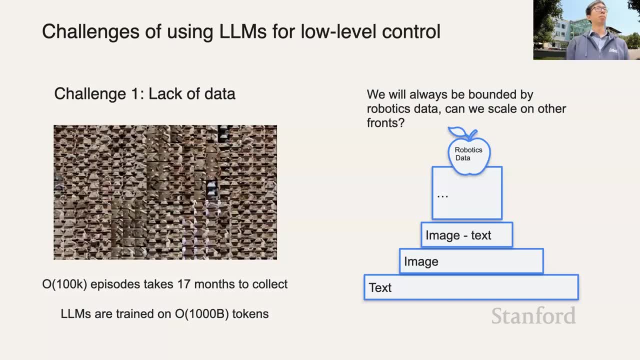 So we do have a lot of challenges in bringing the foundation models to a lower level. So that's what I mean by low-level embodied intelligence. So any questions so far? Also, I want to make this quite interactive, So if there are any questions, feel free to interrupt me anytime. 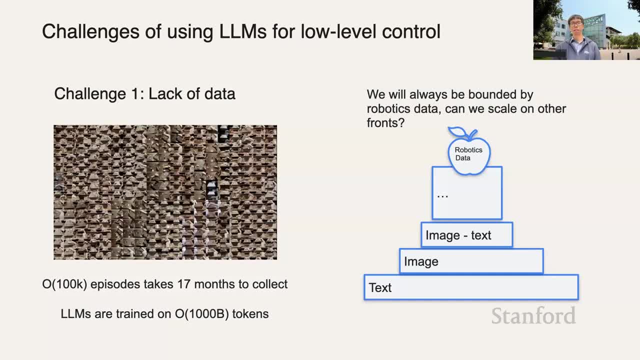 Alright, if not, we can continue. So there are a couple of challenges of using large language models for low-level control, As I just mentioned, the first thing is lack of data, So we only have perhaps 100,000 episodes of human demonstration data. 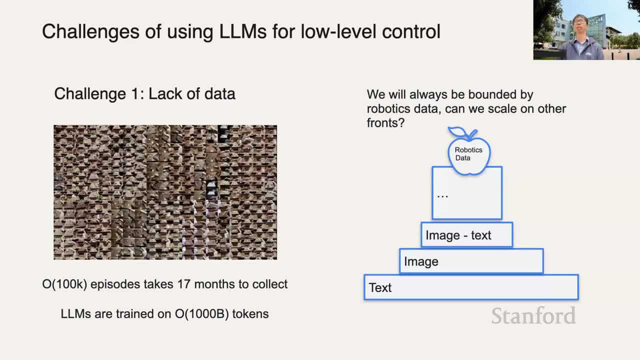 And it takes about 13 robots 17 months To collect. So it's a huge amount of effort. On the contrary, large language models are trained on the order of 1,000 billion tokens. A smaller palm was trained on 780 billion tokens. 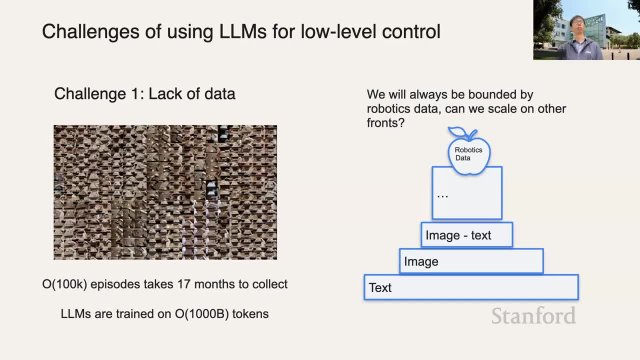 And the larger one is trained Following the chinchilla rule, you would need to train it on 1.35 trillion tokens. So it's a huge amount of discrepancy Between how much data we can use, Between how much data we can achieve in robotics. 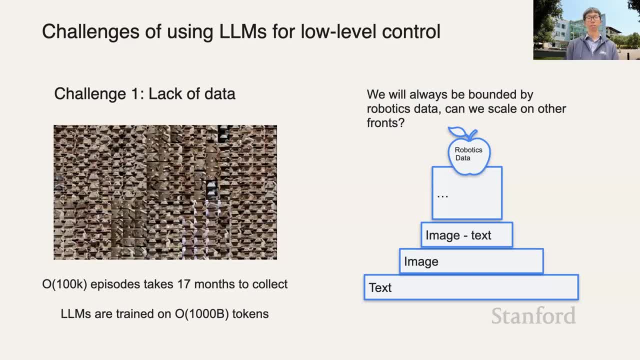 And how much we can get in large language models. So we will always be bounded by robotic data. So maybe we can scale on other fronts. Maybe we can keep the robotics data the same And then we can scale on other fronts. 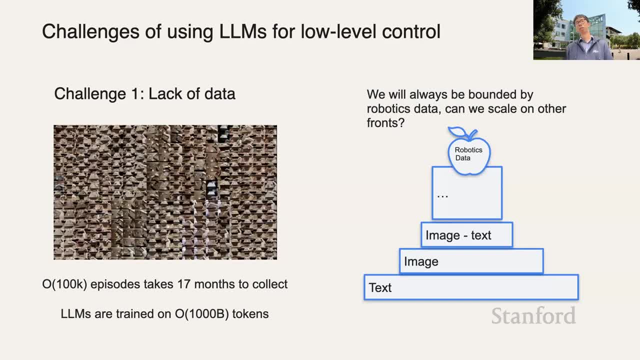 Like, maybe we can scale the pre-training mix of text and image, Or maybe image and text pairs. Maybe we can build this cake- And the robotics data is just a cherry on top of it- And we can scale the fundamentals And we can scale the foundation really, really well. 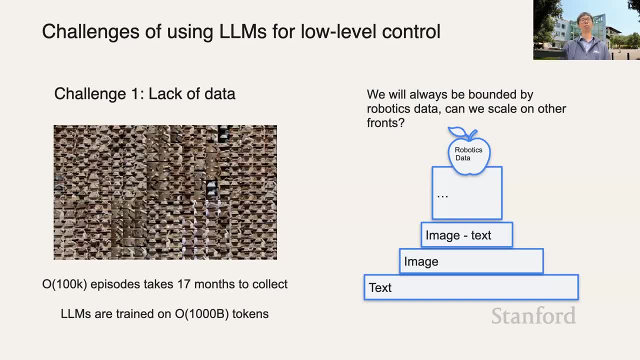 Some of my work that I'm going to talk about today actually reuse the RT1 data. We don't collect the new data for RT2.. But we want to do more things with the same amount of data. The second challenge is kind of related to the first challenge. 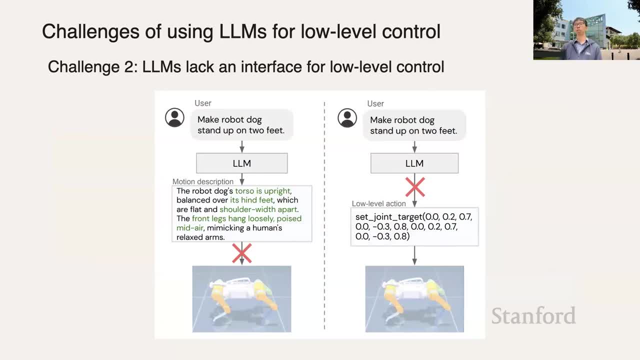 Language models lack an interface for low-level control. If you ask a language model, how do you make a robot dog stand up on two feet? There are a lot of things that sounds reasonable, Sounds plausible. It will tell you the robot dog's torso is upright. 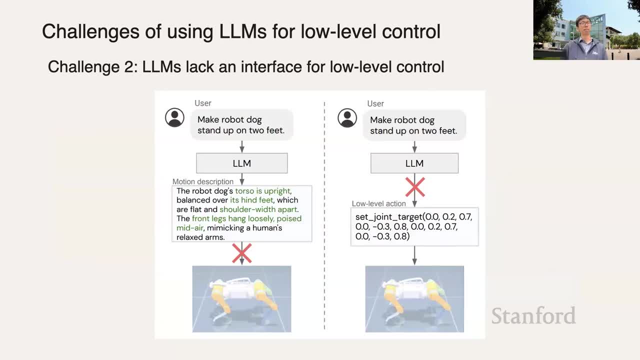 Balanced over to hind feet And standing shoulder width apart. This is great. This is all great, But we cannot put it on the robot. On the other hand, maybe we can ask the language model to write control code to directly control the robot. 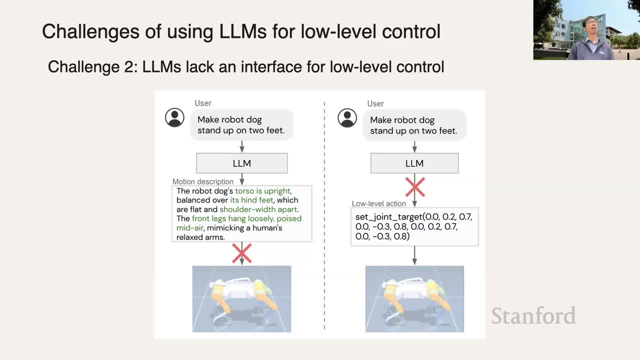 But usually that requires you to curate an API that is friendly to the language model. It will directly ask it to give you my joined answer. It will not give you the right thing because it doesn't have enough context. So, essentially, large language models don't speak robot language. 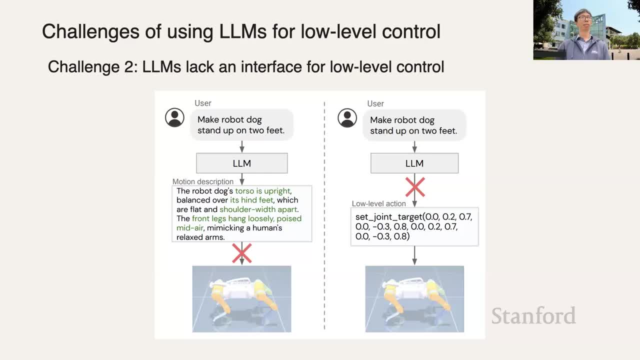 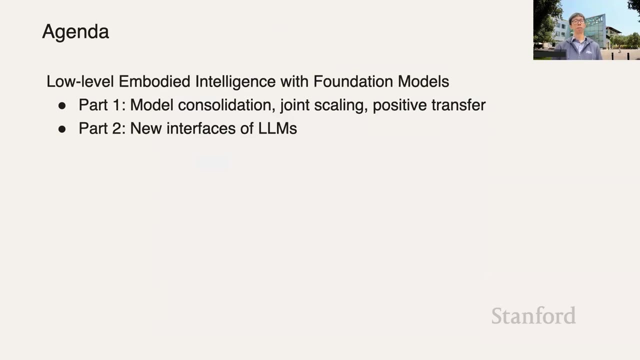 Can we actually find the right robot language? Can we find an interface between large language models and robot control, Or can we just treat robot action as another language? So that's what we want to find out. So in today's agenda I will be talking about low-level embodied intelligence with foundation models. 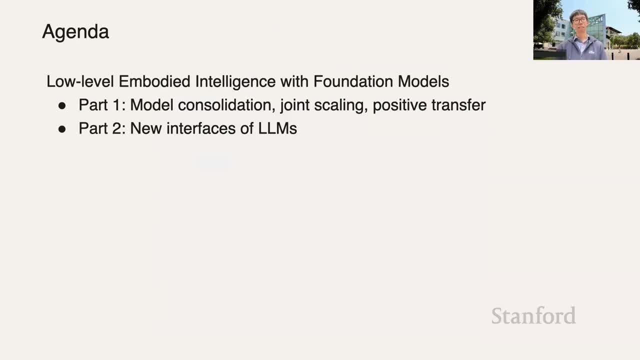 It's separated into two parts And it's addressing the two challenges that I've just mentioned. Part one is about model consolidation, joint scaling and positive transfer, So I have to put them in one part because they are somewhat related. And part two is developing new interface of large language models. 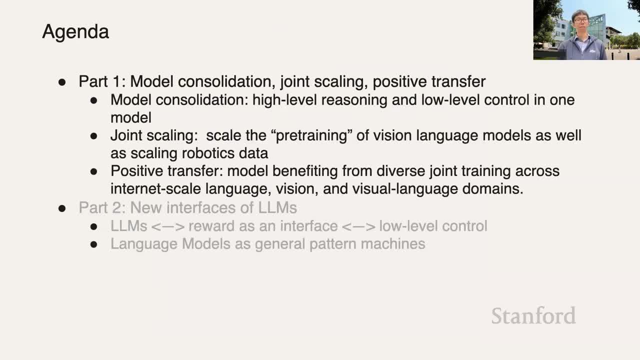 So what do I mean by model consolidation? Model consolidation- Yes, question. Yeah, I was going to ask why couldn't you do your ideas by Tune and LLM, Or Yeah, that's a great question. So the question is: why cannot we fine-tune language model to directly output low-level code or robot actions? 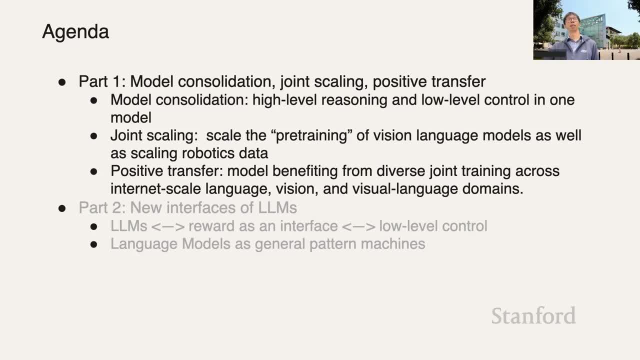 So I will be talking about RT2, which does somewhat similar to that. It fine-tune language model to output action as a language, To output our action representation. There are certain downsides to that, Like, for example, you would need to collect additional data to fine-tune a language model. 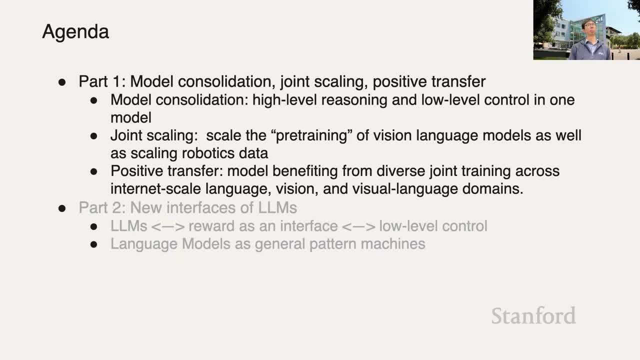 So either we can fine-tune that or we can use the language model zero-shot if you find the right interface, Which I will talk about a little bit in part two: Zero-shot and without fine-tuning. Without fine-tuning- Yeah. 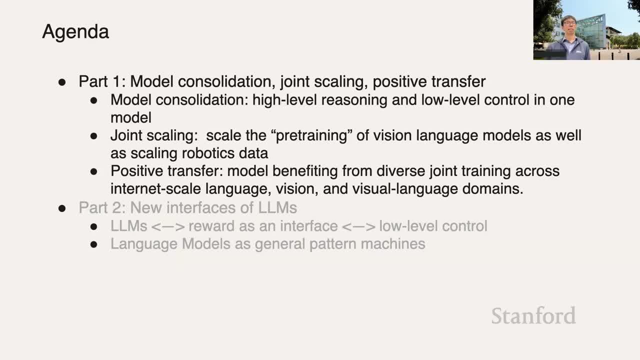 So the model consolidation is: essentially we can do the high-level reasoning and low-level control in one model And joint scaling is: Not only do we scale the robot data, which is expensive, we also scale the pre-training data Or we already start from a pre-trained vision language model. 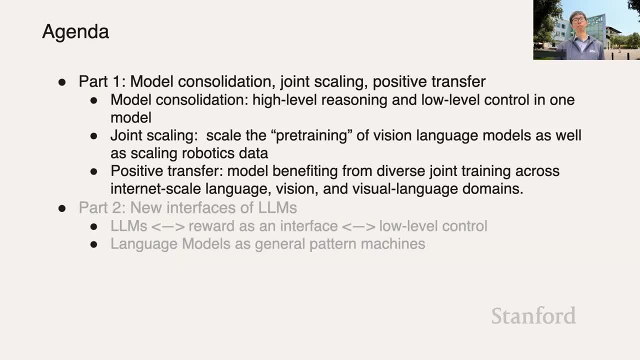 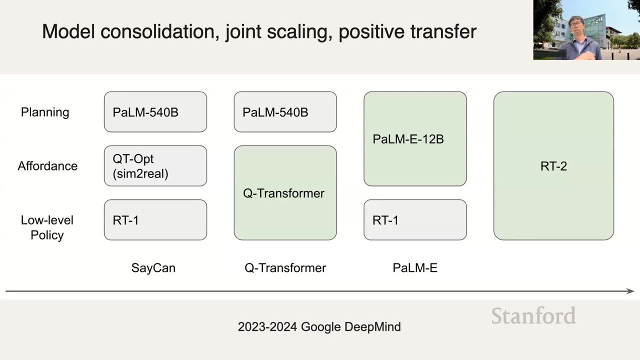 And a positive transfer is the model benefiting from diverse joint training across Internet-scale language, vision and vision language domains Combined with robotics. So this is a continuation of the axes that TAD drew in 2018. In his previous talk. So we can see there is a trend. 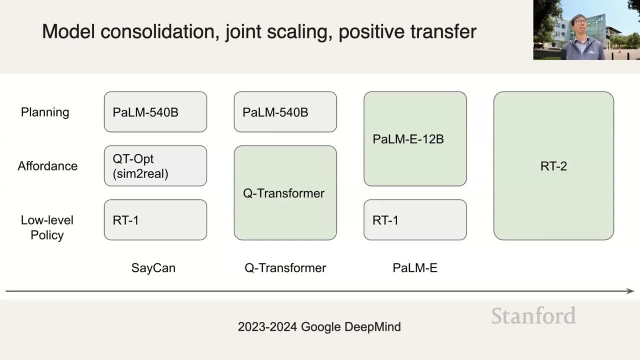 So this visualization basically highlights some of the work on our team, And each work, each column, is basically a robotic system that is able to do both high-level reasoning and low-level control. So previously we need to have separate models for each thing. 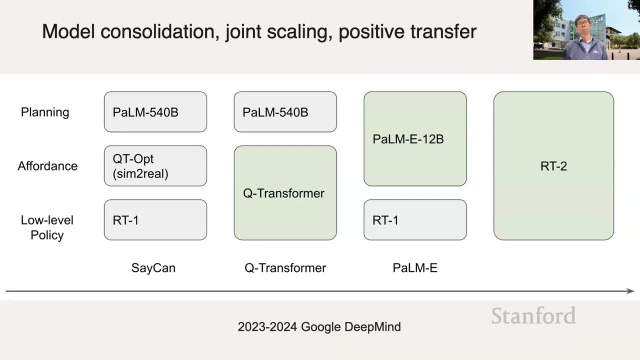 Previously in the initial release of SACAN. the planning is done by a large team. It's a large language model And the affordance is done by. The affordance is done by a QT opt-in policy trained with Sim2Real. 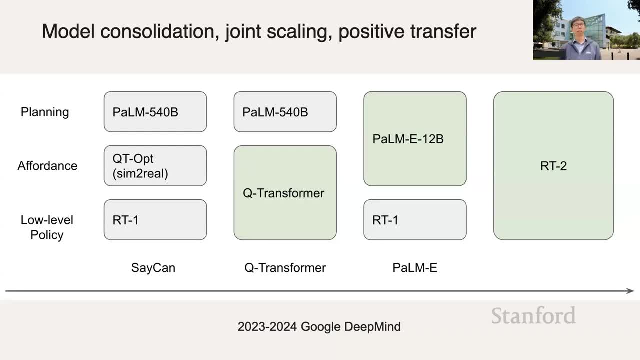 And the low-level policy is Robotic Transformer 1. So it's each model doing its dedicated thing And you need to train each model differently And perhaps with different type of data, And later we have QTransformer, which unifies. 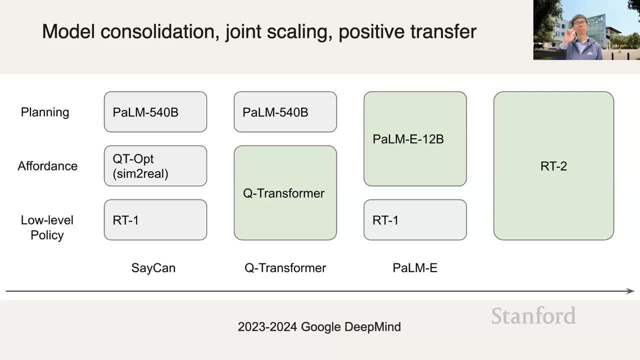 Which is kind of an offline RL method that is leveraging transformer architecture. So it's a high-capacity architecture. It can train on both positive data and negative data And with that we are able to get a policy that is also understanding affordances. 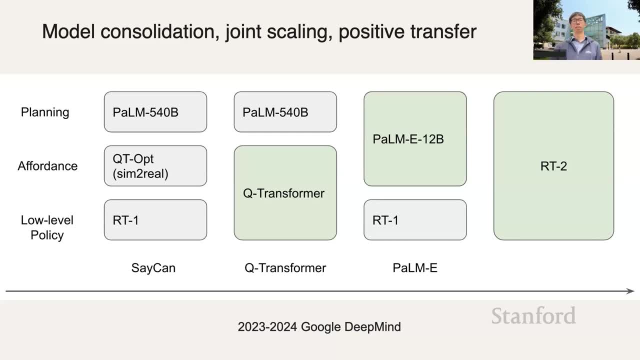 So we can unify the low-level policy and affordances, But the planning is still a large language model. And then we have Palmy, which is a vision language model, Which is a large language model, Also trained on a vision language domain. 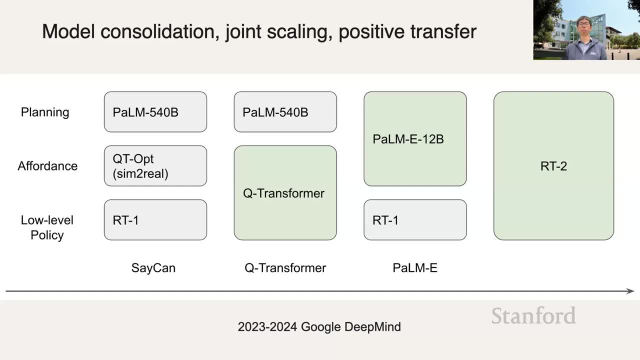 So the Palmy can do planning and affordance in just one model, But the low-level is still using RT1.. And finally, we unify everything together, Like there is RT2, which I'm going to talk about today- That can do both high-level planning- to some extent generating affordance- and do low-level policies. 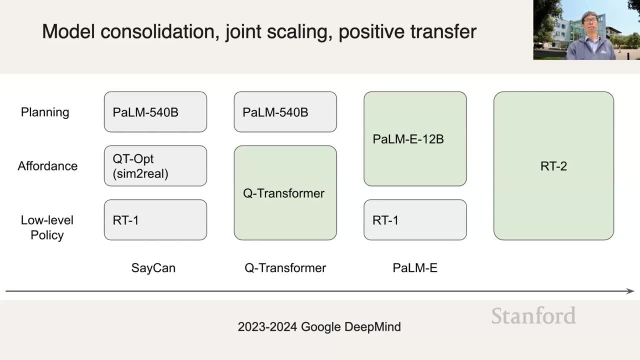 So behind the model consolidation is the consolidation of tasks. We can represent every task as a vision plus text, So it's a really universal representation of the task And then with that you can train it really on using a lot of data And you can see positive transfer. 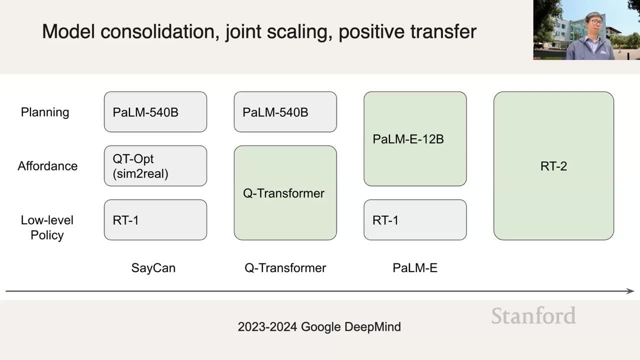 Basically learning affordance can also tell you how to achieve a task, Like there are transfer between tasks when you pull all the tasks together. So to understand this joint scaling And to understand the model consolidation, We need to understand Palmy a little bit. 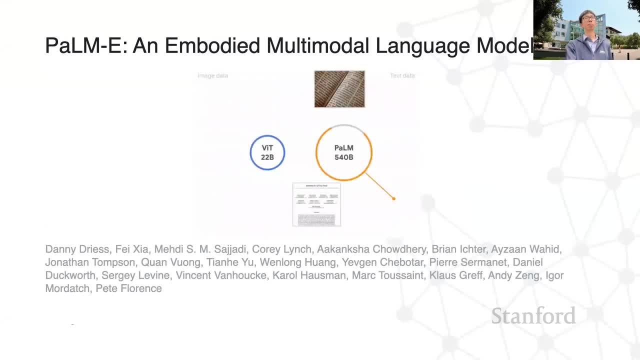 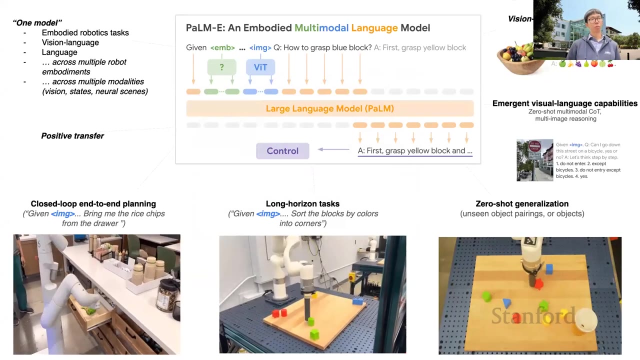 So Palmy is an embodied multi-modal language model. It's based on the Palm architecture, So Palm is a large language model. We made some adaptation on the architecture So it can understand multi-modal input. So it is basically one model that is able to take in multi-modal input. 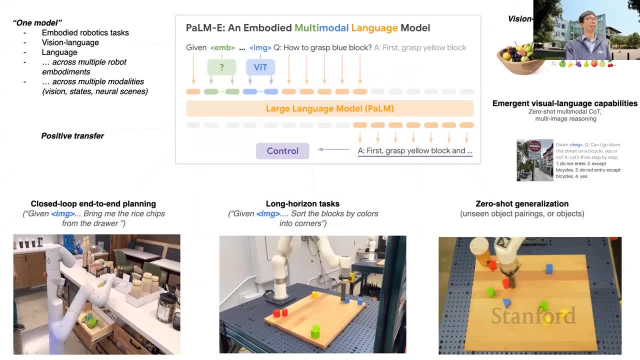 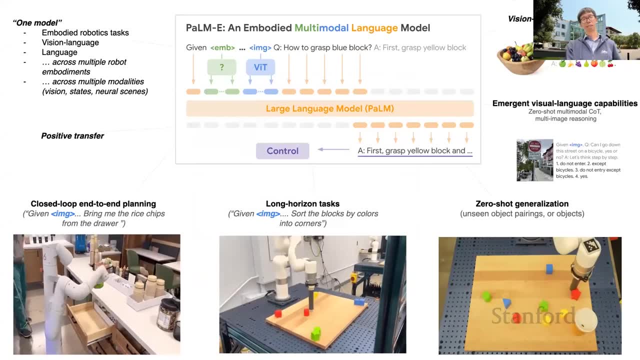 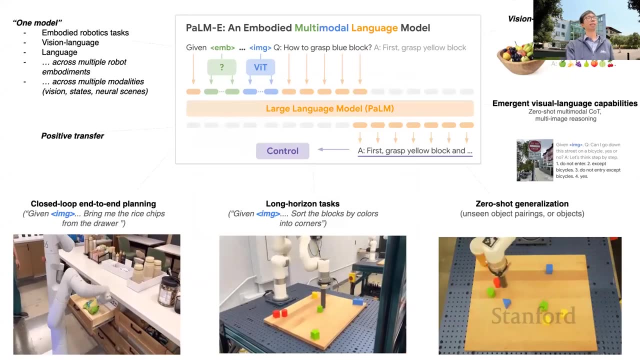 So it is basically one model that is able to take in multi-modal input. So in large language models each word is tokenized And tokenized and getting this embedding of these words, And then that is fed into a large language model. So in Palmy what we do is, instead of using words we can use multi-modal tokens. 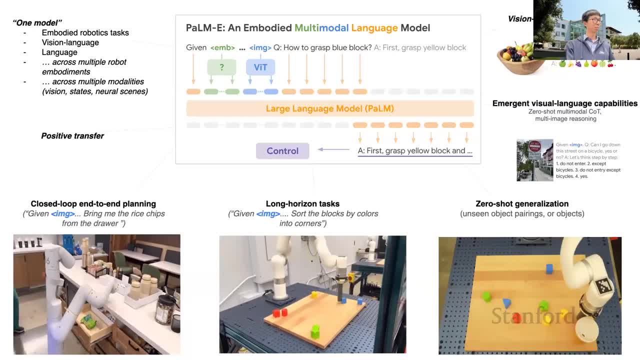 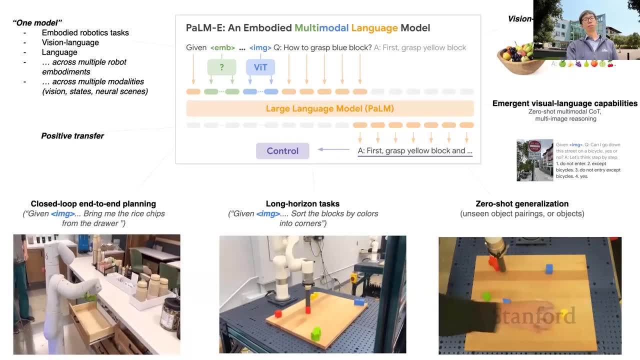 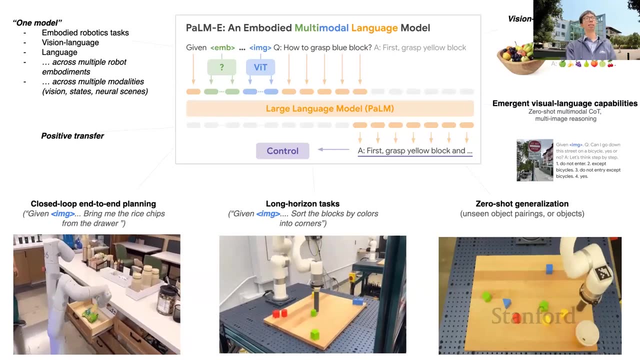 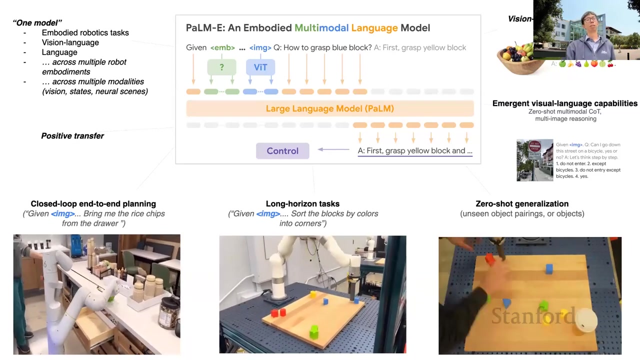 So the multi-modal tokens can come from a vision transformer, a VIT, Or it can come from robot sensors, Or it can come from robot sensory data. So every multi-modal token then we map it to the text embedding space. We basically train a linear affine transform between the multi-modal token and the text embedding space. 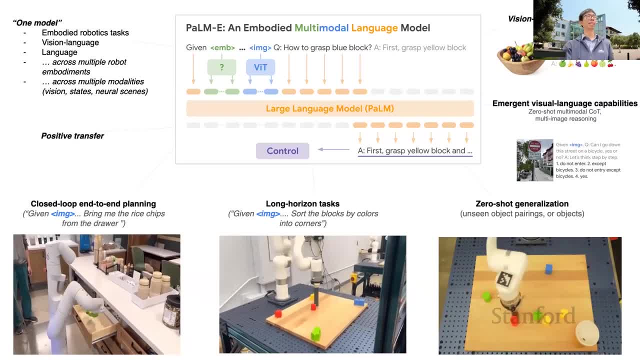 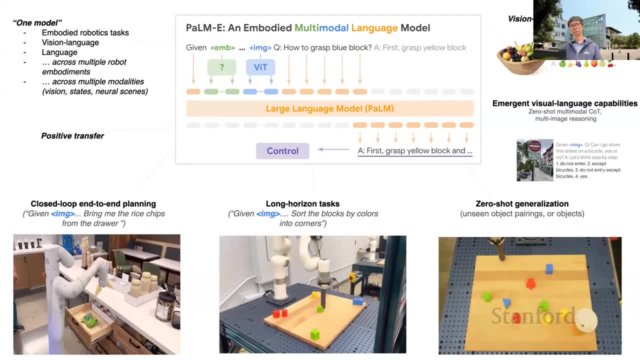 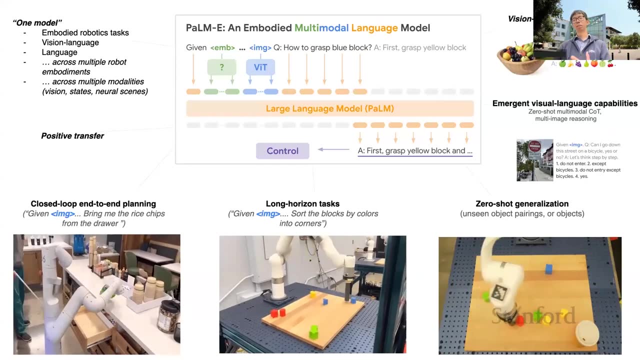 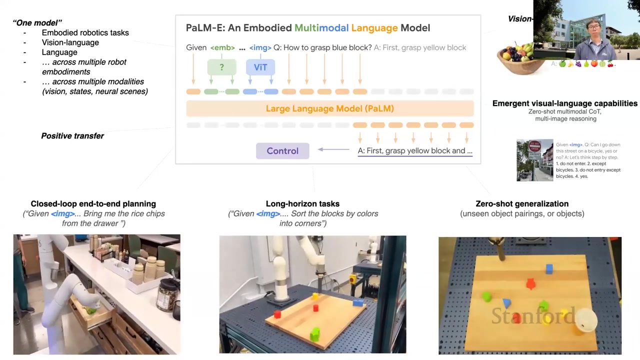 And then we can treat the multi-modal token as words as well. So essentially, we have a language model as words. We can treat the language model as a solid base And then we start to adapt it to understand multi-modal tokens. So this is quite interesting because it doesn't require a ton of adaptation or fine-tuning for it to understand multi-modal input. 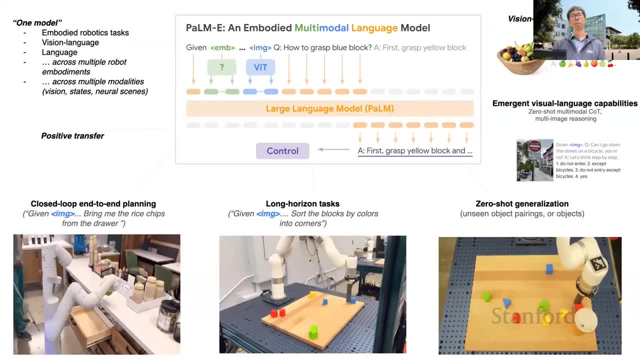 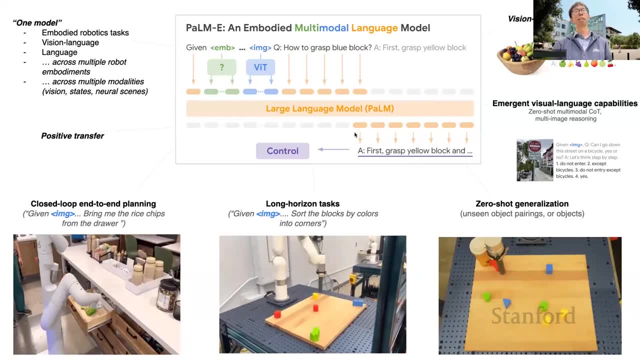 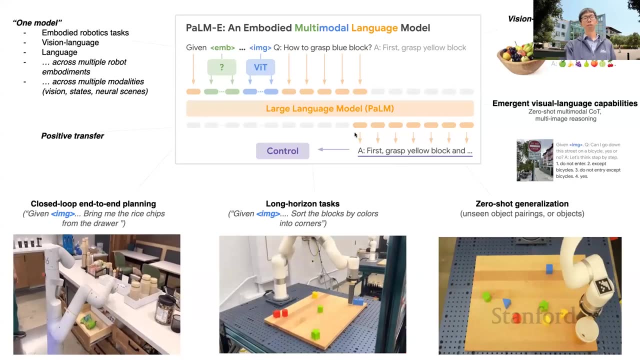 It just aligns naturally to the multi-modal input, such as images. I will show a couple of examples of what it can do And we can train it the same way as training large language models. We can reuse the same infrastructure and training algorithm and everything to train this POM-E. 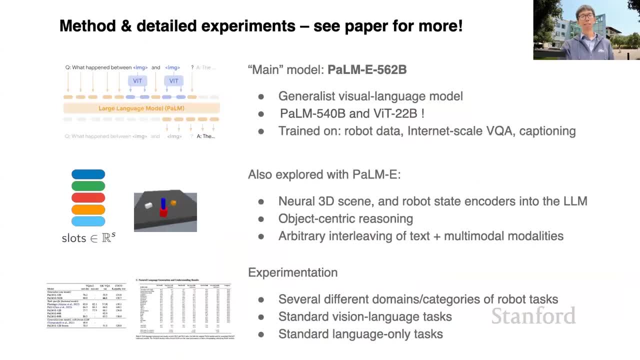 A couple of other things we find along the way is positive transfer, which I will share in a little bit. So I guess here I also want to mention POM-E is one of the largest models we have explored so far. It has 562 billion parameters, which is, by concatenating the POM, 540 billion parameters. 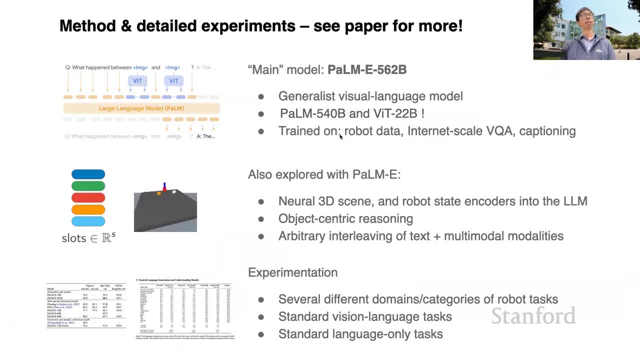 and the 22 billion VIT, And we find a lot of emergent capabilities of these models that we haven't expected during training time. But really we can prompt these models and ask them to do interesting things. We have also explored using neural scene representation. 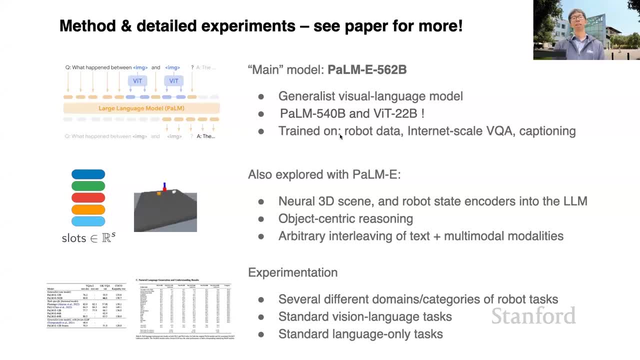 basically an object-centric representation and fed into POM-E. So object-centric representation assigns one token to each object And we find that this representation is super helpful for robot planning tasks, because traditional VIT representation is based on grid and it doesn't have a full understanding of like objects and their relationships. 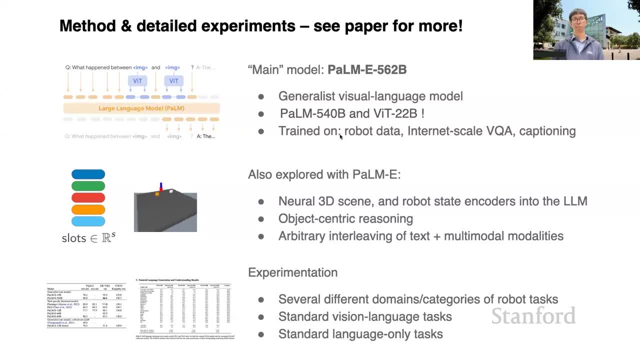 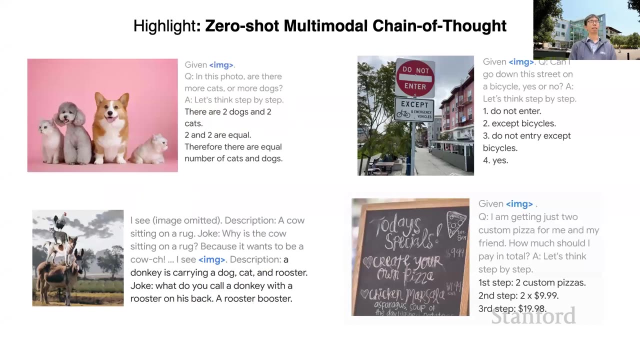 We have done an extensive study on the scaling performance and the catastrophic forgetting performance and all other interesting experiments in the paper. So please refer to the paper for more. So here I'm just showing some interesting qualitative examples or some emergent capability of POM-E that we found out. 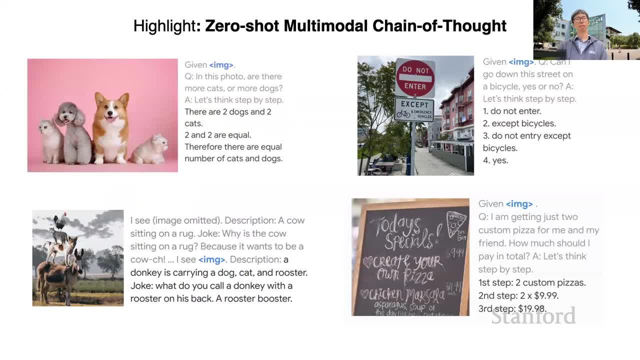 So first, we found this model has some reasoning capability. You can give it an image and ask it questions. that requires a little bit of reasoning And you can prompt this with- let's think step by step- which is a technique used to elicit reasoning. 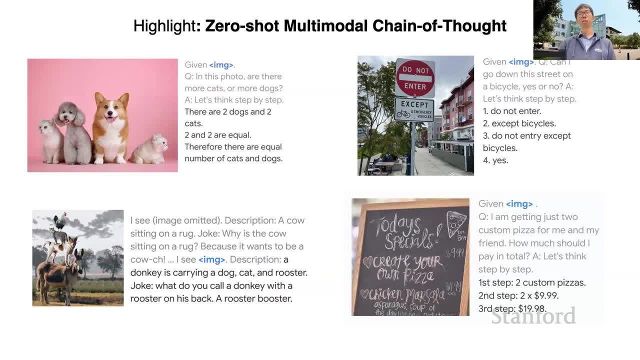 in large language models, But here in multimodal language models you can do the same. I guess people are also experimenting it these days with GPT-4V. You can also prompt it to think step by step or count row by row. 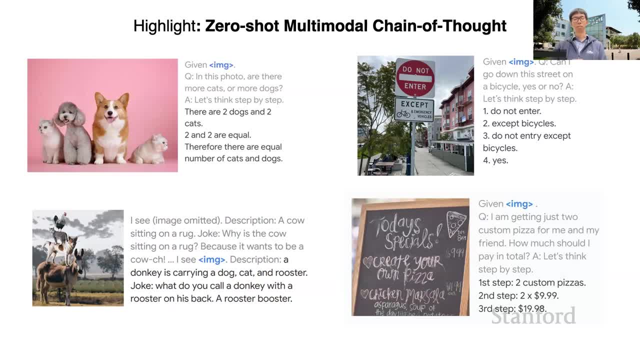 But here this is before GPT-4V, and we were able to elicit reasoning using some of the interesting prompts, such as we can ask it: in this photo: are there more cats or more dogs? Let's think step by step. 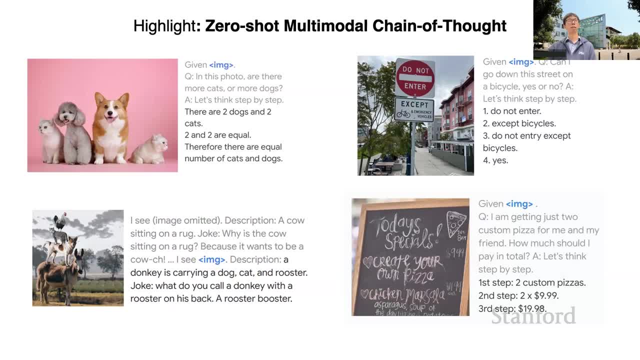 And they found that the POM-E found out there are equal amount of dogs and cats, And on the right give an image. Can I go down the street on a bicycle, Yes or no? Let's think step by step And the reply is: do not enter. 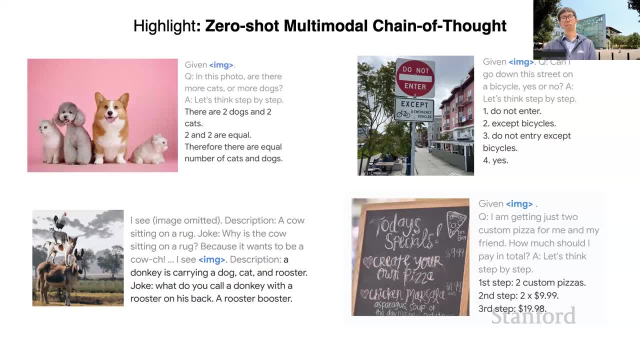 Second, accept the bicycles. Do not entry except the bicycles. Yes, So it's doing this model of reasoning and it's mixing this understanding of symbols and also mixing the understanding of text. So this is quite amazing to me, To be honest, when I first saw this. 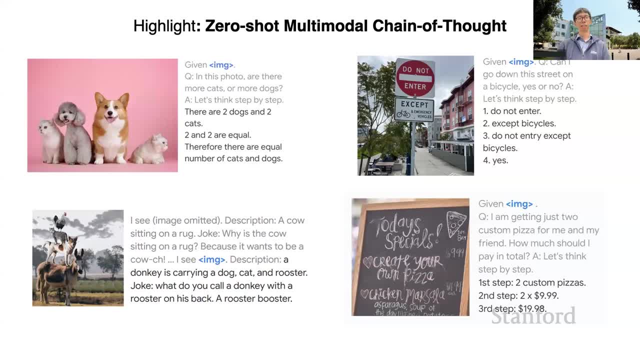 I didn't expect a multi-language model would be able to do that, And we also tried one thing which is traditionally very difficult to language models, which is to tell a joke. Language models can understand joke, but sometimes it's not able to tell you a joke. 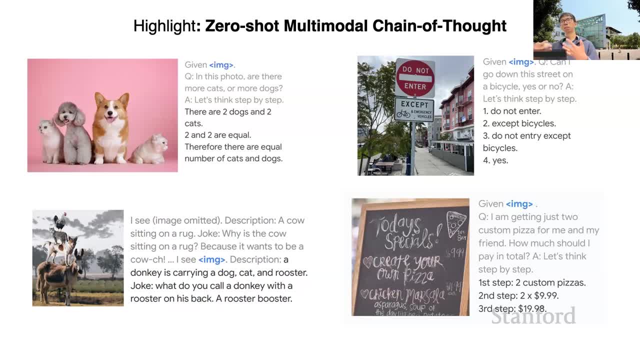 when it comes to the punchline, because it's just trying to make something that is plausible and sounds like a joke. And when it comes to the punchline, it doesn't really know what to say. So here I give it an image and I ask it to come up with a description. 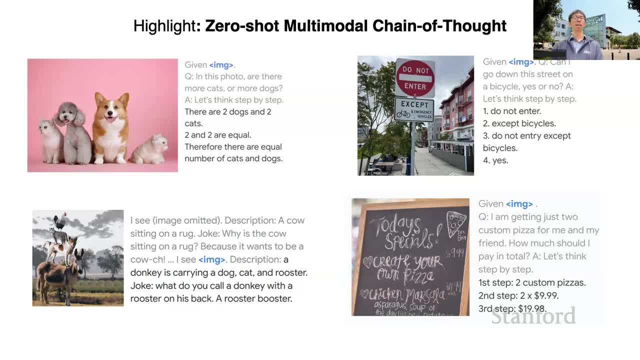 and then comes up with a joke. So this guides the language model to think step by step. And the description is: a donkey is carrying a dog, cat and rooster And the joke is: what do you call a donkey with a rooster on his back? 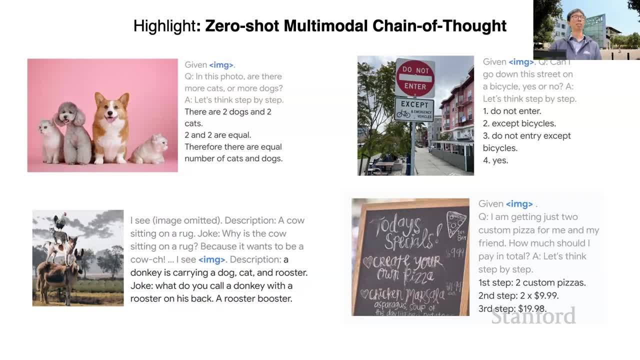 A rooster booster. It's so creative Like. when I saw this, I'm pleasantly surprised And I searched online. I couldn't find another joke like this, So it's actually an original joke by Paul Mee. And finally we see some math reasoning with this model. 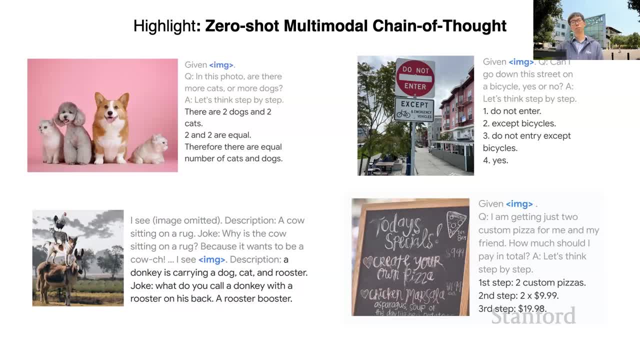 Basically, I give it a messy manual from the pizza store and I ask it: I'm just buying a pizza for me and my friend. How much should I pay? Let's think step by step And it's figuring out. there is a pizza. 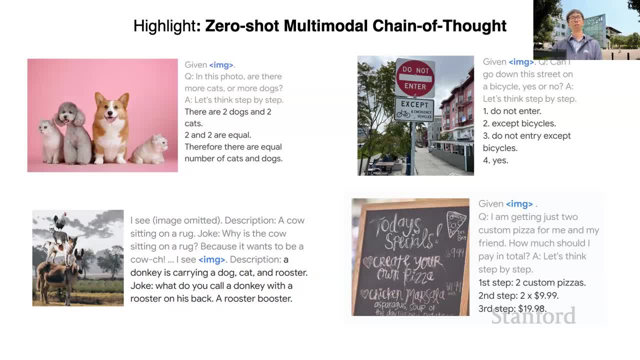 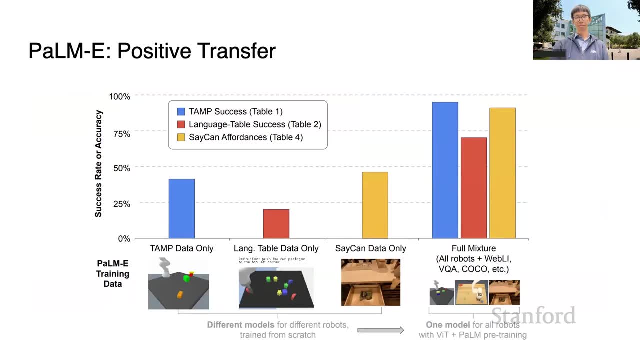 and there is a $9.99 and it tells you the price. In some of the answers it even calculates text, But the text is hallucinated, So that doesn't work. All right, Let's talk about positive transfer. So, apart from the amazing capabilities, 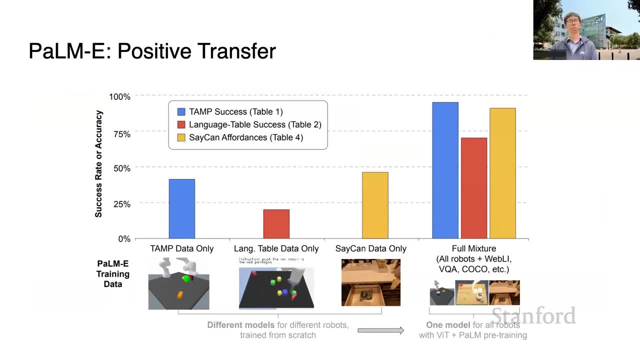 amazing things that Paul Mee can do. it also has interesting positive transfer behavior. So when we train Paul Mee on a single domain, when we train it on just a single robotics task, the performance is not super great. But when we pull all the data together, 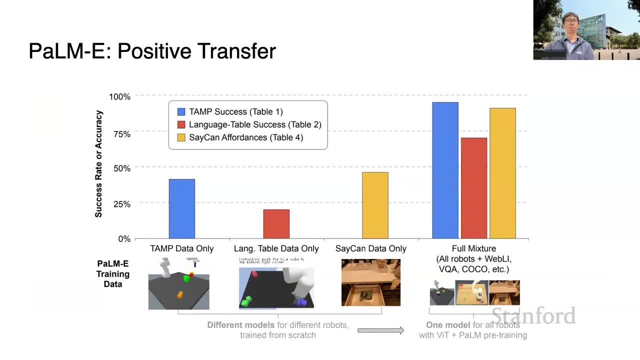 and we also include internet scale vision language tasks such as captioning or visual question answering, it is able to do much better, So this shows that it's important to mix all the data together and train it jointly. The internet scale data can act as a regularizer. 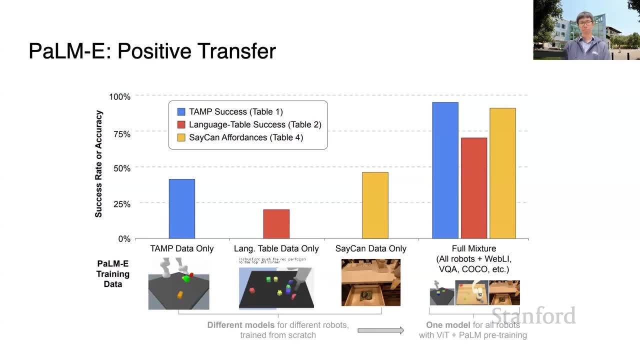 for you to not forget the representations, And those representations are, in turn, very useful for robotics. So that's the positive transfer results, And we start to see more and more positive transfer in other of our studies. Yes, So how much data do you collect? 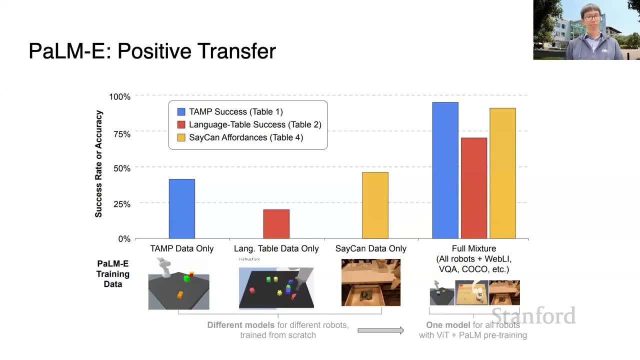 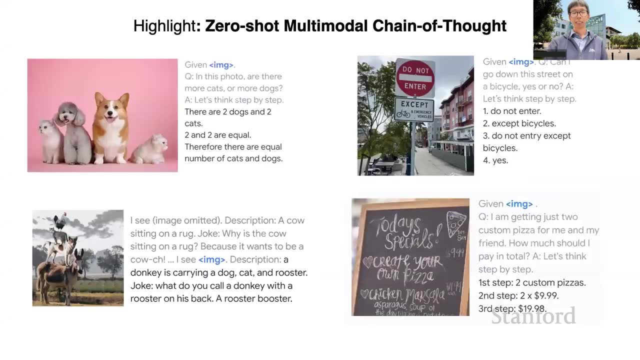 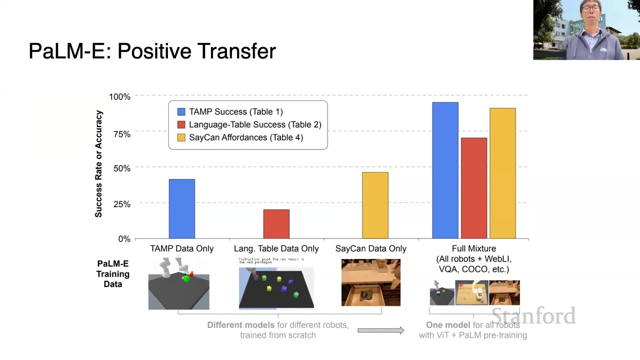 Like in simulation or in real world. I think the playing with sorting stuff on the table is very impressive. Right, Yeah, that's a very good point. So these are all planning data like high-level planning. So maybe let's just talk about two things. 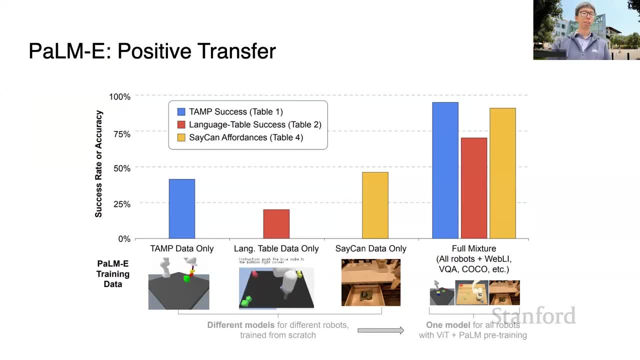 So, first of all, the sorting results. the low-level policy is still using a traditional controller, So it's using a policy called LAVA, And that policy is trained on 68,000 episodes. The high-level planning is probably easier than you think, because it only needs to tell. 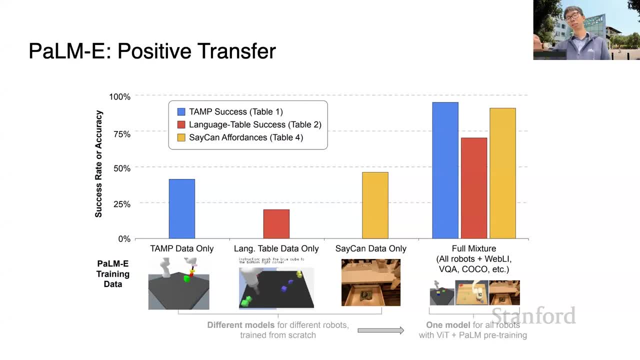 sort put the giving command to the low-level policy. So it's basically only need to say: put the red block into top left corner, put another red block into top left corner. So it's rather a quite standard autoregressive. 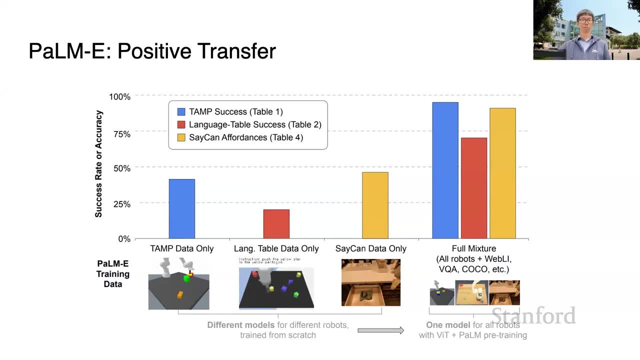 autoregressive, like language modeling task. The only thing I need to do is to determine what task is not finished yet. So, for example, if the block is already in the corner, it shouldn't call low-level policy to move it to the corner again. 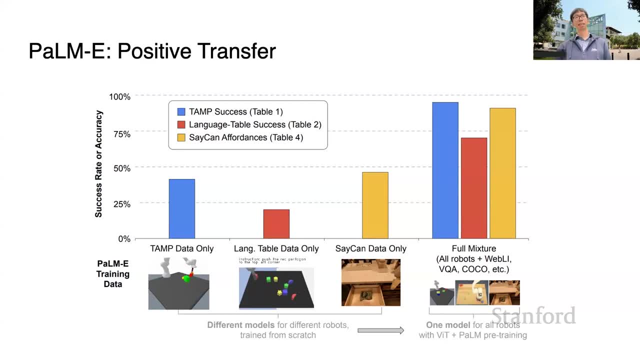 So it's rather like understand, parsing the states And understanding the states. So this high-level policy only requires about like 50 to 100 demonstrations to learn, So it's quite parameter efficient And in the future that's a very good question actually. 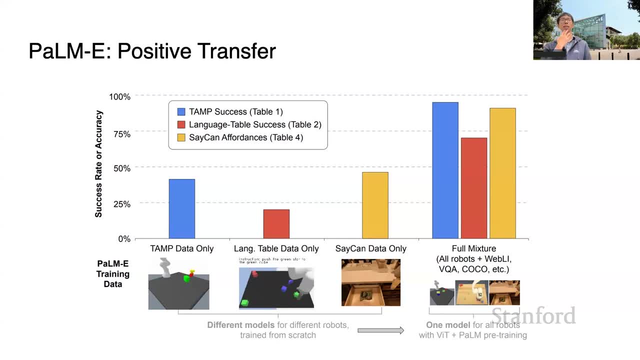 In the future. a lot of these tasks can be taught in context, So maybe we just demonstrate it once to the large language model, then it knows how to do that. How can the large language model know like which low-level This is? through human demonstration as well? 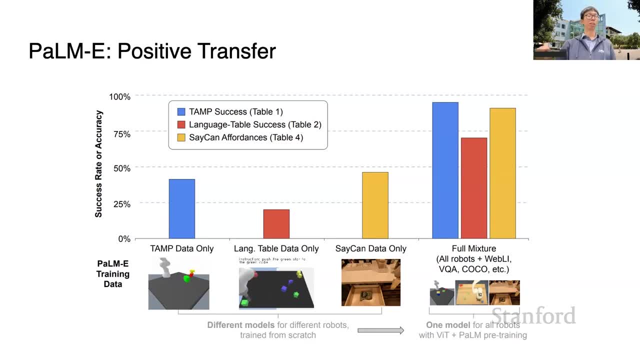 So human on a low level can demonstrate low-level policy by tele-operating a robot to do a certain task. But on a high level it could also just give the low-level policy Like: imagine your control interface is through text And then you can. 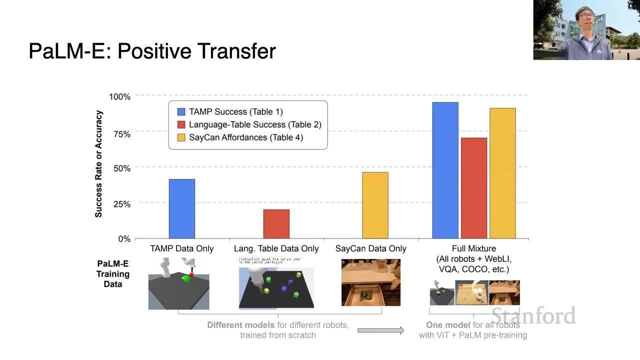 as a human, you can also guide a low-level policy to accomplish a task, And then that thing can then be used to train a large language model. So that's for the sorting block. The second is a little bit more interesting because the planning steps. 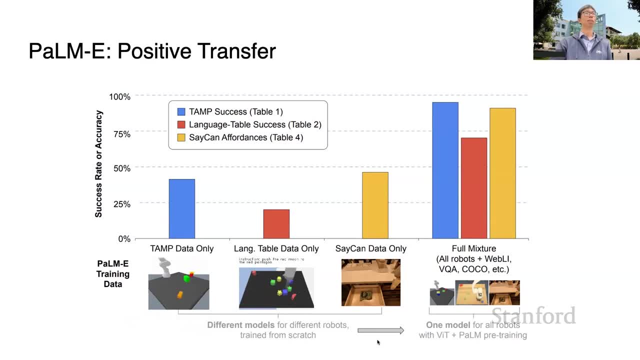 are actually generated by Palm. So we essentially distilled Palm plus this affordance model into Palm E. So that's a little bit more interesting. That's like using the AI data to bootstrap itself. That one has about 3,000 episodes- also not quite a lot. 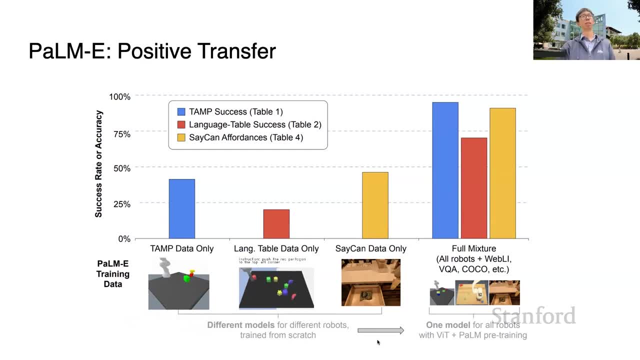 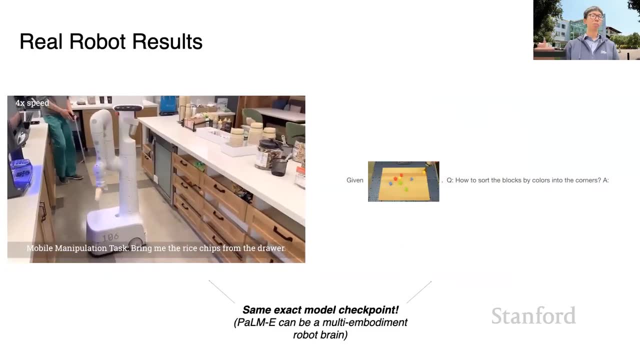 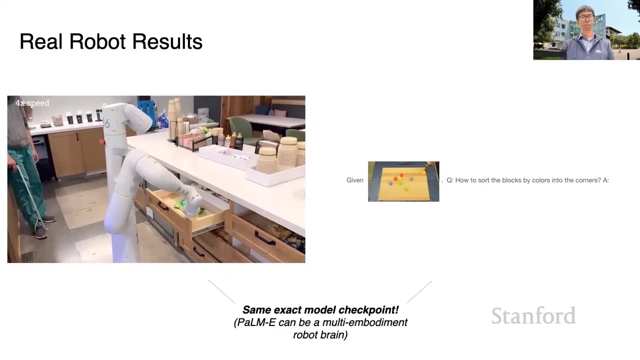 But it's able to learn complex planning behavior, re-planning behavior, error recovery, which I will show in this slide. So with the Palm E as a high-level planner, we are able to take the rice chips out of the drawer. And there is a twist. 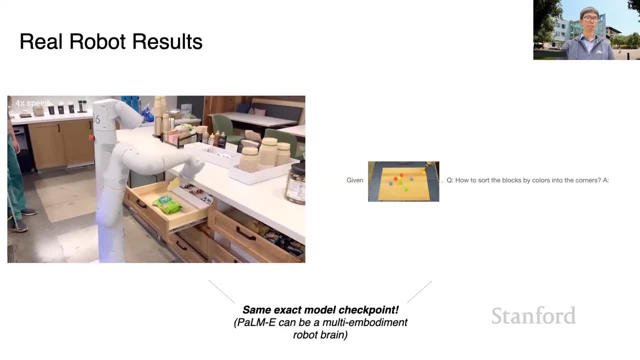 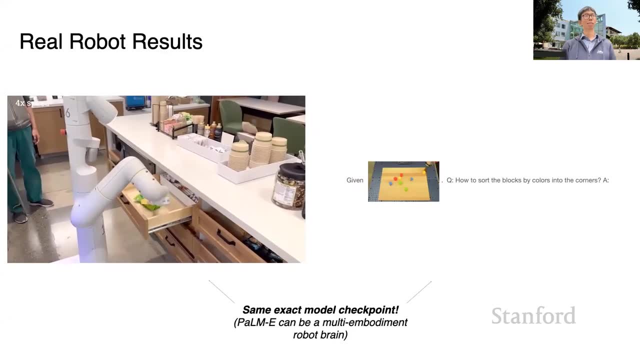 which is I will be messing with the robot. So, as it put onto the counter, I put it back to the drawer, And then, as it pick it up again, and then I put it back again, So it's able to understand the state. 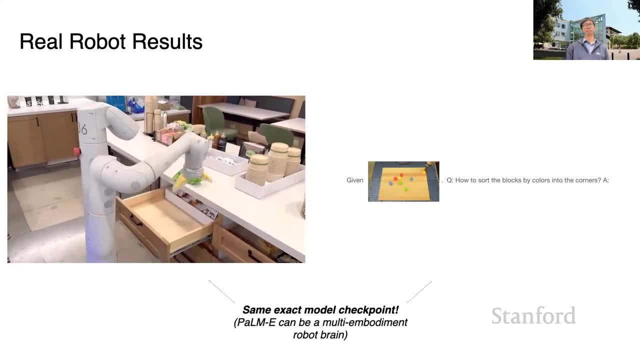 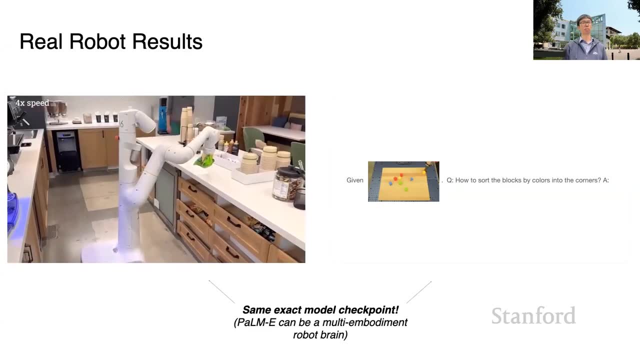 It's able to understand my task is not finished. I cannot proceed with the next task Now, after I don't mess with it anymore. it's able to close the drawer and pick up the bag of chips, So Palm E is able to combine affordance. 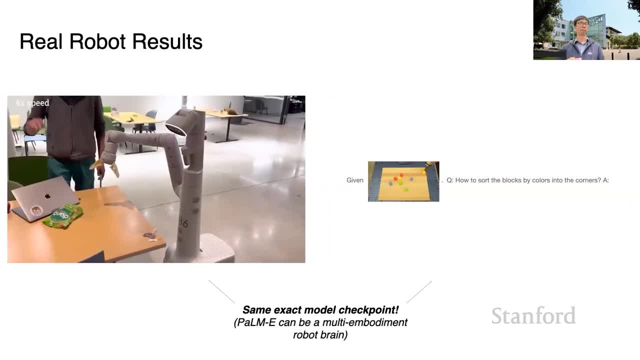 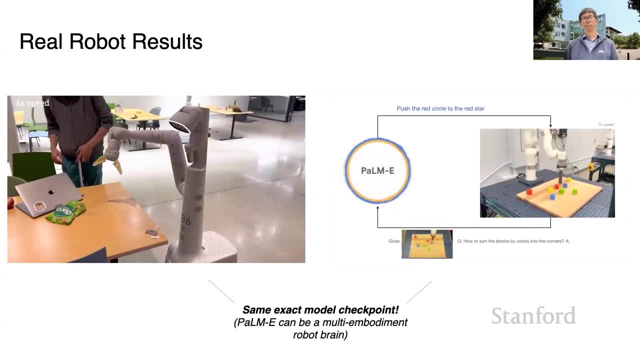 and planning in one model and do complex reasoning of the scene and environment. And interestingly, we can use the exact same model checkpoint to do block sorting as well. So this is the same model checkpoint. It can not only reason about how to bring a bag of chips to a user. 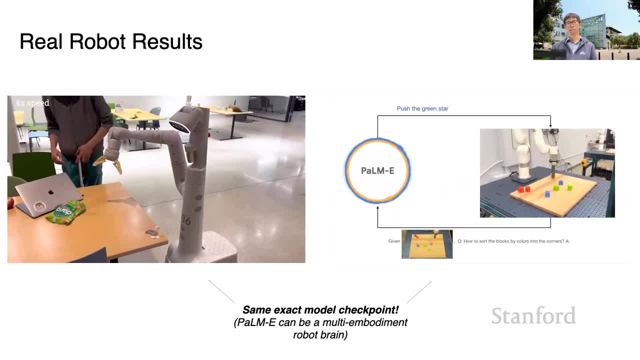 it can also sort blocks And it's also responding to adversarial perturbation, Like if the user is putting the block in the middle again, it's able to recover from that. So these are all coming from the same model And it can also tell a joke. 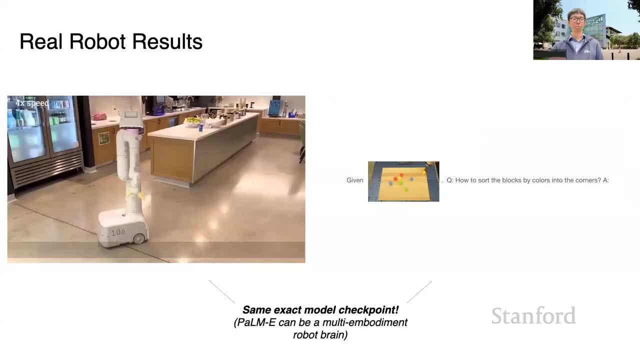 So, yeah, this is the power of like vision language models. Now we want to go a level deeper. Like these are all vision language models that are used for planning or high-level reasoning. Can we use them for low-level control? It turns out we can. 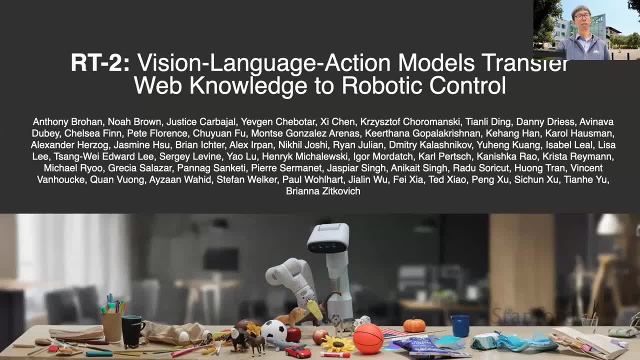 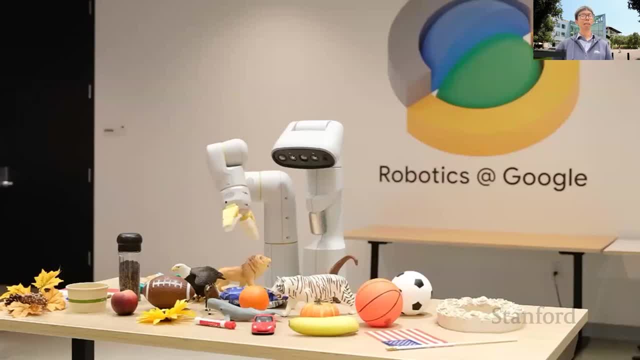 And that's the RG2 work, which is vision language action model to transfer web knowledge to robotic control. What can it do When asked: pick up the extinct animal And it has a whole range of objects on the table. It will pick up the dinosaur. 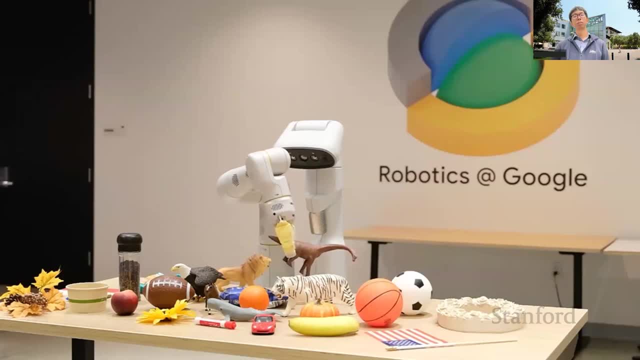 So it can link the extinct animal to dinosaur and to the action that pick the dinosaur up. So it's really doing like this emergent reasoning and also the manipulation in just the one model. And, by the way, this robot hasn't seen any of these before. 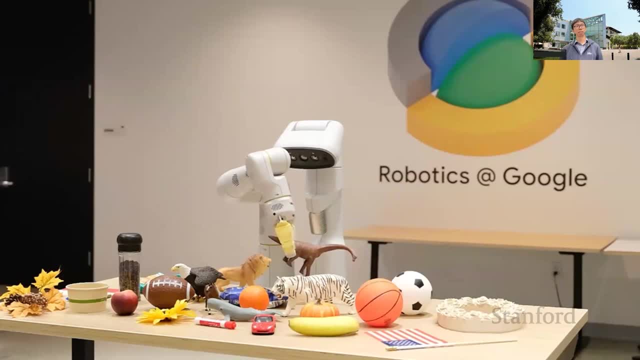 at least in the robot training data. It might have seen this in the internet catalog, right, But it has never seen it in the robotics training data. So it's quite interesting how we need to evaluate these robots nowadays. So when we evaluate language models, 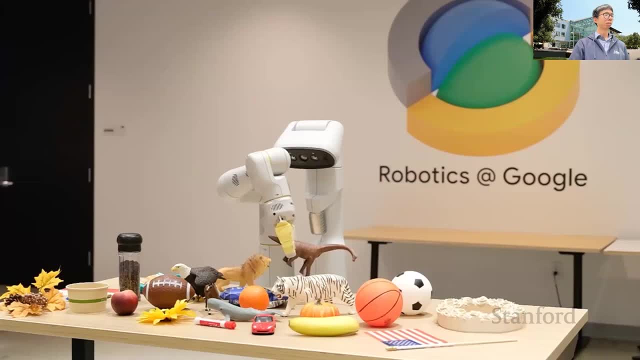 to prevent data contamination. every time you need to give it new questions, otherwise it might already memorize it in its training. When we evaluate these robots, we actually go to a dollar store to buy all these toys. to make sure it hasn't seen that before. 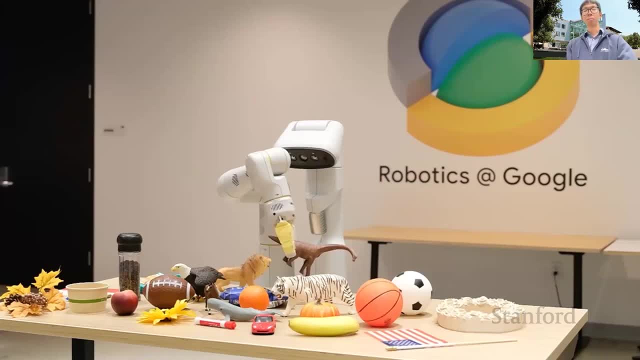 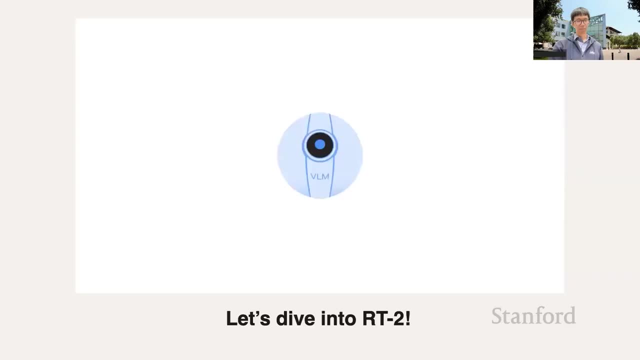 And as we run more evaluation, maybe there will be some replication as well, But, as you can see, it is able to understand to pick up this dinosaur toy. How did we do that? So we start from a vision language model that is trained on internet scale data. 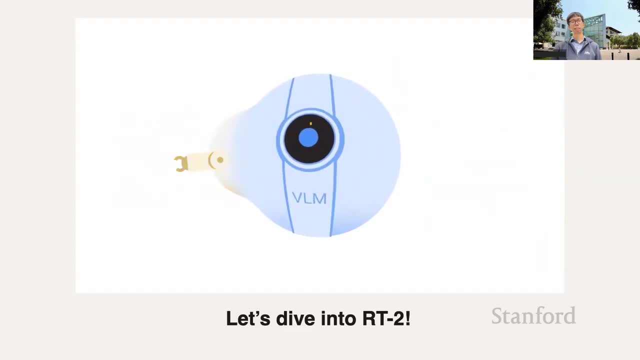 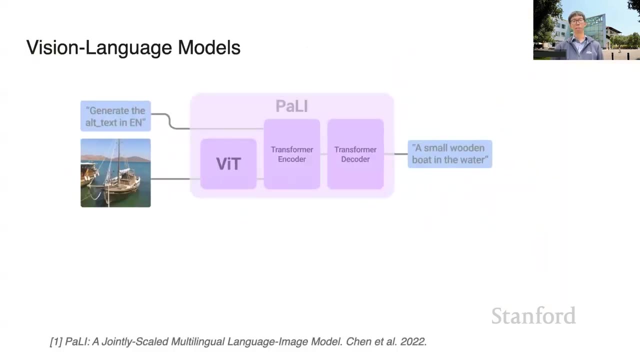 And then we also combine it with robotics action data, which is the RT1 data, and we get RT2.. And we can dive deeper, a little bit deeper into RT2.. So first, what is a vision language model? A vision language model is a transformer. 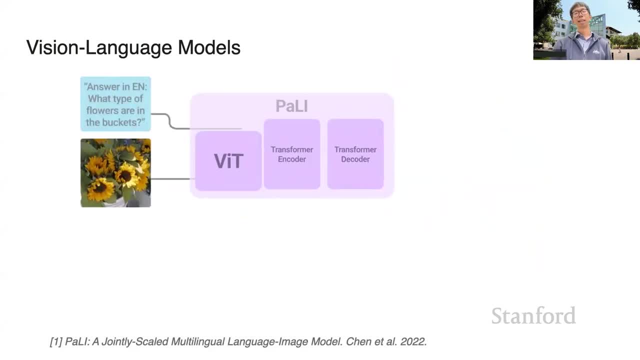 that takes in image and text and then output text. So within Google there is a vision language model called Pali, which is an encoder-decoder type of architecture. It's basically having a VIT to understand the images and then a transformer encoder. 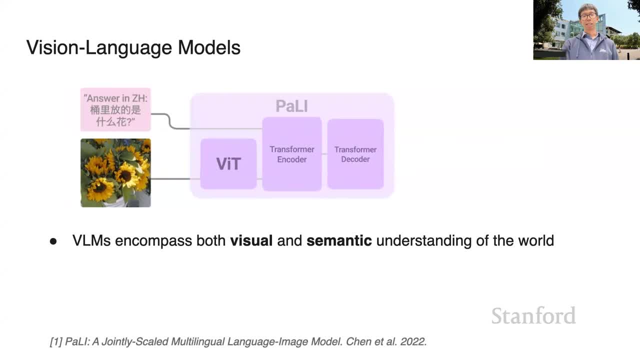 and the transformer decoder. They encompass both the visual and semantics to understand the world, And in robotics we have to deal with a lot of both of these And the question is: can we leverage the knowledge in the vision language models and apply them to robotics? 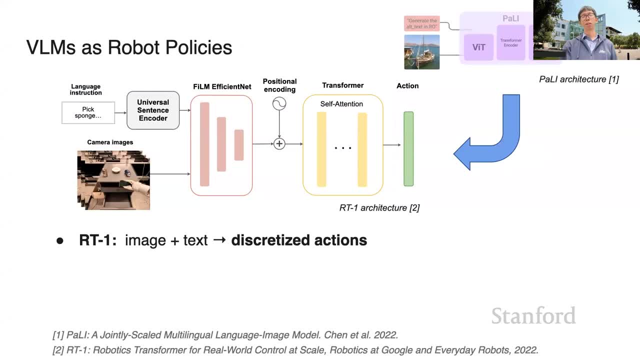 On the other hand, we have the RT1.. If you want to learn more about RT1, you can listen to the previous episode of this CS25 by Ted, So he gave a detailed introduction on the RT1. But the RT1 is. 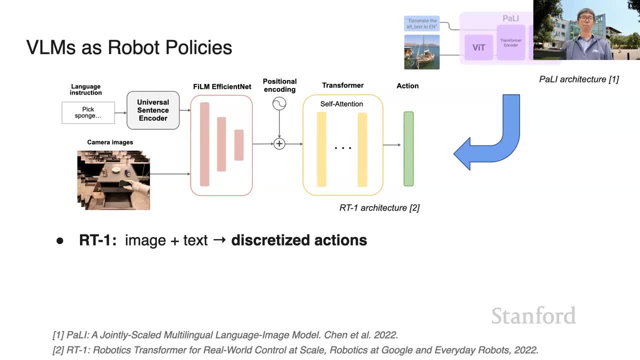 if you stand far enough. it is also a vision language to action or something model. It takes in human instruction. It takes in the current camera image. The camera image pass through a film efficient net which is tokenized into 81 tokens and then going to a token learner. 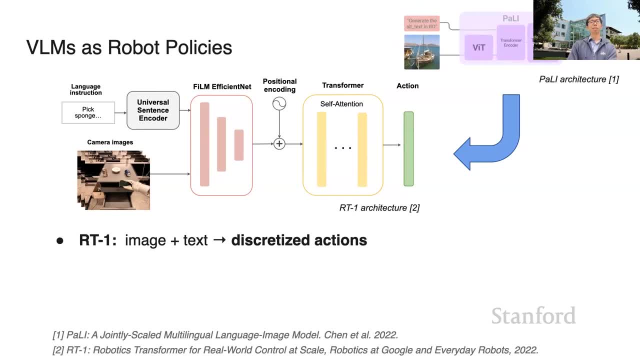 which compress everything into eight tokens. And then there is a transformer block leveraging a lot of self-intention layer and then generate actions. The action is also tokenized. The robot have seven degree of freedom. Basically, the end effector has six degree of freedom. 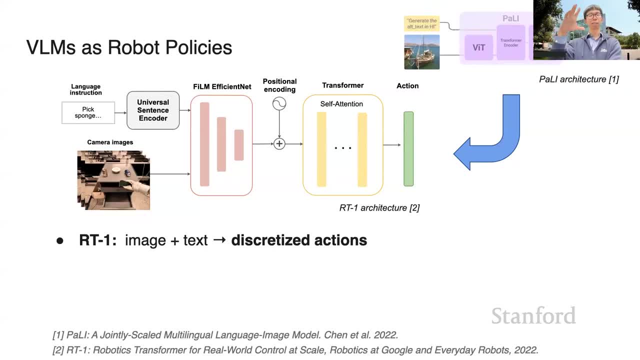 Its position and the rotation and the gripper can open and close, And there is another dimension representing terminate the episode or not. Terminating means my task is already done And we discretize every dimension into 256 bins And then we do cross entropy loss on those bins. 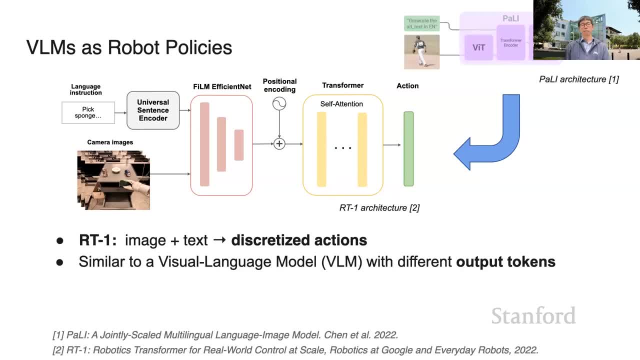 So that's the RT1 architecture in a nutshell. It's quite similar to a vision language model with different output tokens. So it's rather natural that we just use a large, pre-trained vision language model directly as policy. We can use the poly or polyme as a policy. 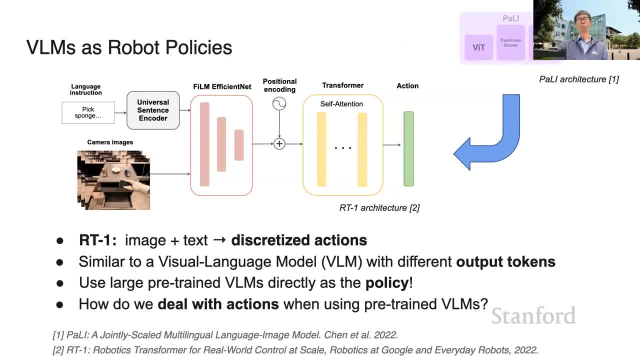 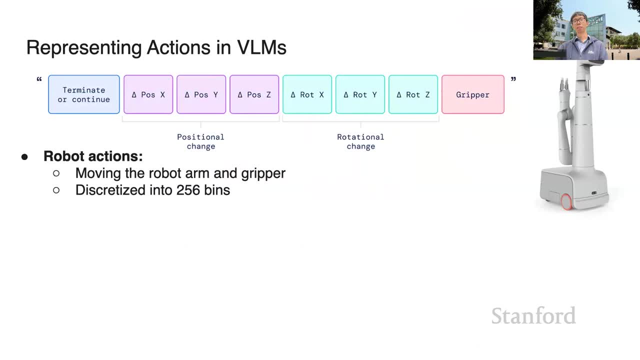 And one question is: how do we deal with actions when using pre-trained vision language models? And here is action representation that we use The robot actions. here are the eight dimensions And, as I mentioned, there's termination, position change and rotation change. 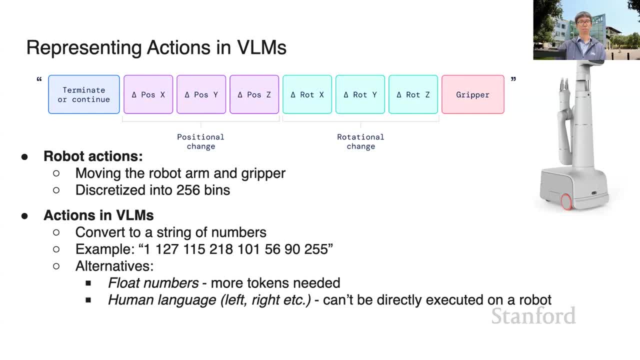 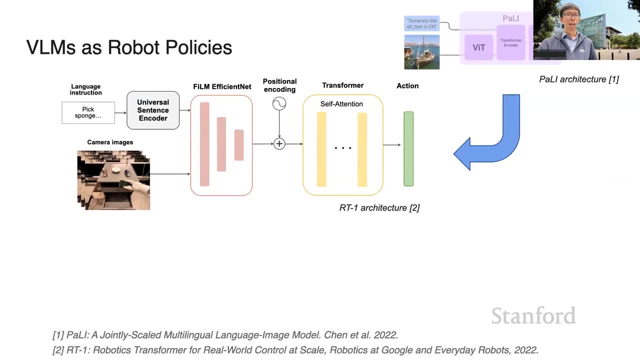 And we discretize everything into 256 bins. We also have tried other alternative representations, but they are not as good as just this, like naive representation. Yes, Can you go back to your question? Yeah, What is Film EfficientNet doing? Oh, the Film EfficientNet is a pre-trained. 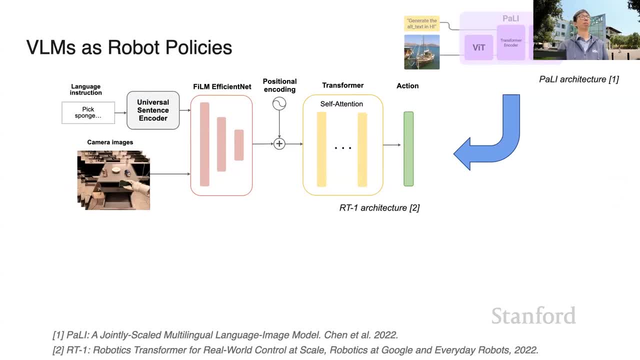 convolutional neural network. It's used to tokenize the images. So the reason that we do this is through some ablation study. we can tokenize the image in different ways We can. We can tokenize in ResNet. We can tokenize everything into ResNet. 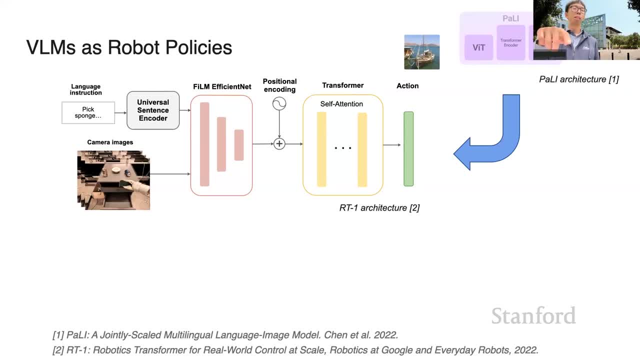 And we can tokenize using Film EfficientNet Film. what it means is it also takes into the language embedding and append it to the intermediate layers of the ResNet, So we basically have like some compadination of the other sentence, encoder and the conventions. 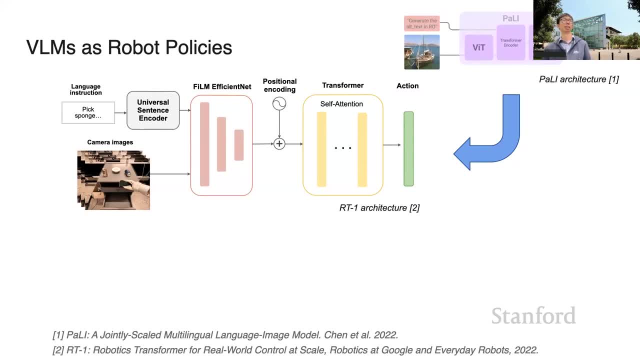 Yeah, And that goes through this neural network, this foundation layer. That's right, That's right. And then we transform it. So you're saying that the action and the output go to action. training, That's right, Is action, as in the code. 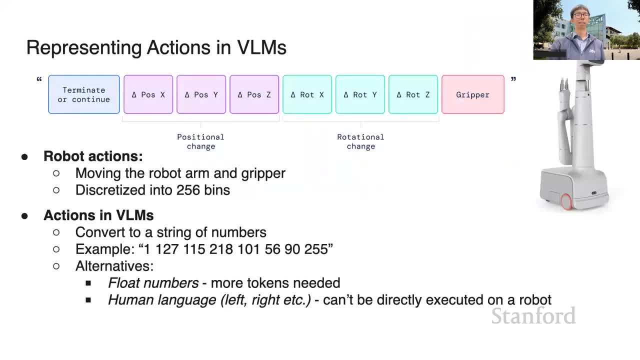 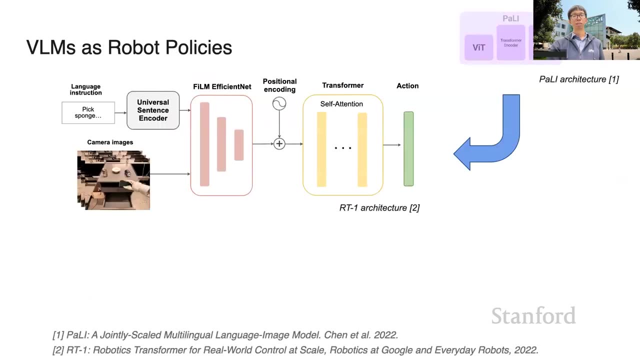 The action is not in code. The action is in text. It's basically what is shown here And this is the action. It's eight numbers. Each number range from 0 to 255.. Yeah, And maybe another note on the Film ResNet. 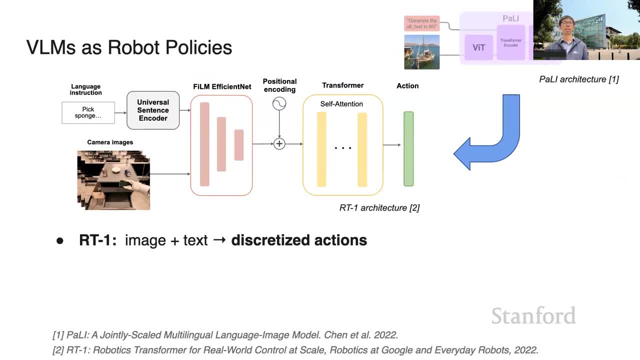 It's about how we tokenize the images and how we combine vision information and language information. There are many ways to do that. This is not the only way. There is early fusion and late fusion, And there is also cross-attention. You can basically tokenize your image. 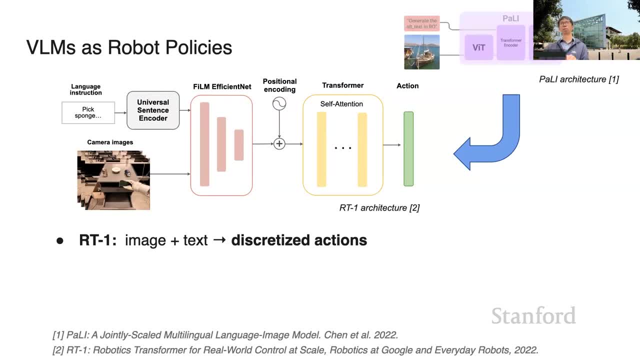 just by itself, And then you can have language and use cross-attention to combine the image and text representation. So here we are using this model. This is RT1 for robotics, So we do have a lot of considerations such as latency. That's why we use this Film ResNet. 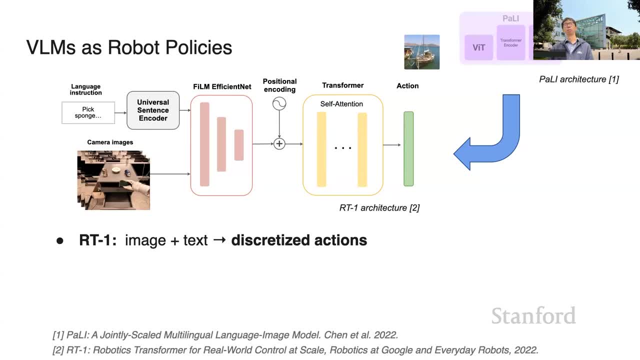 because it's super fast And it can output a limited amount of tokens which we can further compress with Token Learner. Yeah, And is this autoregressive? Like every single image it sees, it then runs this machine Right, So it is autoregressive, yeah. 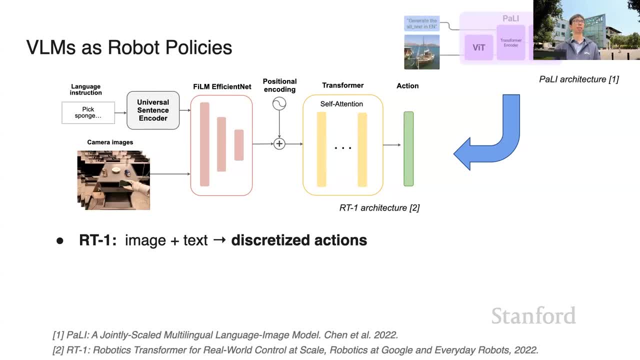 And every time we use a history of up to six steps. So every time you see this image right now and you see about two seconds of history before it And this will be your input. Yeah, Again, if you have more questions about RT1, I recommend watching. 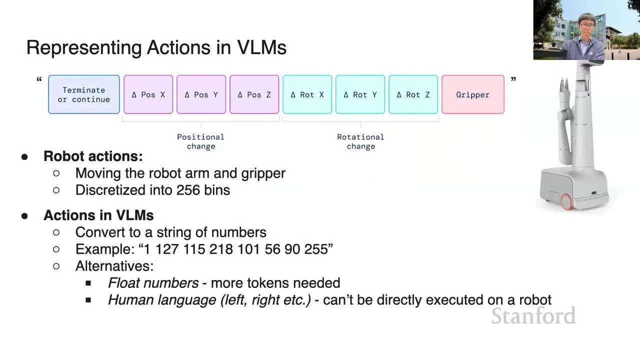 the previous episode And here is all about RT2.. So we can convert the string of numbers. This will be our output of our transformer, which is a vision language model. We tried other alternatives, such as floating numbers. Floating numbers is not super friendly. 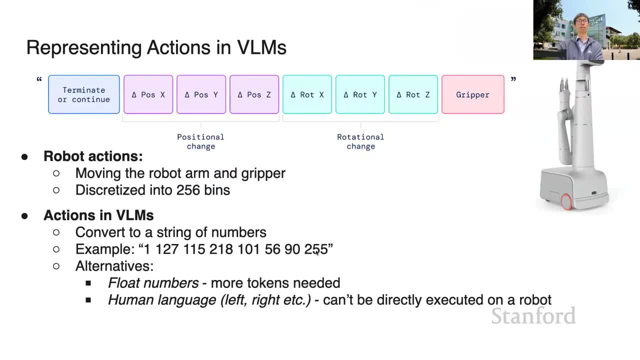 to language model tokenizer Because it has these decimal points. We also tried the human language, such as left or right. It's more semantic representation, But it cannot be directly executed on a robot, which is a limitation of this method. So if we commit, 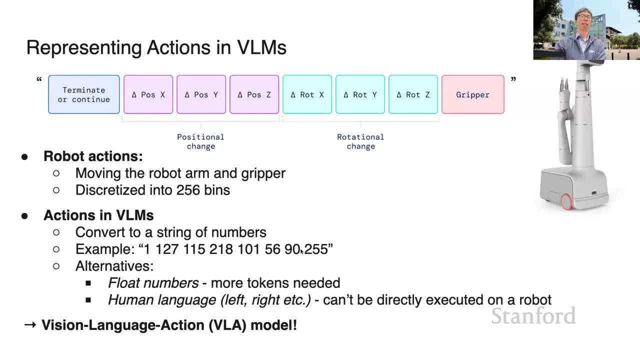 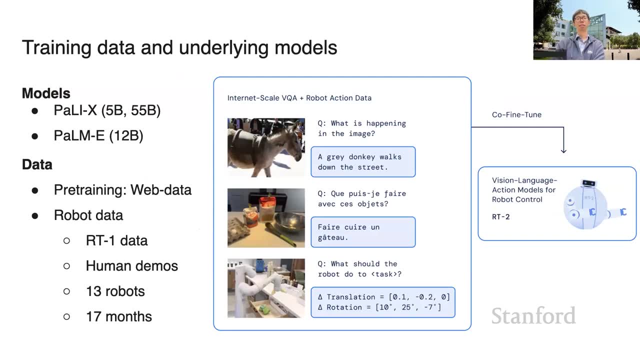 to this action representation, which is just a string of numbers, we essentially get a vision language action model. We tried different variants, including PolyX. This is a pathways language and image model. There are 5 billion parameter variants and 55 billion parameter variants. 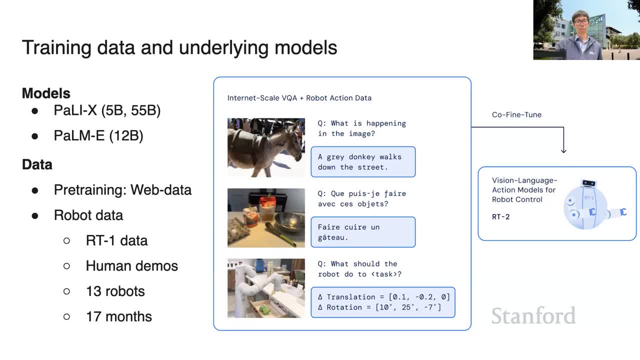 And we also tried POMI, which is 12 billion parameters. The procedure that we did to train this RT2 is via cofine tuning. Cofine tuning is to put the internet scale data and the robotic data together And then we fine tune it. 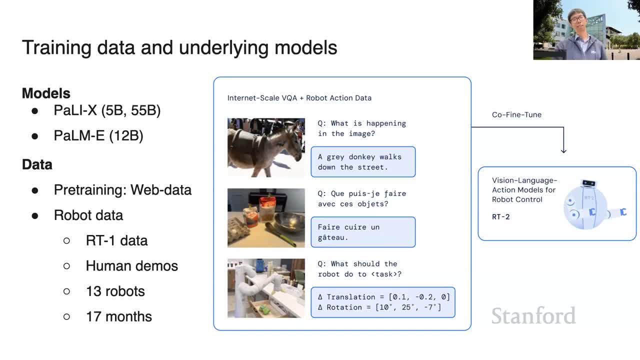 on this mixture of data so that it retains the internet scale data. Maybe that's also an artifact of our data is too small and not diverse enough. So if you just fine tune on robotics data, it will quickly overfit and forget about all this protruding mixture. 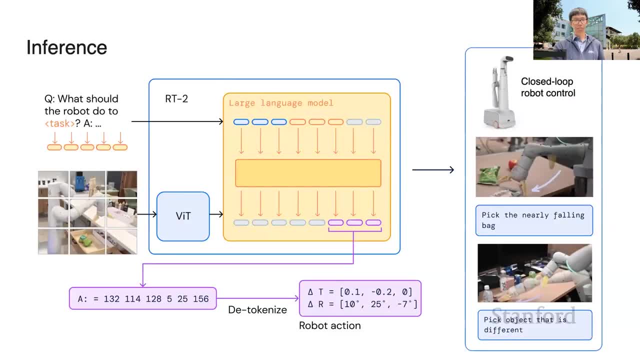 Maybe it's a dynamic of scale. So we'll see At inference time how do we do this. Again, we do this auto-regressively. We have an instruction of a function called task And we format this as a question and answering task. 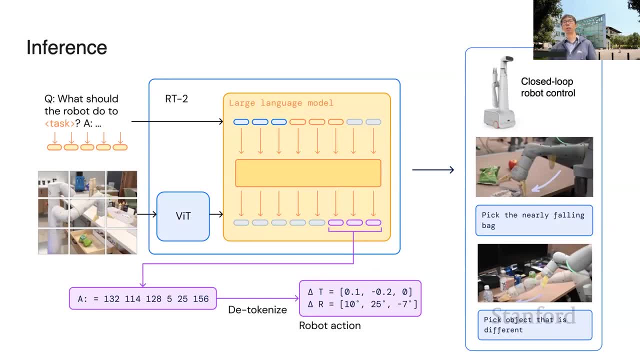 What should the robot do to achieve a certain task? And the task is a string that humans give the robot for the robot to achieve. And it also has the current observation, which is the robot observation, the camera image, RGB image, passed through a VIT and then passed through. 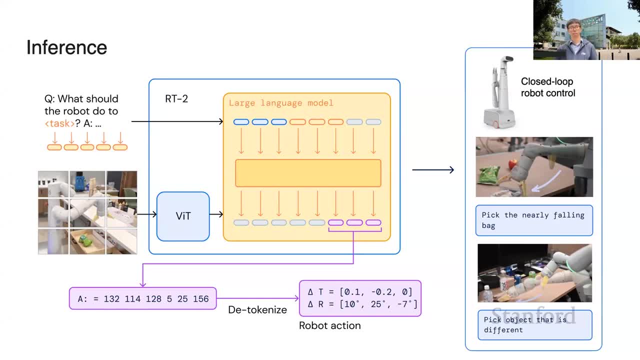 the large language model and we leverage constraint decoding to make sure it always has eight numbers, because otherwise we cannot de-tokenize it. It's very easy for a language model to just miss one number. So we do have some mechanisms such as constraint decoding and beam search. 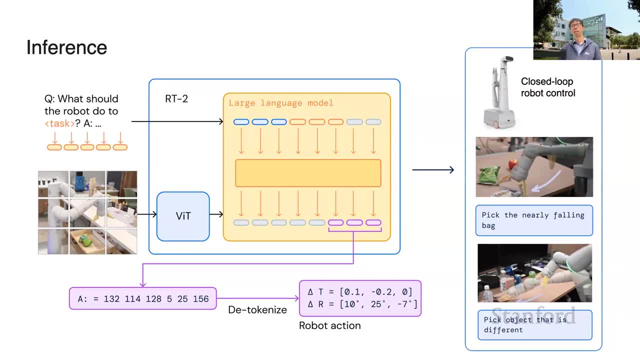 to make sure the format is correct. After we get a string of eight numbers, we de-tokenize it to a delta t and delta r and run this on the robot. After the run on the robot, we repeat this process. We get another new image. 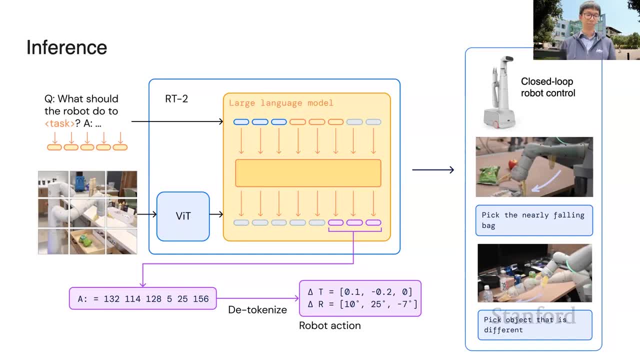 run through this process and get a new action And we repeat this process until a termination is decoded. So some people might be concerned that this is rather slow. It's in fact quite slow because it's 12 billion parameters or 5 billion parameters. 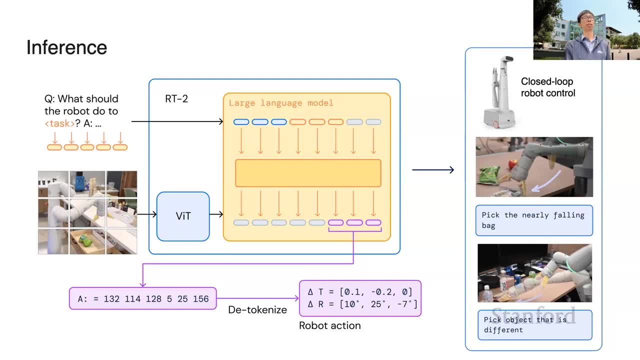 We cannot run on a robot, so we run on a TPO cluster to get the numbers and apply it on the robot. So for the 12 billion parameters we can actually run at 10 Hz, so it's quite fast. For all those models we can run at at least 3 Hz. 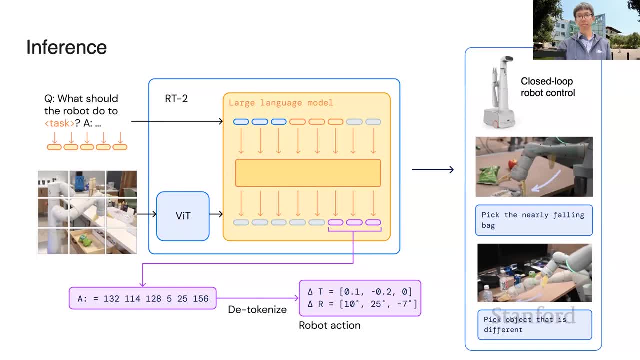 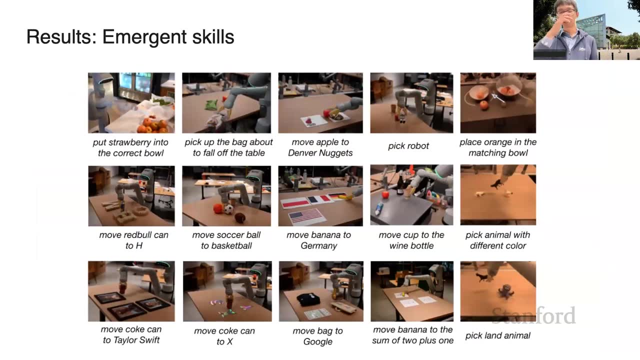 so that is sufficient for controlling a robot And we see a lot of emergent skills that is not trained, that is not on the training set. Essentially, as I just mentioned, we are probing what this RT2 can do. We actually don't know. 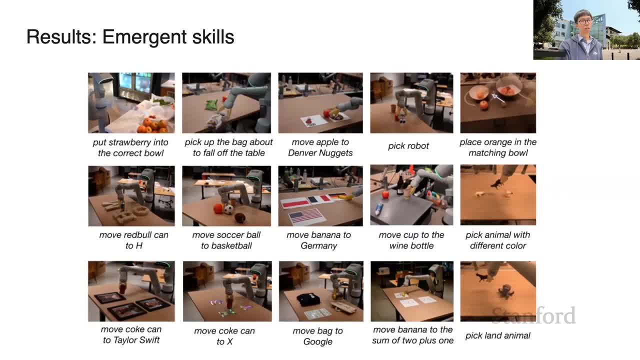 so we are trying to figure out what RT2 can do. So we test it with a lot of new tasks, such as putting a strawberry into the correct bowl or moving a banana to Germany, just to test its understanding of symbols or flags. Pick a land animal. 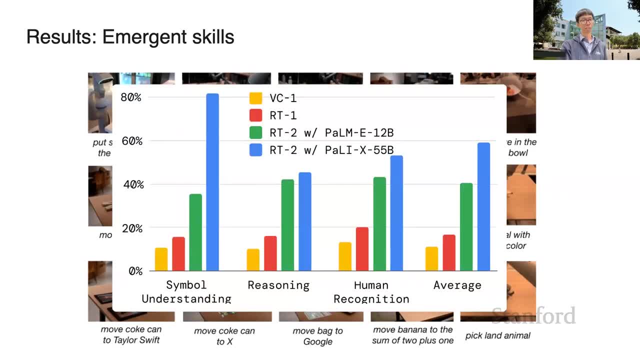 there's a horse, there's an octopus- and basically test its semantic reasoning and also low-level manipulation skills, And we divide the tasks into symbol understanding and reasoning and human recognition and average. We found that with RT1, which is not trained on internet-scale data, 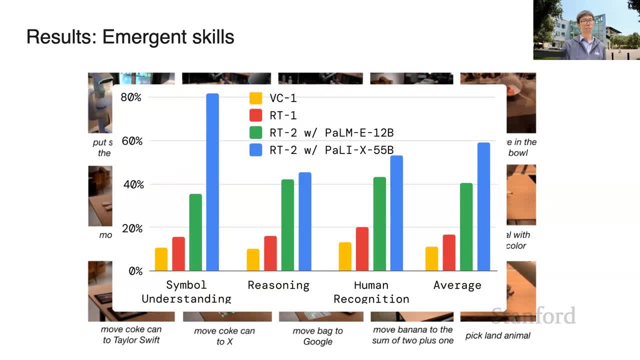 we do quite poorly in these emergent evaluation tasks And in the RT2 variants, which is co-fine-tuned on the internet data and on robotics data, we do much better in these tasks. There's also an effect of scale, so the RT2 with 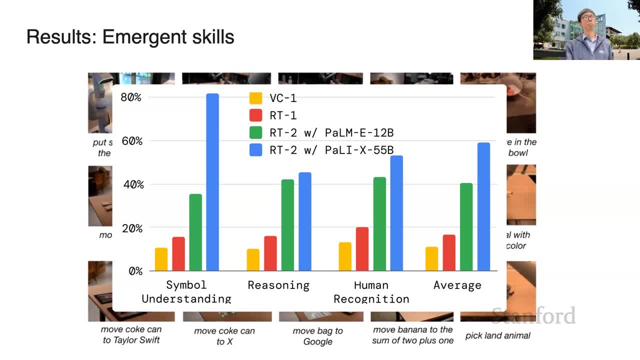 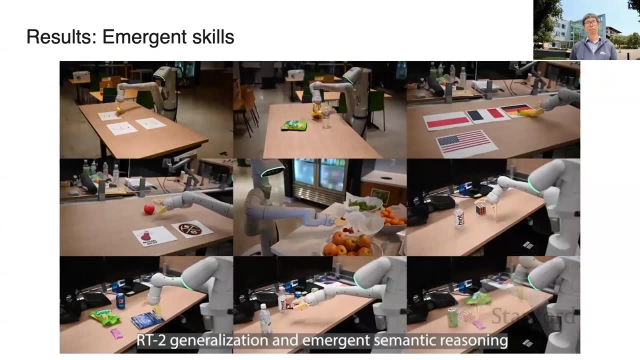 a 55 billion poly is performing better than the 12 billion poly, although they perform quite similarly for in-domain tasks. But the generalization is kind of interesting. It seems with larger scale you can generalize better. And here are some videos of the robot. 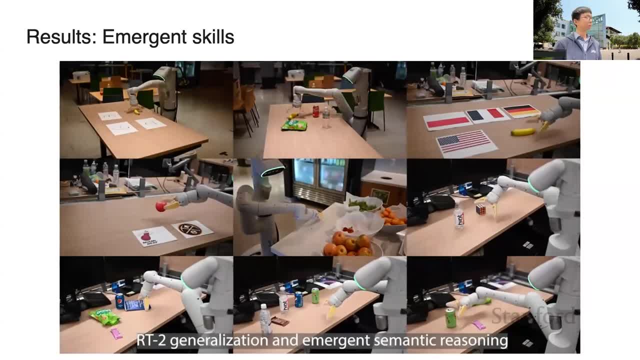 achieving these tasks like moving the banana to a number, put the strawberry into the correct bowl, move a Rubik's cube to the water bottle- but I'm speaking Chinese- moving the banana to a German flag, so it's able to do all of these very interesting tasks. 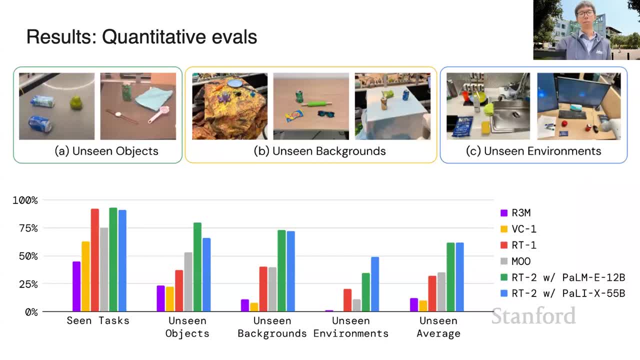 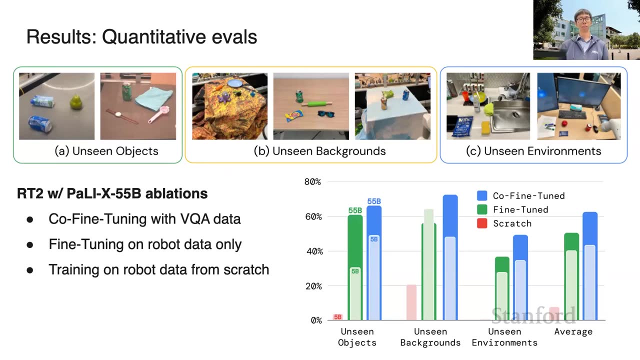 In terms of the quantitative evaluations, we also found that the RT2 policy is quite robust to unseen objects, unseen backgrounds and unseen environments, And here is another evidence of positive transfer. so, co-fine-tuned with VQA, data outperforms fine-tuning. 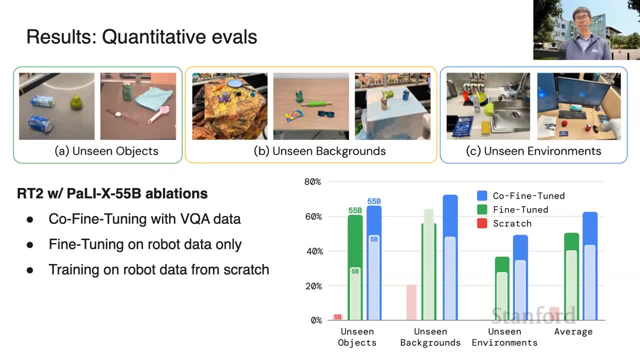 on robotics only, And if you train on robot data from scratch, it barely works, it almost doesn't work, because it overfits to robot data and our robot data is just too small. So we do need to do co-fine-tuning, or at least fine-tuning. 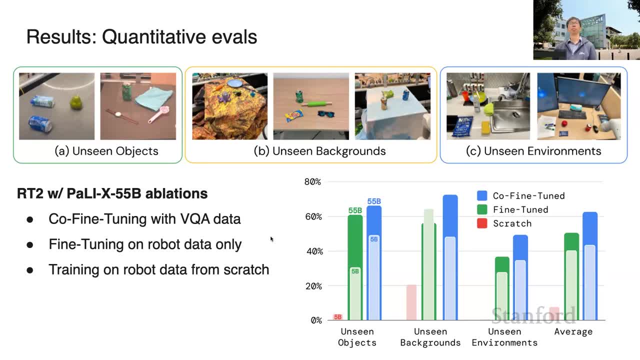 so it retains its internet-scale knowledge. This is also a recipe for how people would develop a domain-specific vision language model. so you start from a very general knowledge model and you fine-tune on your domain or you can co-fine-tune with your specific domain data. 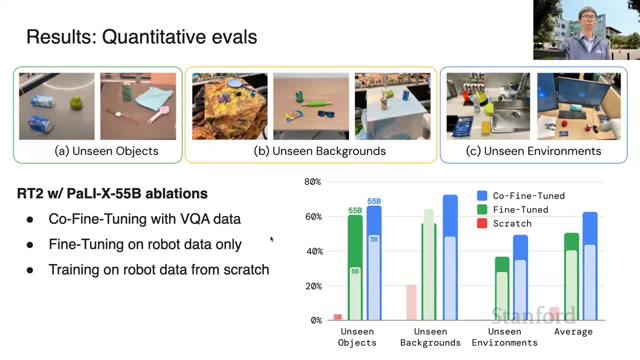 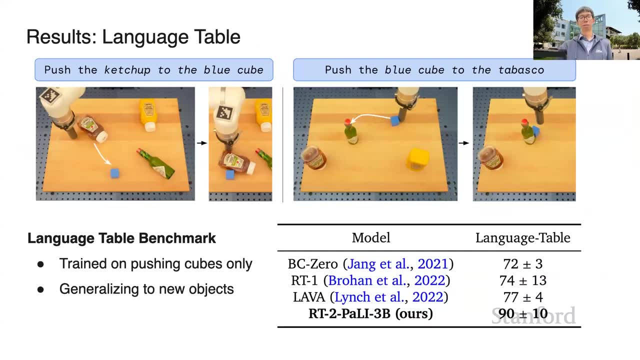 This is likely a problem that each vertical of artificial intelligence would incur someday. We can also test on other platforms like. this shows some cross embodiment. the RT2, Poly3D outperforms previous models in terms of moving blocks around to the environment And in large language models. 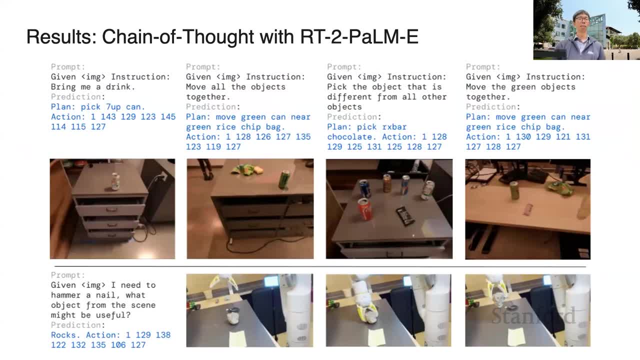 we have this chain of thought reasoning, which is a method to elicit reasoning in large language models. You can either do zero-shot chain of thought reasoning by, say, eliciting step by step, or give it examples of reasoning. it's basically decoding more things and then come to the conclusion. 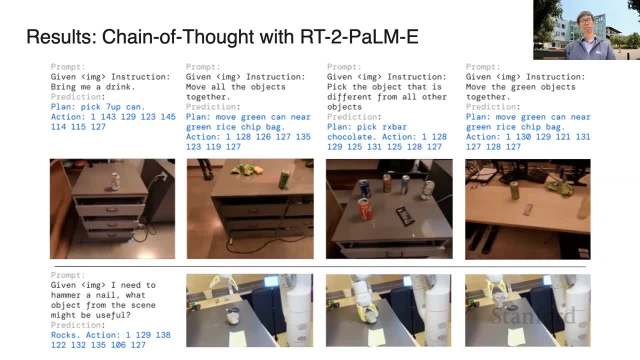 We can use a similar procedure for the RT2 as well. So in RT2, PalmE, instead of directly decoding the actions, we can candidate with actions. So this gives the language model an opportunity to understand the question or parse the question differently. It also gives us the opportunity 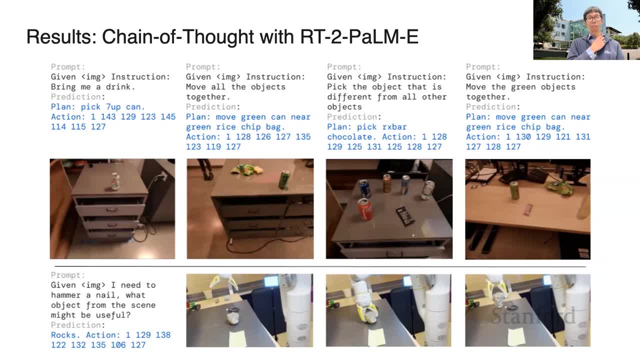 to reason about things a little bit. For example, if you say, bring me a drink, and it would say: pick up 7up can because there's a 7up can on the table. So we synthesized a couple hundred such examples using a large language model. 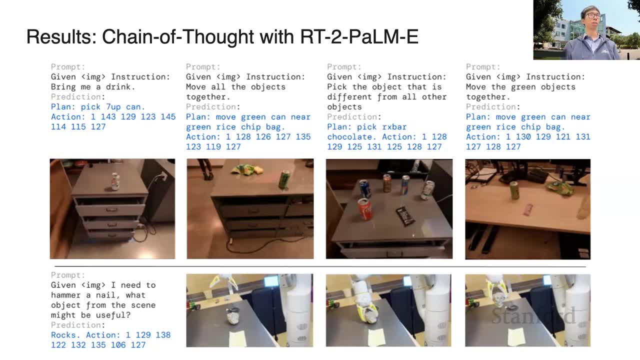 just by augmenting the instruction and then fine-tune the RT2 just for a couple hundred steps. So it's able to do some fine-tuning and in-context learning and it's able to do some reasoning And some of the interesting reasoning tasks include: 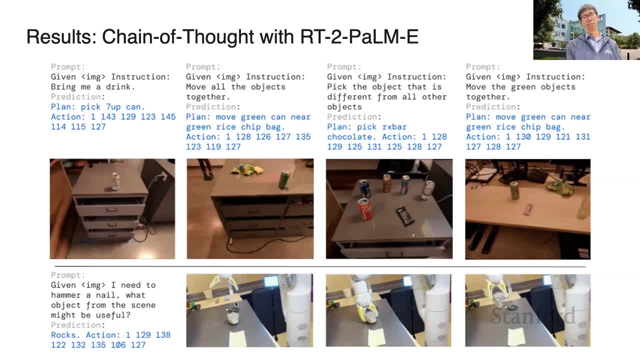 I need to hammer a nail which object from the scene might be useful, And in the scene there is a headphone, there is a rock and there is a sticky note And the robot will say rocks and then generate actions to pick up the rock. So it's interesting that it's able to do. 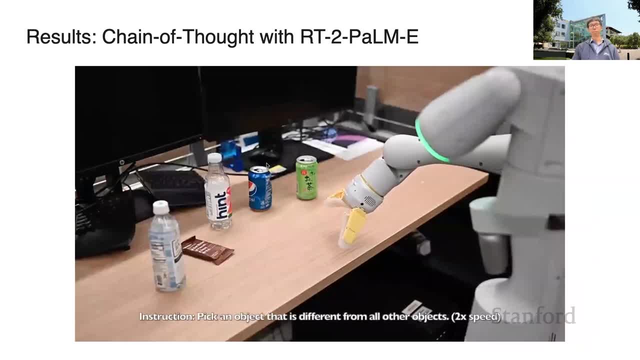 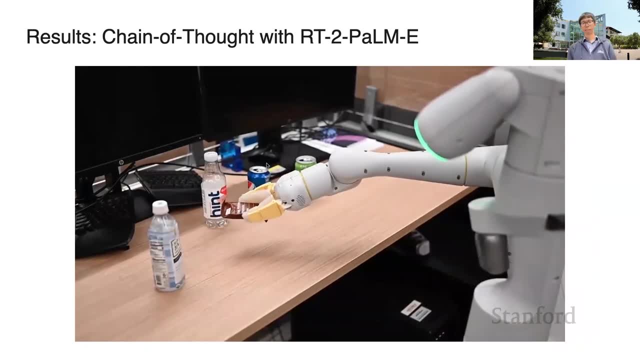 this sort of reasoning with RT2.. And here is a demonstration of some of the chain of thought reasoning and the task is: pick up the thing that is different from all other objects. and it picks up the chocolate because this is a snack and other things are the drink. 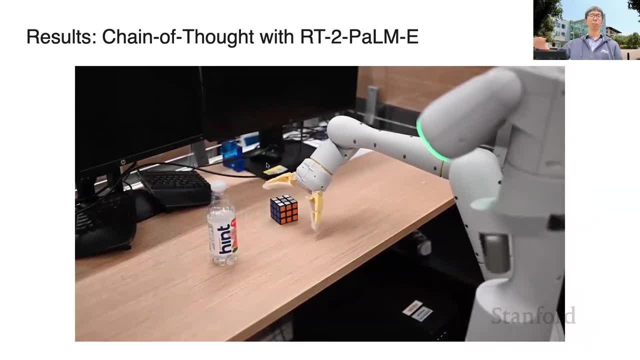 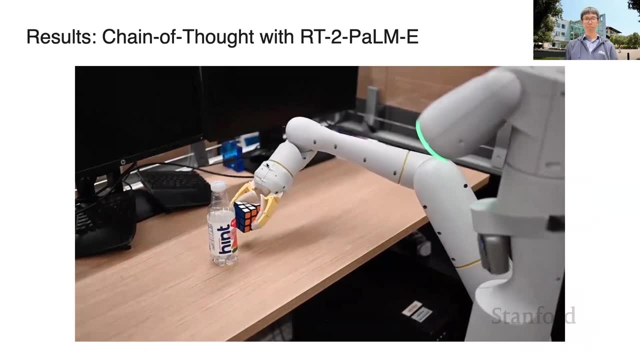 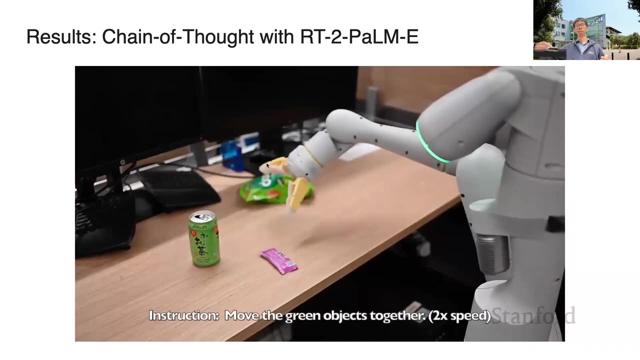 And I can also speak a different language, and the plan would be to translate it into a language that it's familiar with, which is English, and then do the task. There are also potentially a failure case of the chain of thought reasoning. So here I say: move the green object together. 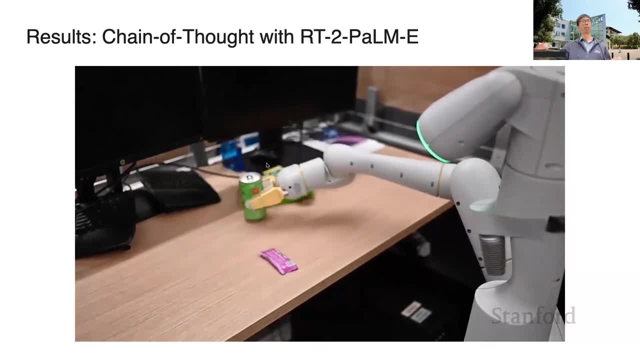 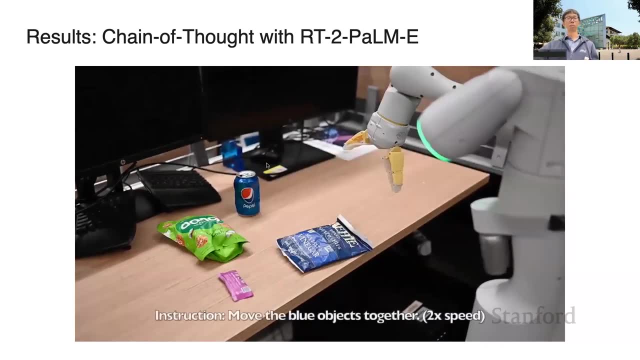 and, as you can see, the robot is moving the two green objects because there are rather two plans. It could move the can to the bag of chips, or it could move the bag of chips to the can. It oscillates between two plans until one action. 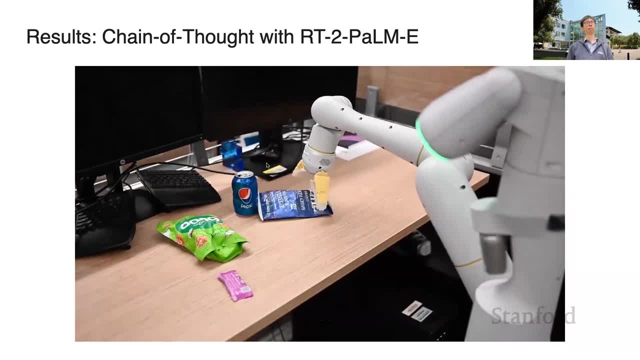 brings it to an object and it will commit to one of the plans rather than another. It's not always guaranteed to work, but it's quite interesting. And it's also interesting that again we are testing the manipulation policy, like how we test intelligence of humans or animals or kids. 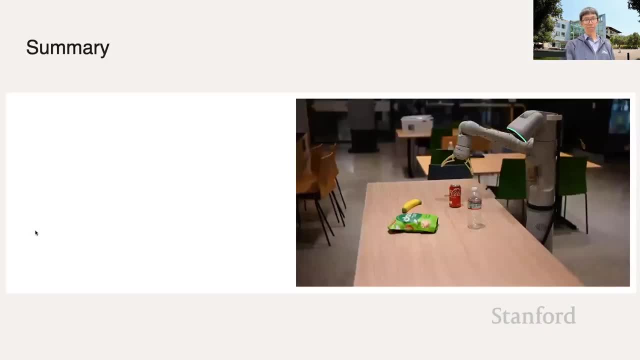 Because they're getting more and more advanced. As a summary, we have the vision, language and action model that is able to achieve, improve the generalization. It can do new tasks and operate new objects. It can also do chain of thought, reasoning and improving. 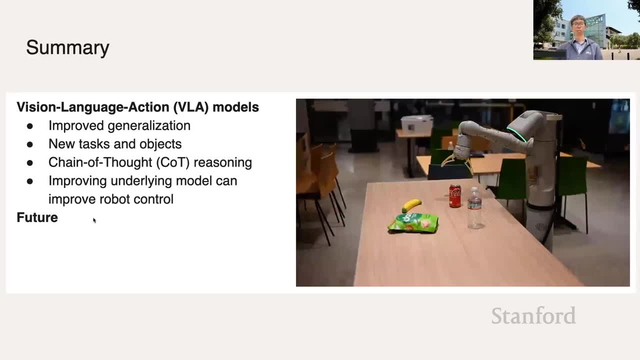 the underlying model, such as the vision language model itself. by scaling it up and training it with internet scale data or training it with larger or higher quality internet scale data, We can achieve better robot control, which is quite amazing because robotics field has been traditionally developing quite slowly and is bounded by 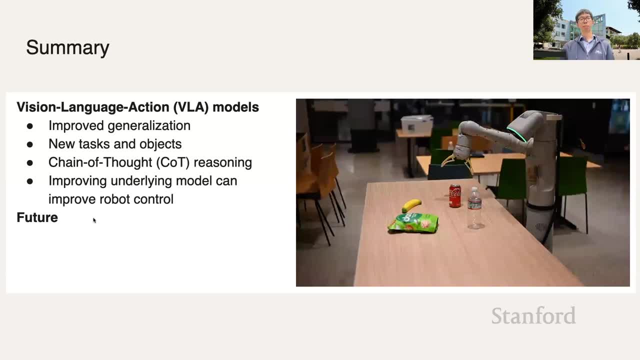 hardware, bounded by a lot of different things, bounded by operation, But now it seems we can piggyback on the development of the foundation model field, and whatever they do will trickle down to our field as well, And the future will be to increase. 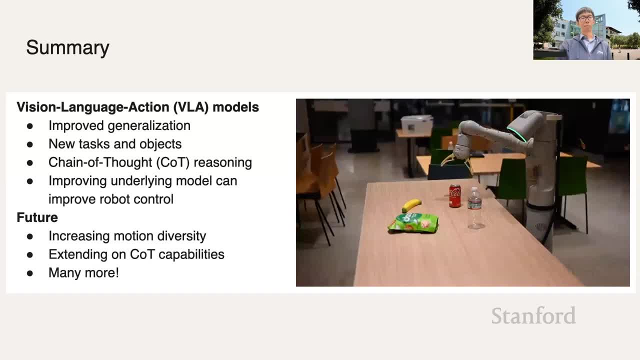 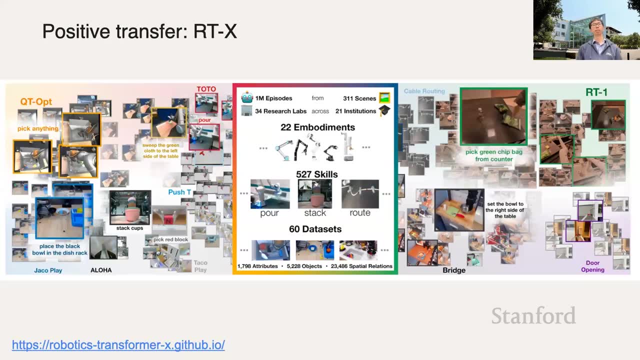 the motion, diversity and extent on the chain of thought reasoning capability. And so there is another example of positive transfer which you might have seen recently. So far, I've been talking about scaling differently. I've been talking about: don't scale robotics data and scale other data. 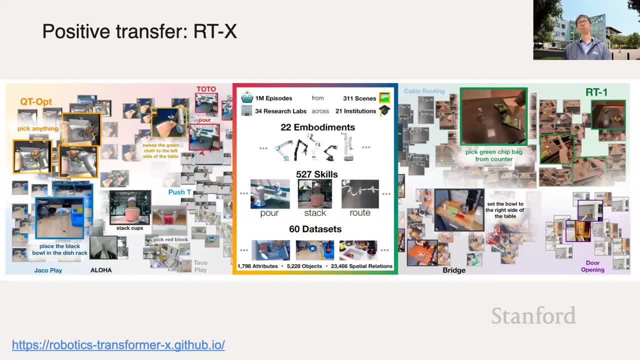 That's because robotics data is so hard to collect, and the purpose is not to avoid collecting robotics data. It's to develop a recipe that you can do more with limited robotics data. However, there's also an effort from our team and the entire robotics field. 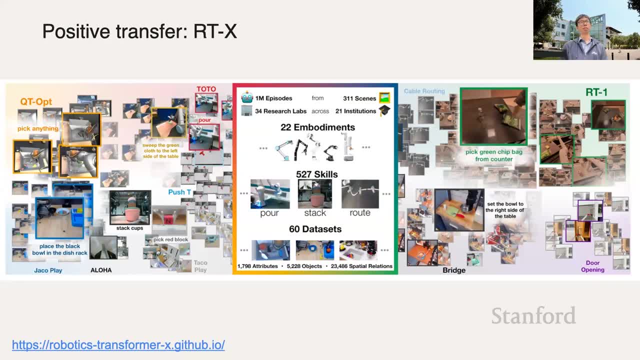 to scale up the robot data collection, which is called OpenX Embodiment, And the model chain is called RTX Robotics Transformer X. It's basically 22 types of embodiments and 572 scales and 60 datasets pulled all together, So this will be the ultimate dataset we can use to study. 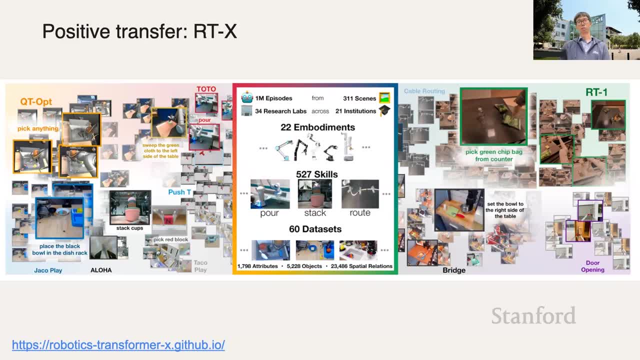 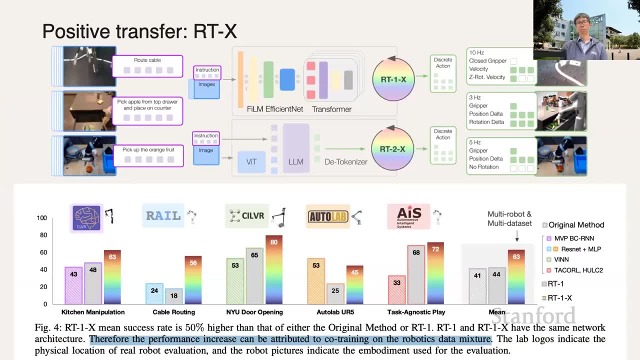 positive transfer and to study this joint scaling, And there are already evidence of positive transfer. So we pulled all the data together from all these labs and find a common action representation that we can use to train a robotic transformer. And we have already found this. 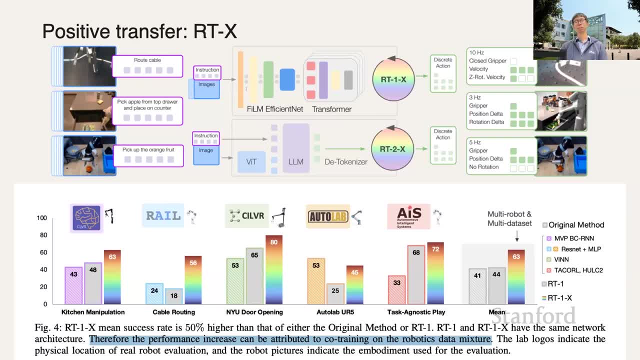 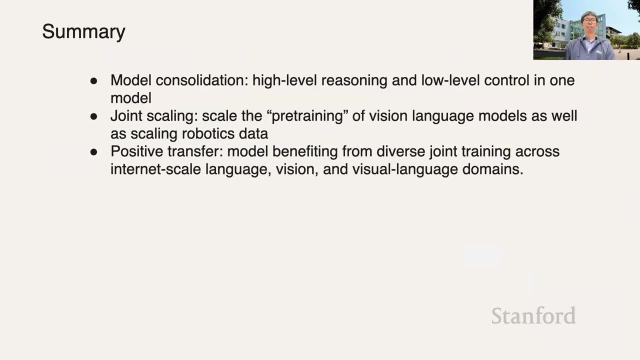 jointly trained model can outperform task specific model that is developed in each of the lab. So there's some benefits in pulling all the data together. Scaling robot data is also quite important. So the summary for this part is that we are having a model consolidation. 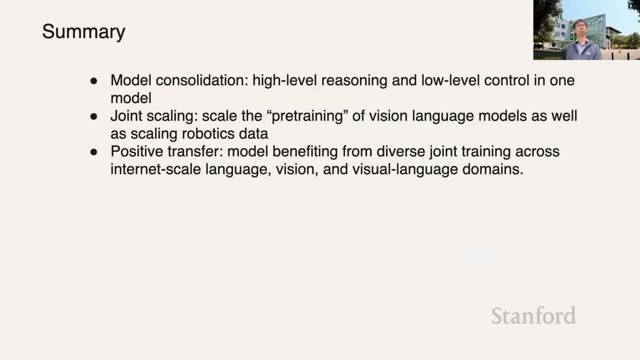 We can now do the high-level reasoning and low-level control in one model, And the low-level control part is what excites me because it's so far away from the traditional language model domain, It's so different And it shows signs of life. 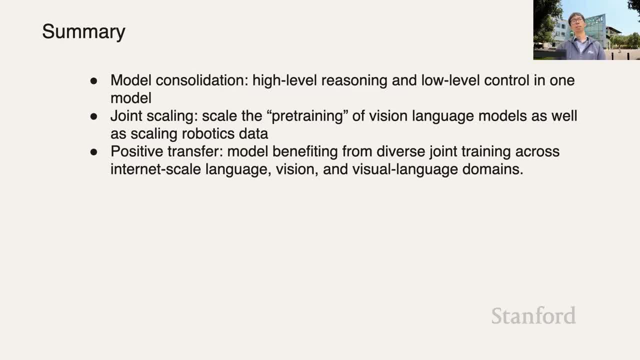 that we can trickle down a lot more than we used to think is possible And we can scale the training of vision language models as well as scaling robotics data, And we observe more and more positive transfer model benefiting from diverse joint training across internet scale language, vision and vision language domains. 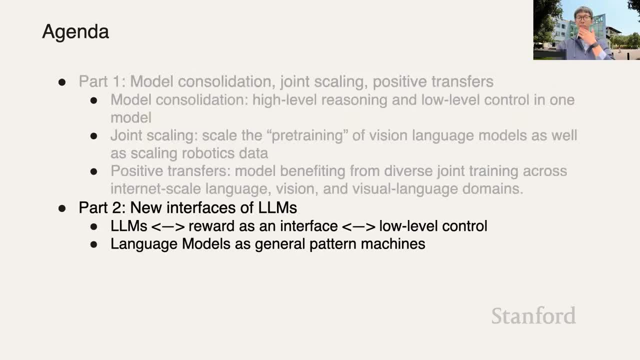 All right. So I noticed that we are close to running out of time, So I will just very quickly go through the second part, which I think is also interesting. It's to find new interfaces of language models, But I will only talk at a very high. 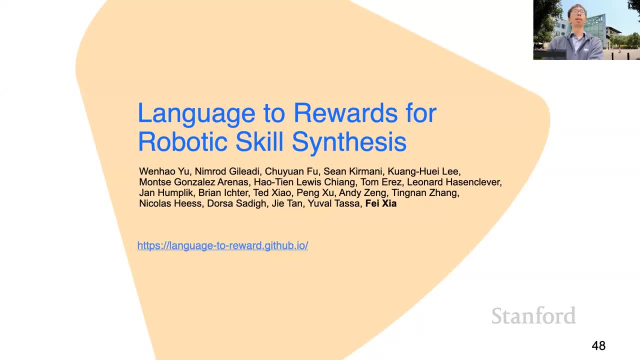 level. So language models, as we can see, can directly output action tokens. if we found action representation, So we can treat action as yet another language to the language model. So language model can do translation, So it should be able to generate action as well. But that requires fine tuning. 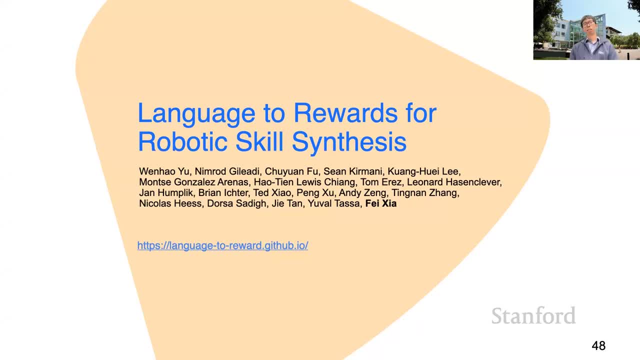 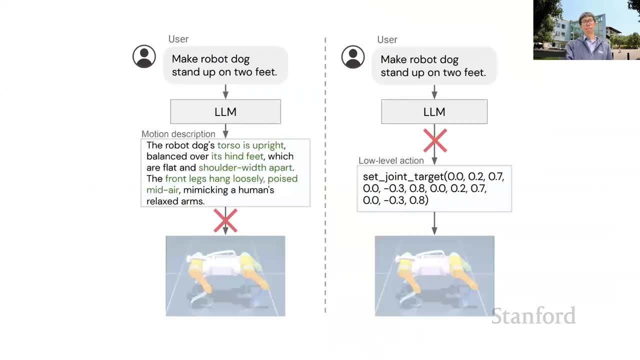 Can we do it without fine tuning Or can we generate more expressive actions? that is beyond the scope of fine tuning. So that is about finding the right interface. So previously we have already established that language model doesn't have an action interface If it has an action interface. 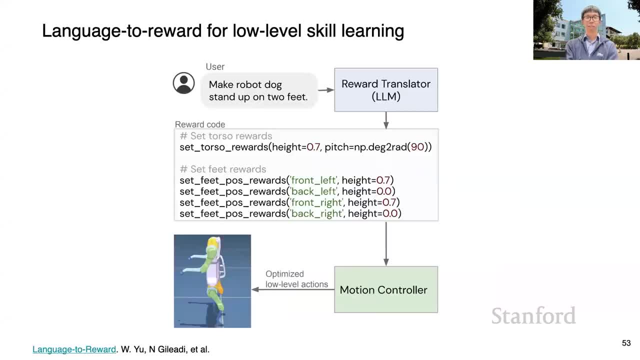 it's not as effective. So what is the best interface between language and low-level actions? I would argue the best interface between language model and low-level actions is reward functions, And reward functions is universal. It has been used in reinforcement learning And it's also. 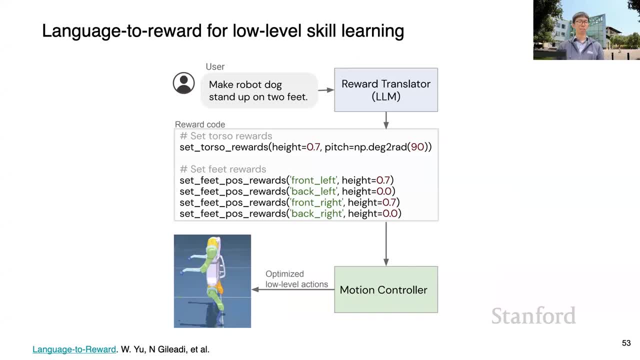 a reparameterization of actions. What is action? Let's see if I want to pick up this bottle And I can say what is a skill? A skill is a mapping between my observation and my action. So the mapping between my observation. 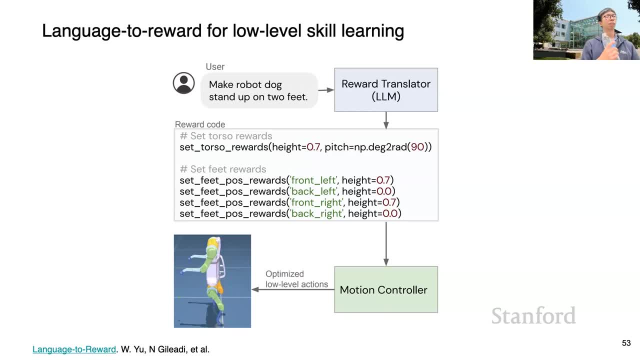 and action can be seen as a skill. But a skill can have an alternative definition, which is a set of constraints and a set of objectives. So picking up the bottle means the bottle is in my right hand and the bottle is off a supporting surface. 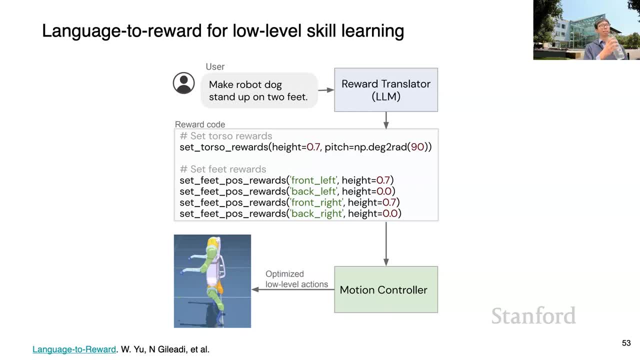 That means picking up, And how do I pick it up doesn't really matter. That's a more to its broader sense, a definition of skills. It's more transferable between different skills And the constraints and objectives can be represented as rewards. 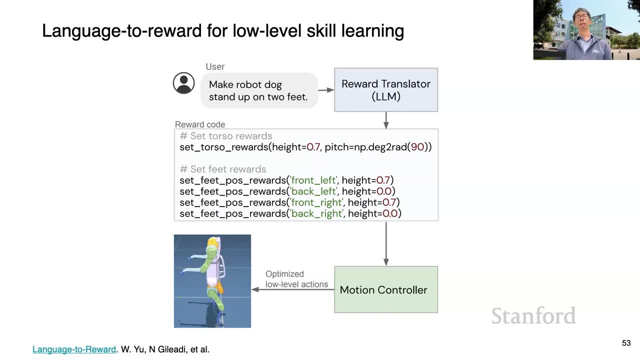 So we can ask language model to generate these reward functions. And then there's an optimizer. It could be reinforcement learning or it could be model predictive control that optimizes for those rewards and then runs it on the robot. So what is in the reward translator? 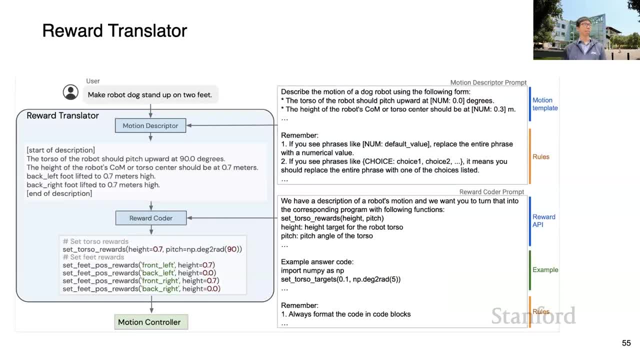 Let's open a box. So the reward translator basically is a two-stage process. It's using the same language model and it is using two different prompts. So the motion description basically describes the motion. So just now we found that the language model can output a description. 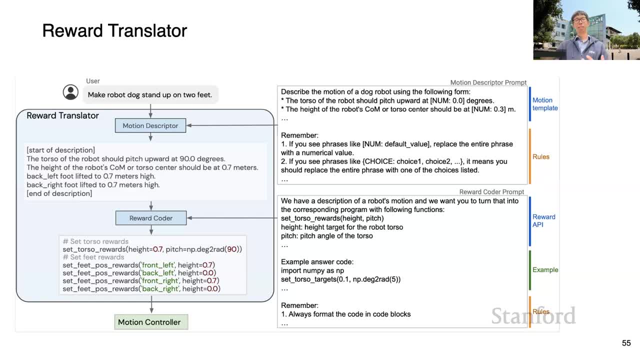 of how a robot dog should stand up, But it's not able to achieve that. But the motion description is still sensible, It still makes sense, It gives you the right thing. So we just generate this motion description and then we have a reward translator- a reward. 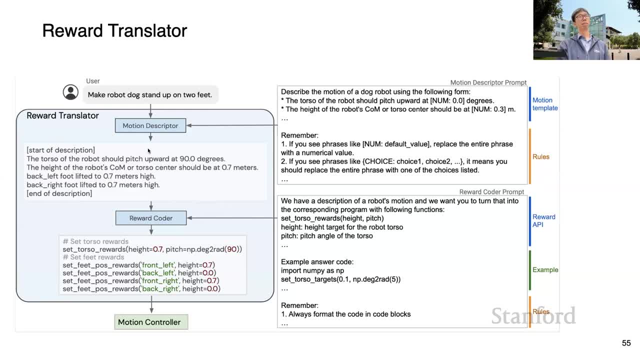 coder that translates this motion description into a piece of code that is representing reward functions, And these reward functions cannot be directly executed on the robot, but it can go through our optimization process to learn how to achieve those reward functions. So we're using reward. 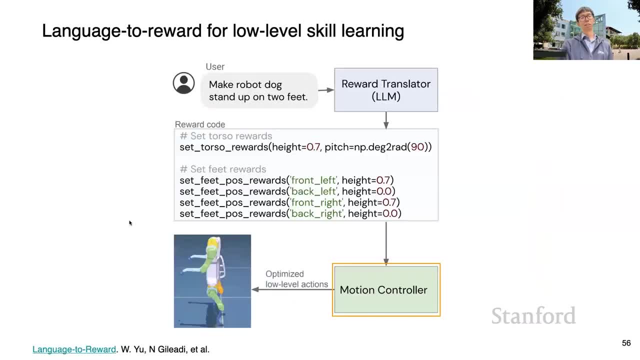 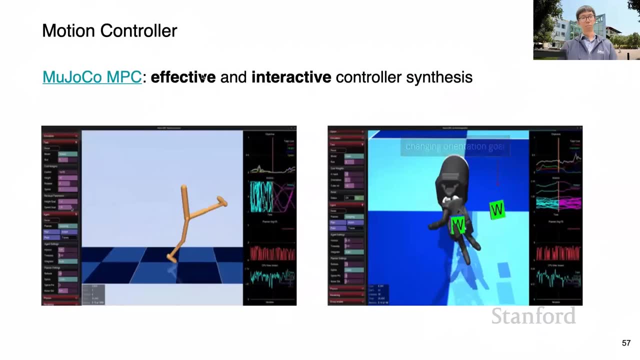 as the interface between language model and a low-level controller. And for the low-level controller we're using Mojoco MPC, which is a model predictive control algorithm. It's basically a black box controller. It samples a lot of trajectories and finds one that 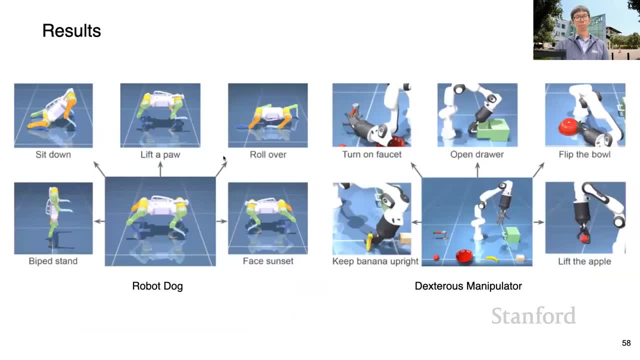 optimizes your reward. And we tested on a robot dog, a quadruped robot, essentially, and a dextrous manipulator. So the dextrous manipulator has an arm of six or seven degrees of freedom and a hand. It's impossible to control it because it. 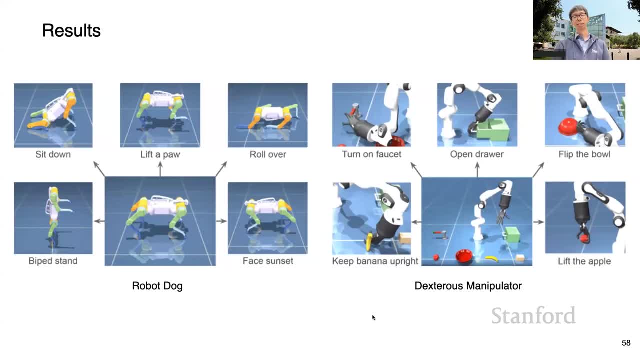 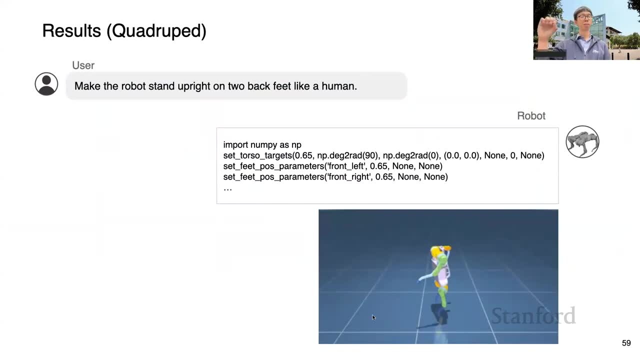 has so many degrees of freedom, It's highly challenging. Just to showcase some of the examples, I omitted the motion description part. I only output the reward code part. So it seems that the language model is able to generate the right reward functions to 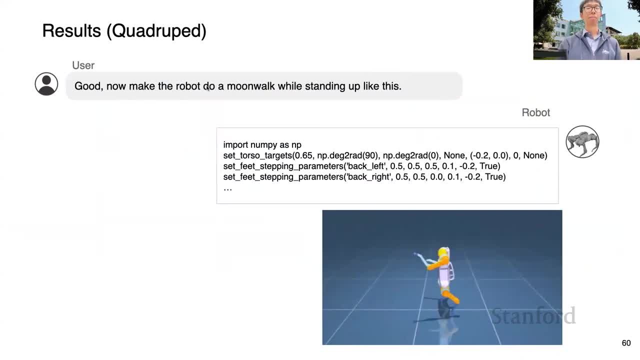 make the robot stand up on two back feet like a human, All right. And then now we are a little bit more ambitious. We know it can stand up. Can we make the robot do a moonwalk while standing up like this? So a moonwalk is from Michael Jackson. 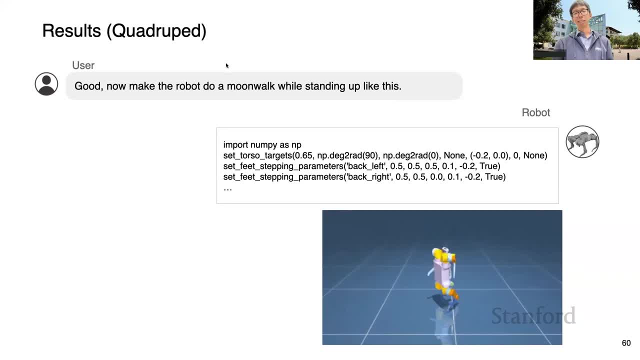 and it's very challenging. How do we make the robot to do it? So it generates the motion description and generates the reward code, But the motion is not so correct. Not exactly what we want. The nice thing about using a language model and 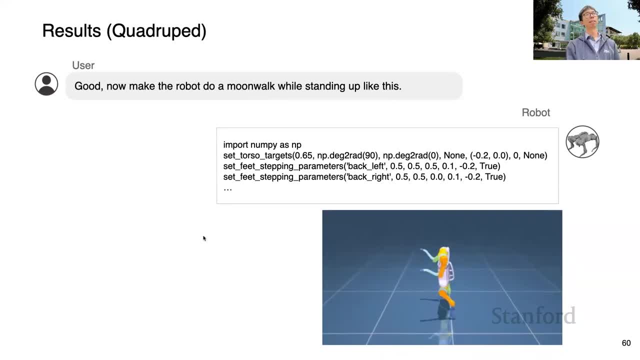 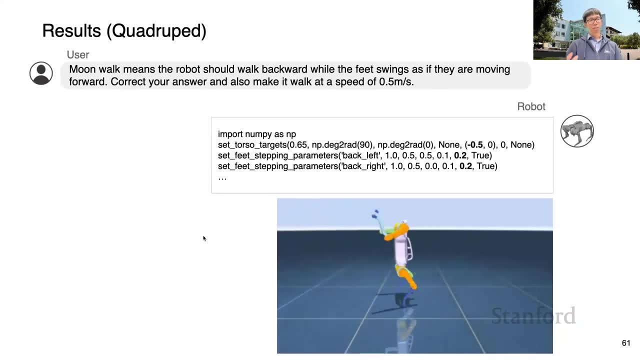 using the reward function is that you can coach the robot. You can go back and explain what went wrong and ask the language model to fix it. So now we can actually say you're being very patient. You say moonwalk means the robot should walk backwards, while the feet 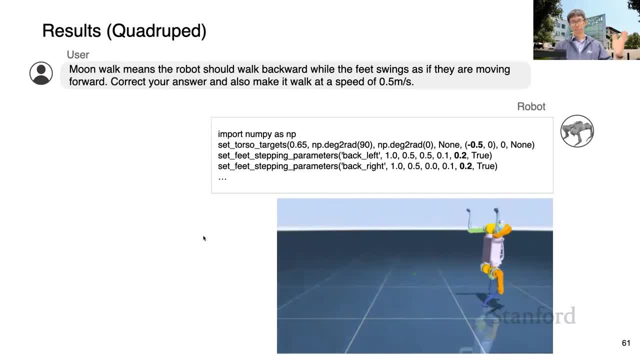 swing as if they are moving forward. Such a great explanation, Kudos to my colleague And correct your answer and also make it work at the speed of 0.5 meters per second And after you like being very patient and give it the right instruction. 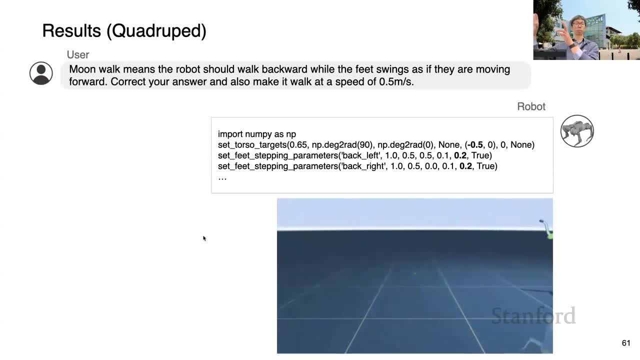 it's able to modify the reward, the motion descriptor, and also generate the right set of rewards to make this happen. And now you can teach a robot to do moonwalk just by using the language as an interface. And one day we'll be able. 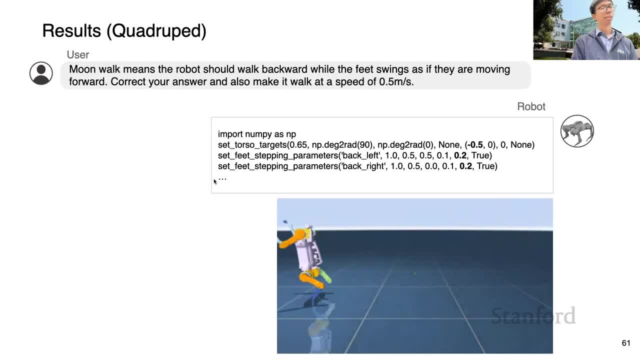 to do this on the real robot as well. Yes, So the previous session we showed how the moonwalk works with state numbers and you're constraining them to state numbers Here. how do you prevent it from just hallucinating in some program? 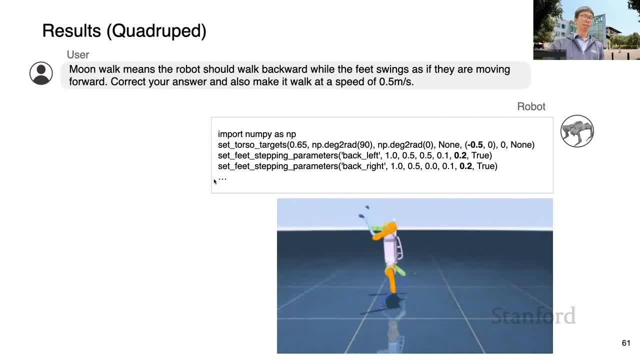 Right. So that's a great question. In this work we are not preventing it to do hallucination in a programmatic way. We have a set of system prompts or a set of rules. that is explaining the API. After all, the reward functions. 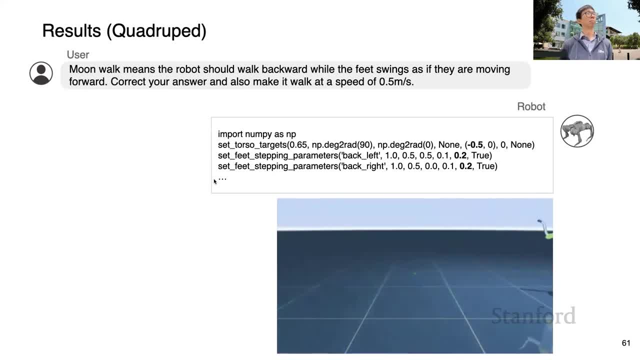 need to be able to be compiled by the optimizer and then like: yeah, so we do need to have some check. What's more, if it doesn't compile, we can just give the error message to the language model. It doesn't have to propagate all the way to the motion. 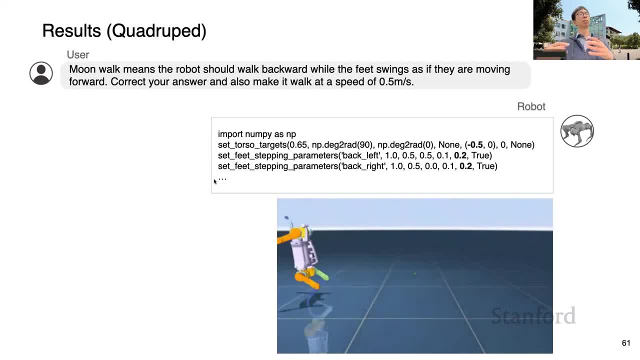 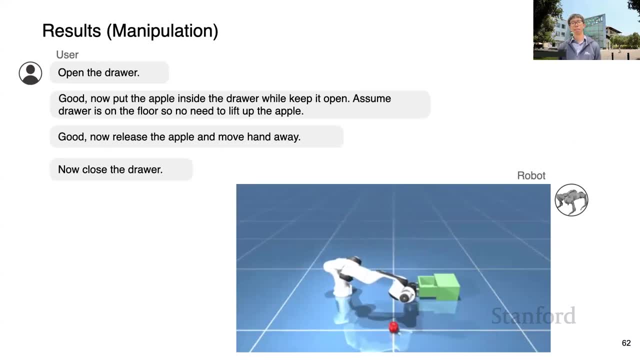 descriptor. It can stay at the reward folder. If there are errors, please fix it. So after that it should be able to fix it. We can also chain multiple tasks together using this framework. We can say: open a drawer, take the apple, put. 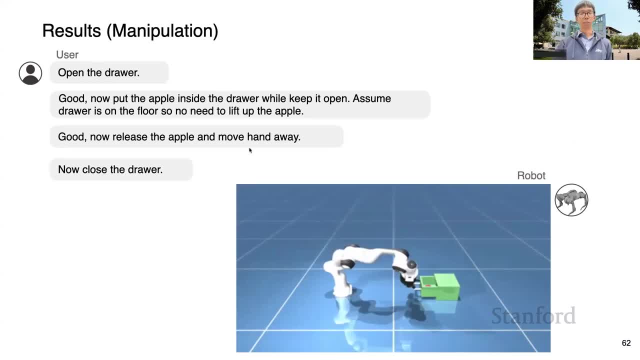 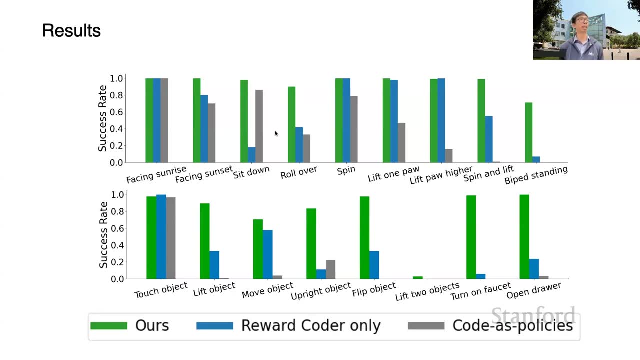 it into the drawer and close the drawer, and it will be able to do that. So we tried that. just using reward coder is not good enough. It's rather our two-stage prompt is really, really helpful. I think that's another inspiration for other fields, like when your domain 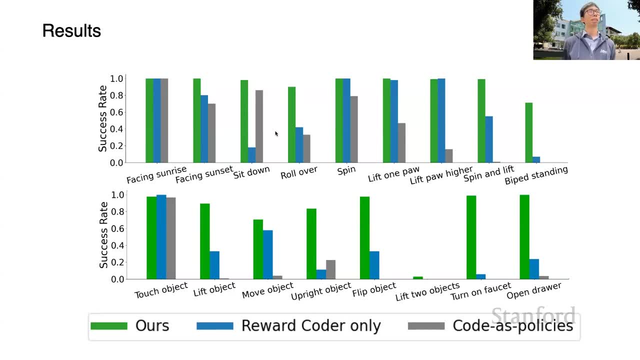 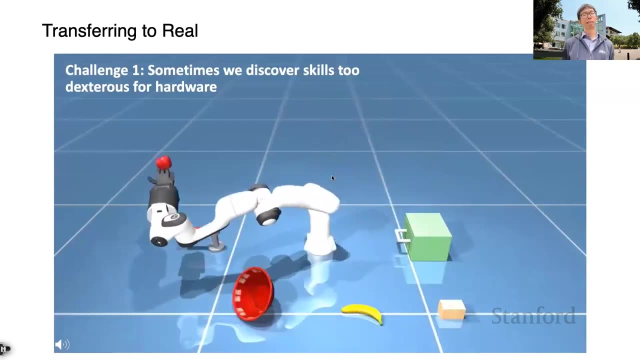 is too different from language domain. maybe it would be good to find an intermediate representation and ask the language model to explain in that intermediate representation before directly go to a more obscure representation. And finally, we want to transfer this to the real world. but there is a 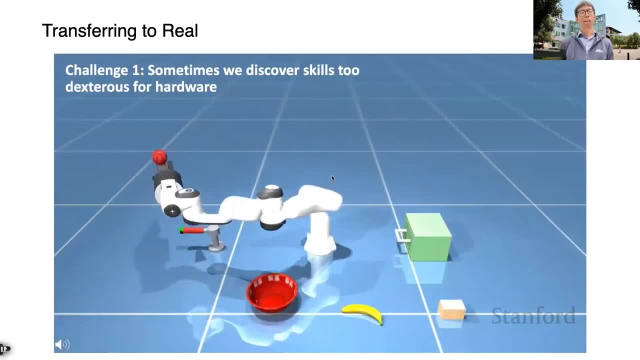 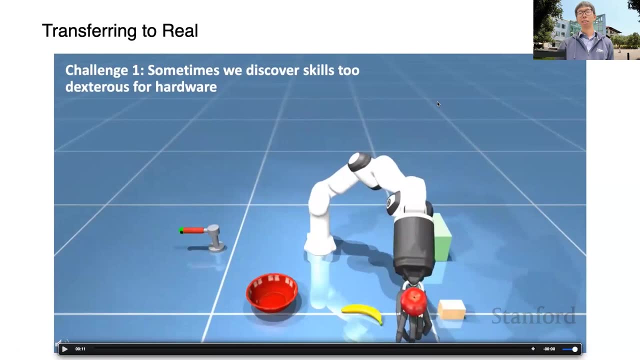 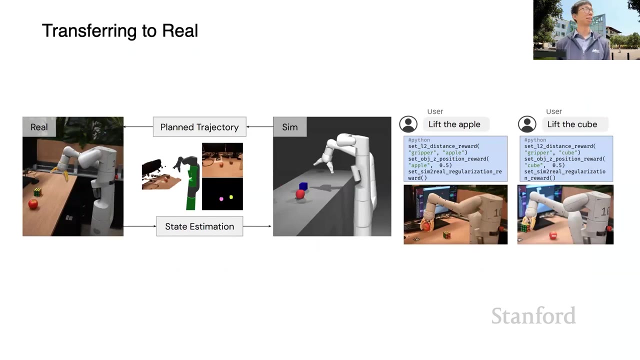 challenge In simulation. it might generate actions that are too dextrous, like this thing is not possible to do in the real world. So we add a few more regularizer terms to stabilize the motion and we also run some state estimation on the real robot. 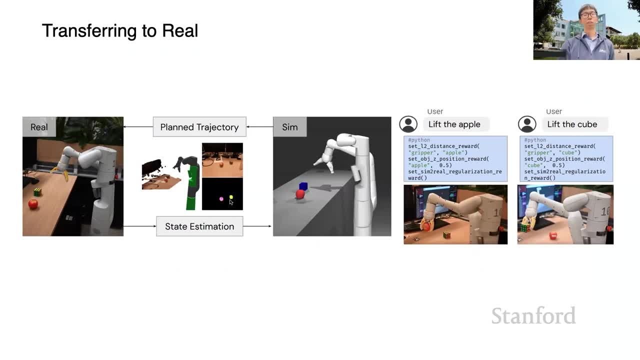 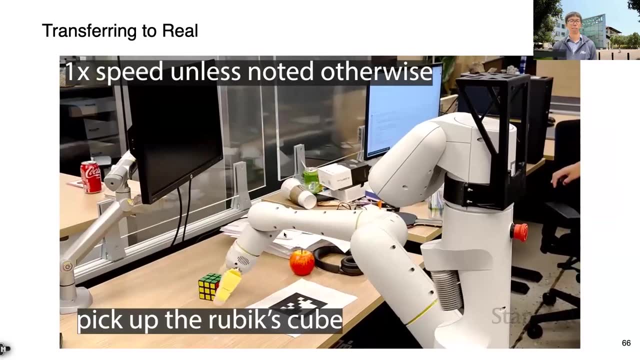 so that they understand where is the cubes. and then we can in the simulation map the motion and then achieve it in the real world. So here are some of the execution in the real world. So you can say, pick up the Rubik's cube and it will generate. 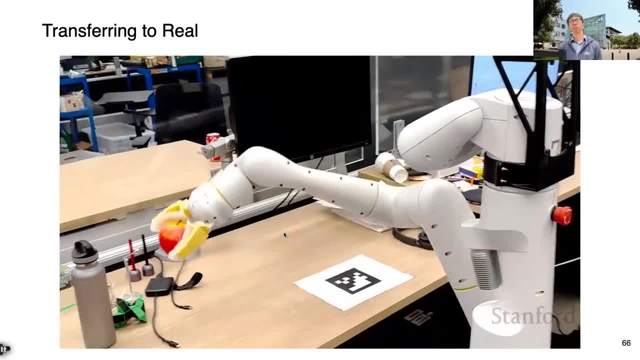 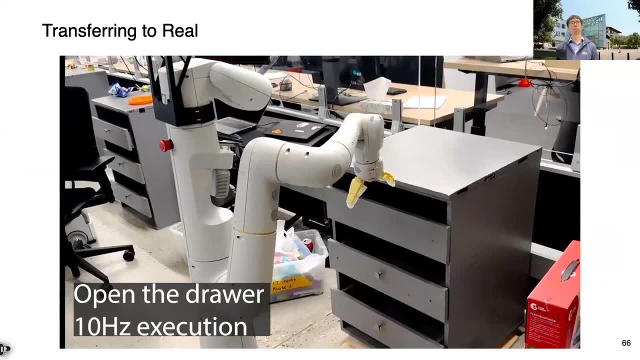 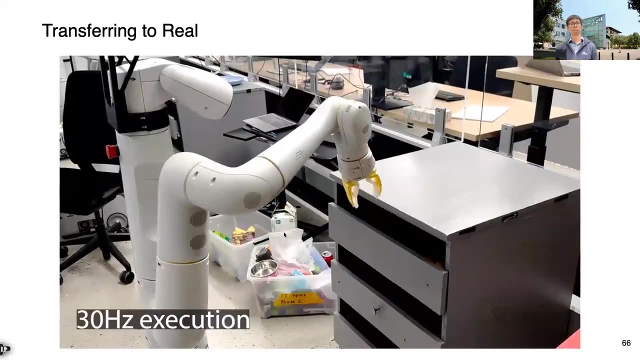 the motion to pick up the Rubik's cube and the double. This is quite different from RT2.. The motions are quite smooth. It's quite fast. It's much faster than 3 Hz, So here it can do 10 Hz or even. 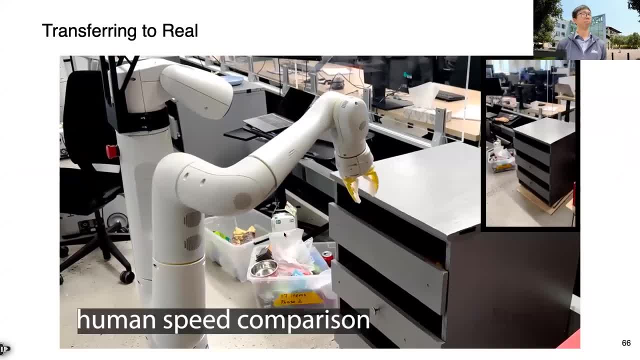 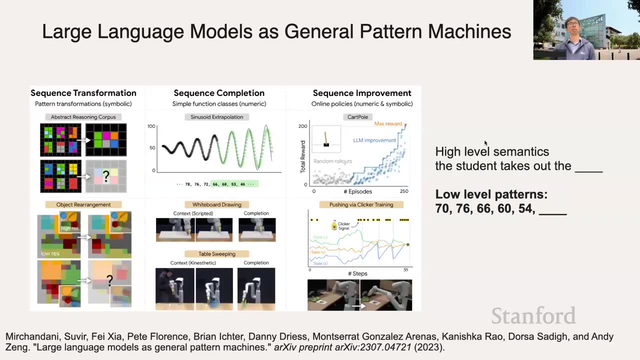 30 Hz, So it's comparable with human speed. Alright, so that's the language cue reward. There's one last thing that I want to talk about in terms of finding a new interface. So a lot of time we have been thinking about language. 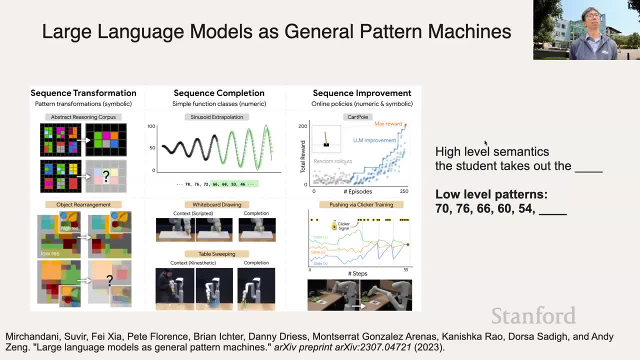 model as a semantic engine, a semantic machine. It understands semantics. So, for example, you say the student takes out the book, you will say: book like language model is able to reason about such a sequence. But if you do low-level patterns, like if you just give it, 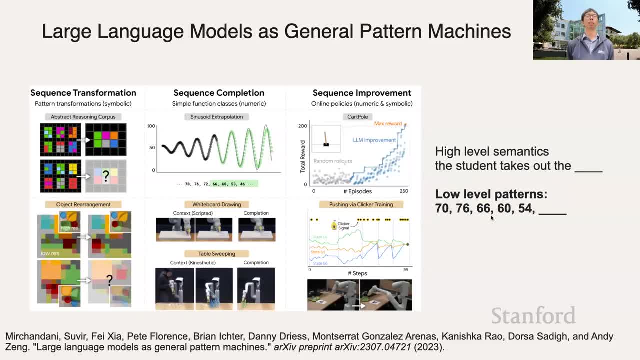 obscure numbers. what can you do? It's actually a low-level interface And we can open up the low-level interface of language model and ask it to do robotics tasks. So in this paper, large language model as general pattern machines we explore. 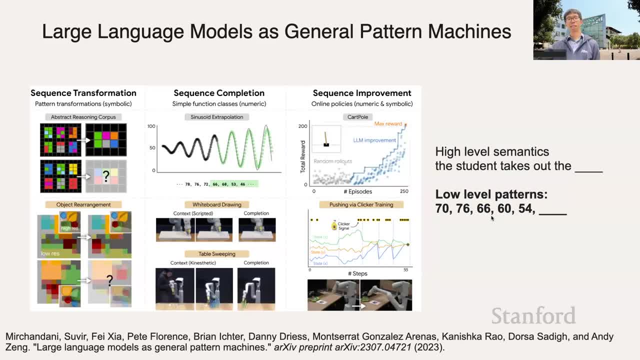 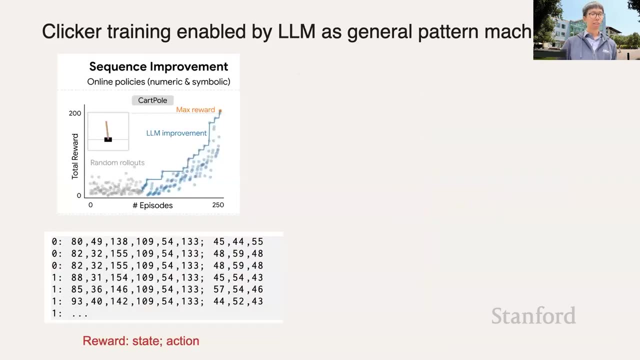 using the low-level interface of a large language model, essentially asking it to reason about different sequences, And it's surprisingly quite effective. And it can solve tasks like the ARC challenge and the PCFG And it can even do sequence improvement. So I will dig a little bit. 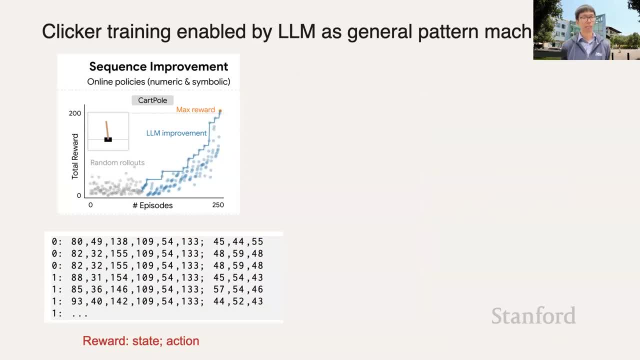 into sequence improvement, because that's quite relevant to robotics. So sequence improvement is that you prompt the language model with state action and the reward tuples And you just prompt it with higher reward and see if it can generate actions that achieve the higher reward. 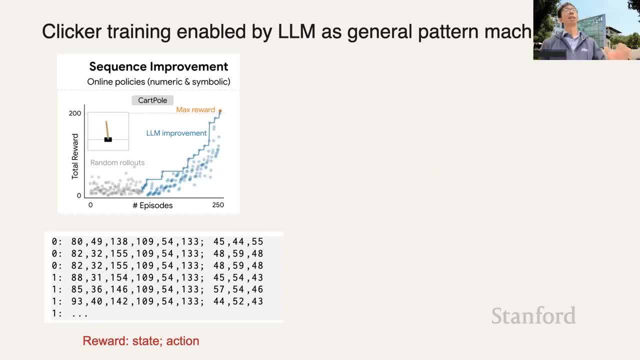 So it's doing reinforced learning or reinforced learning-like thing, but in context. So this is quite amazing. So previously you would need a dedicated algorithm collecting data, replay buffer- to do this reinforced learning, But now you can just build everything in the language model. 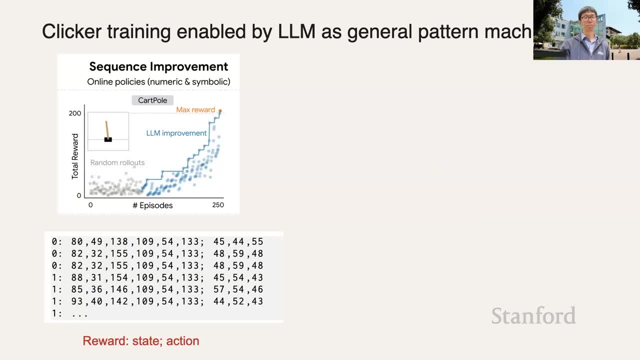 context by leveraging the low-level interface of a language model And with that we can actually do something like clicker training. So if you are not very familiar with clicker training, it's how you train a dog. You can have a dog and you can. 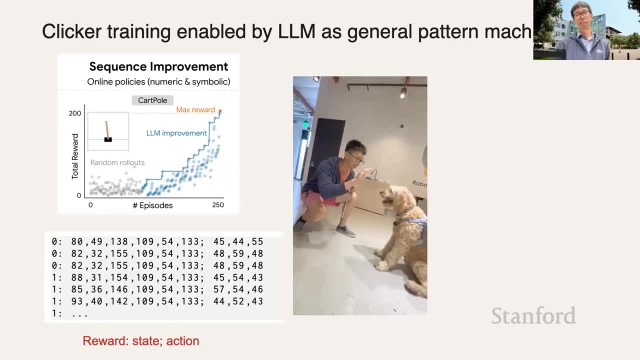 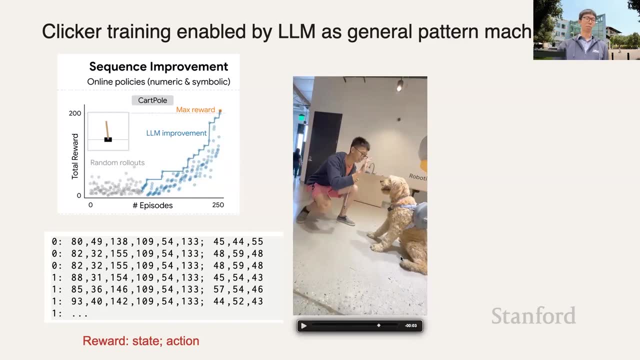 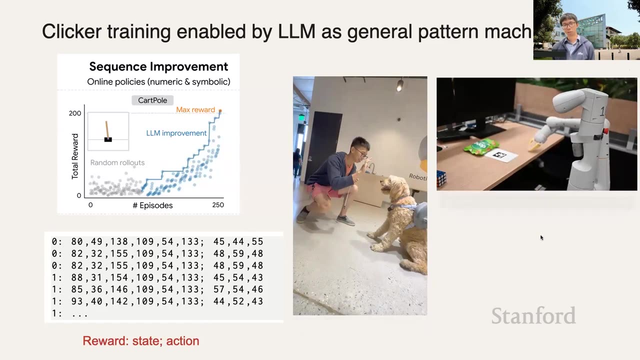 when it does the right thing, you give it a reward by clicking So you can. so the clicker training is giving the agent a reward, And we can now use clicker training to train robots as well. So here the robot is exploring. 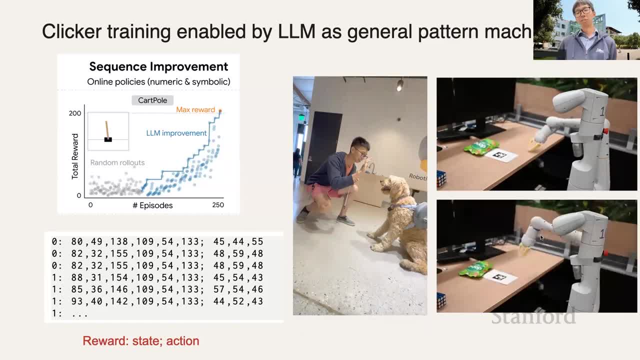 but I would give click when it does the right thing or towards the right direction, And over time it will be able to push the bag of chips, which is the objective of this training. So you can do this entire decision transformer-like operation, but purely in context. 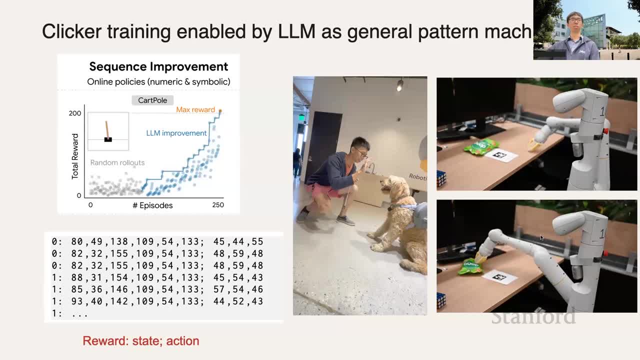 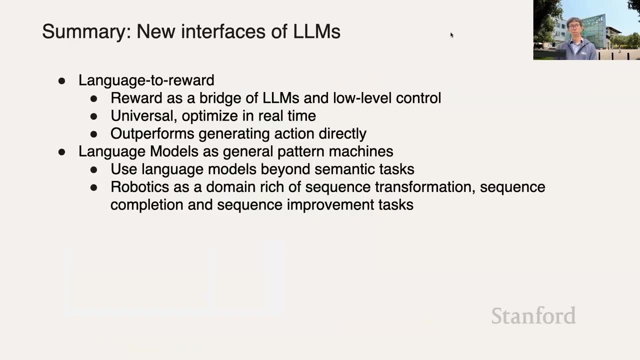 By just giving the language model a bunch of patterns and ask it to figure out what is the regularity of this sequence, And this way it can generate new actions to improve previous sequence. Alright, so for the language model we can find new interfaces that are more. 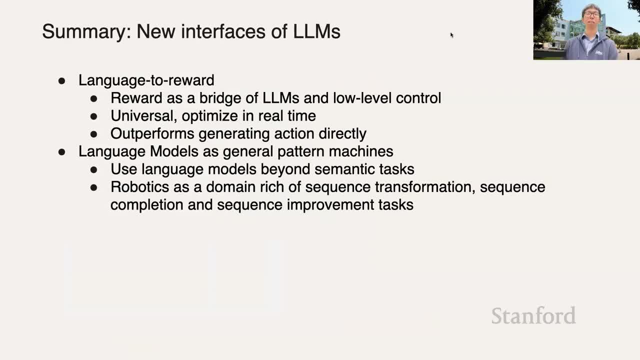 suitable for teaching it. low-level skills Reward is a bridge of language model and low-level control and we can fully leverage it as a universal interface and we can optimize in real time. Sometimes it outperforms generating action directly, so it really motivates to use. 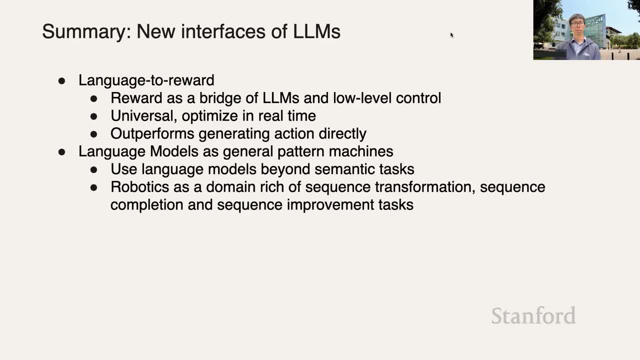 reward functions as an interface And in the language model as a general pattern machine. we can use language model beyond the semantic tasks. We can ask it to reason low-level things And also robotics as a domain is rich of sequence transformation and sequence completion and sequence improvement tasks. 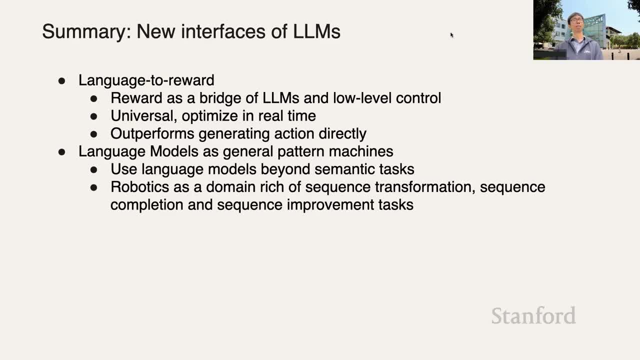 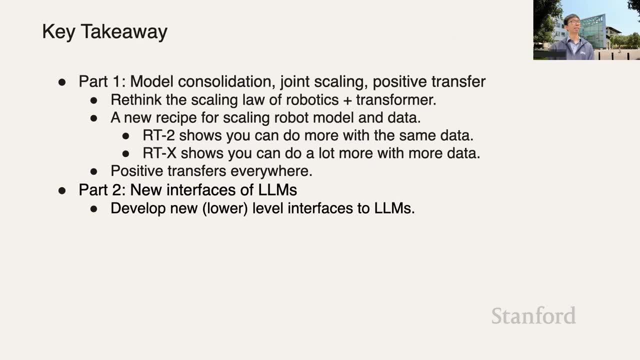 So we can really study the lower-level mechanisms of language models, And the key takeaway is that for this talk is that we are seeing more and more use of foundation models, not only on the semantic reasoning side of robotics, but more on the dextrous. 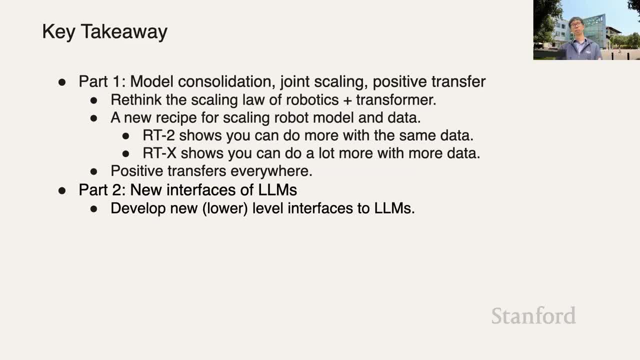 on the generating actions on the lower-level embodied intelligence side of robotics And we need to rethink the scaling law of robotics and transformer. How do we scale it with limited amount of data? We have a new recipe for scaling robot model and data in RT2. 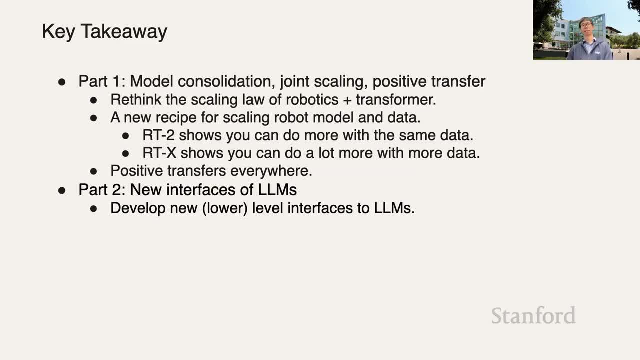 which shows that you can do more with the same data. with essentially RT1 data plus internet data, you can generalize to a lot more things, And RTX shows that you can do a lot more with more data. There is also benefits to collect more robotics data. 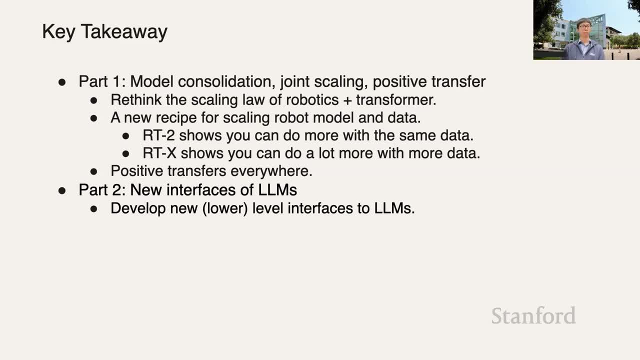 And there is positive transfers everywhere. And part two, in terms of new interfaces for language models, I think it's worth for the robotics field to think about developing new and lower-level language models which facilitate learning low-level skills. With that, I would like to conclude. 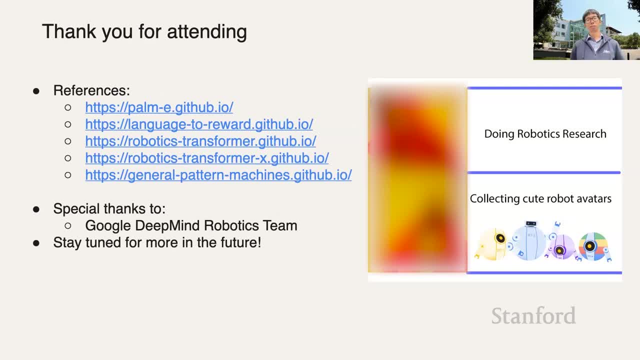 my talk and, if you find it interesting, there are a lot of references for you to look into. and special thanks to my team, Google DeepMind Robotics team. So we are at the forefront of developing foundation models for robotics and stay tuned for more in the future. Thank you. 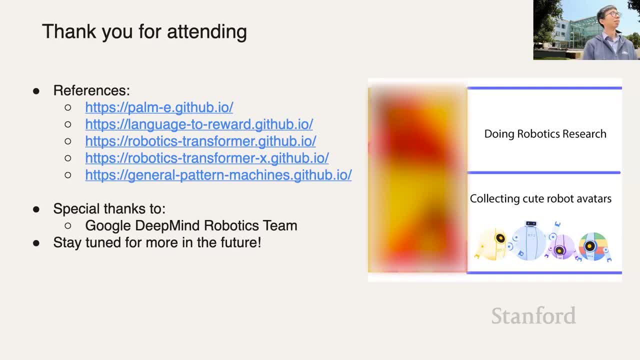 Yes, You mentioned that load numbers are difficult for a large language model. If you're just generating the action tokens themselves, like no rocks or whatever you had as an example, why don't you just have a linear layer appended to the transformer? that would just generate numbers? 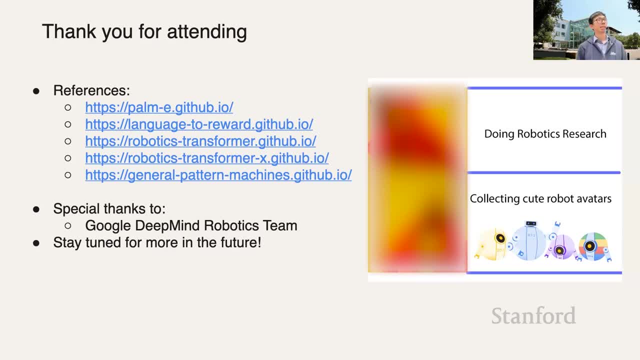 from here. Yeah, The question is that if we are the large language models have difficulty understanding numbers. why don't we use a linear layer to output the action directly? I think language models are difficult to understand numbers, but sometimes we still want it to. 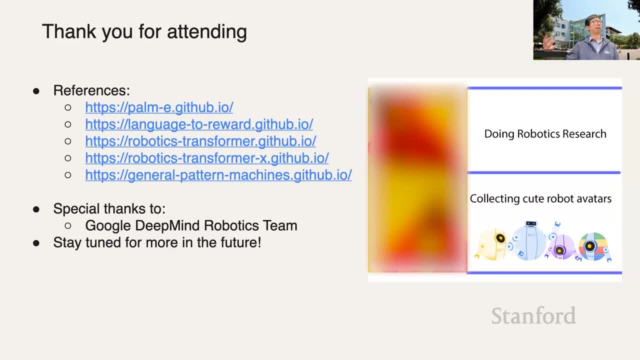 bring in knowledge from the pre-training mixture. If I have a new layer, that new layer is not present in the pre-training, so how do I expect it to transfer? I think that's an interesting question, But at the same time I don't necessarily think. 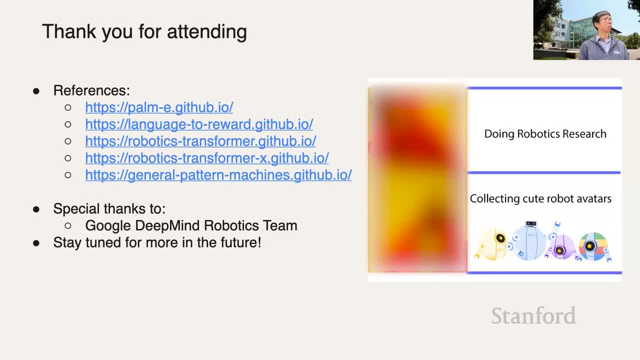 using the raw numbers is the right interface. We probably could do some action representation, learning to learn a representation and the language model can output that representation. So we're still trying to figure out what is the right representation. So among the representations that we haven't tried before, 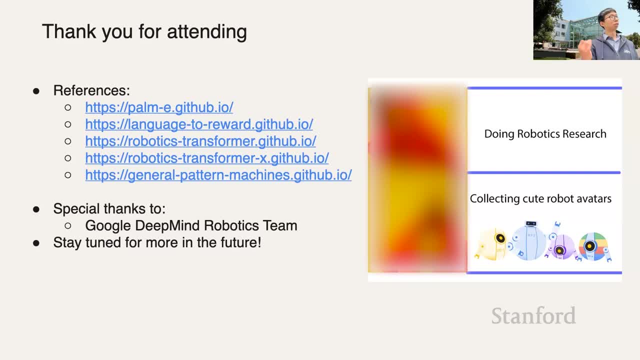 like decimal numbers, float numbers, extra tokens. we find that just using numbers or extra tokens would be good enough. Yes, Alright. From where do you think your children can average their rettings? Do you think Both directions are more promising, or 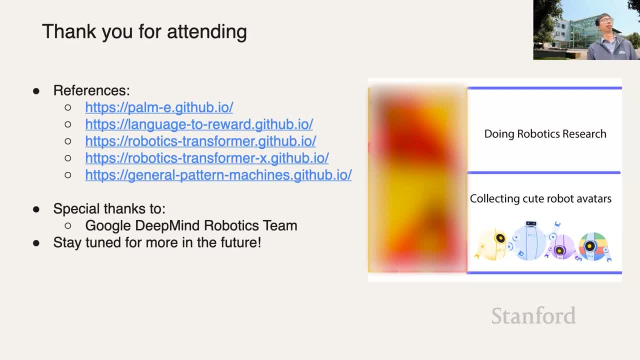 Yeah, I think both directions are worth exploring. There are different advantages of generating action directly. I think it borrows aggressive nature of like language modeling and it aligns with a lot of other tasks like visual question answering, really well. the limitation is that then, when you're generating 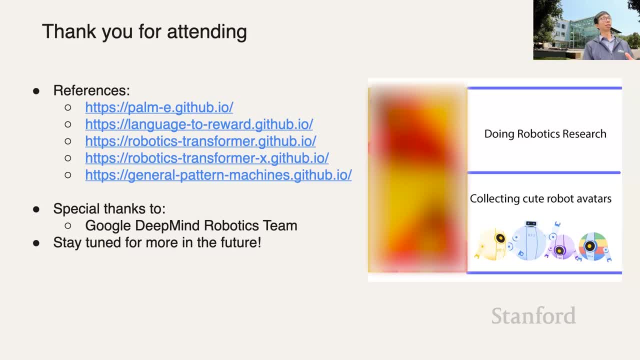 actions. it's heavily irregularized. can you generate dexterous actions? that is so out of distribution? that is kind of difficult. the language to reward actually brings a page of the book of traditional robotics like right, this optimization based or model predictive control. so, and you can. 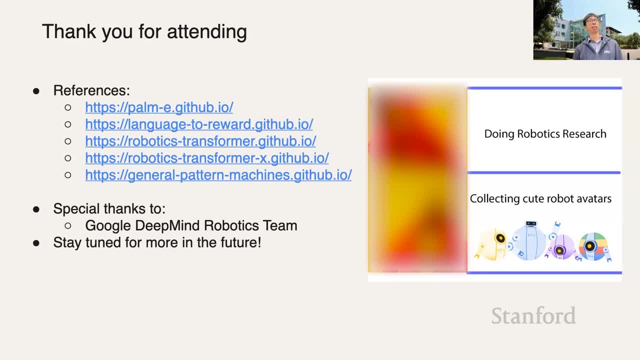 also take into, let's say, safety constraints. uh, more, more, more easily it can generate more diverse actions. maybe one recipe is to generate a lot of data with the language to reward system and distill them into a transformer, because then you're imbuing your large language model with. 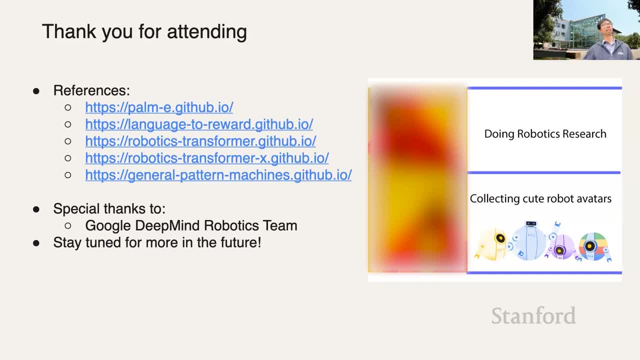 all this other desirable uh, the language to reward system itself. i don't know how scalable it is, like it's. we're not fine-tuning language model, so maybe you are limited to what? the uh? you are at the mercy of the training data of the language model, the. 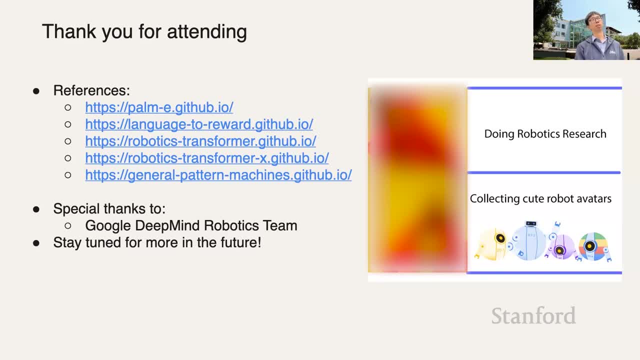 language model can do uh moonwalk, because it knows what moonwalk is. it roughly knows how that, uh like how to do that. but if you want to scale to completely new things, maybe you can use the language to reward, to boost up your data generation and then put into like the other policy. 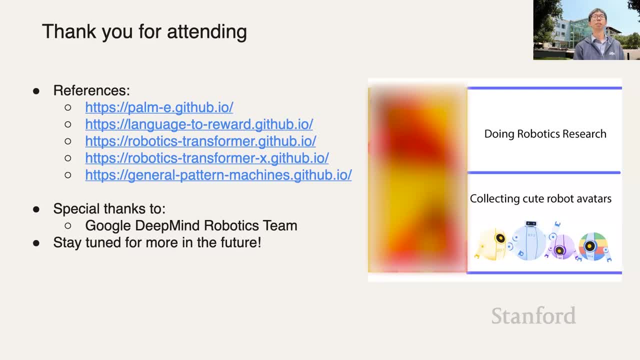 yeah, i think that's a good question. so this, the scaling of the, the scaling being the end of the lecture, uh, that as a joke, but as i'm being quite serious, like it's actually a promising recipe. so, uh, we have been, we've been. uh, everybody is believing in the uh power. 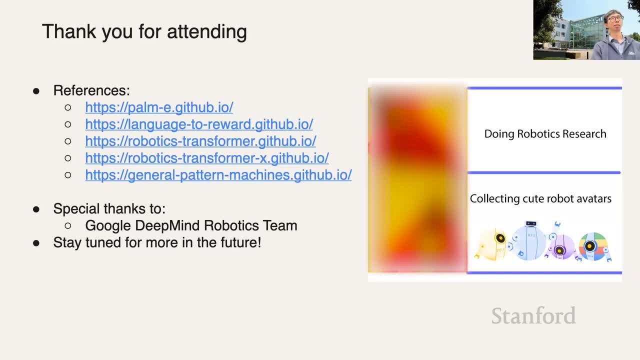 of the scaling rule. so just by giving it more data, giving it more compute, you will see interesting kind of capabilities coming out right. yeah, possibly like gbd to gbp, a little big jump. so do you think like, uh, yeah, that is for robotics to have that jump that we can. 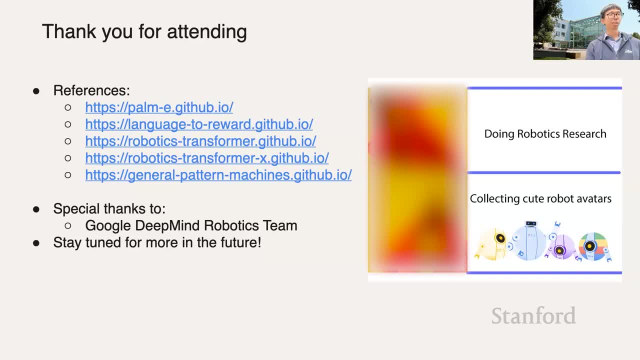 where do you see the capturing? yeah, um, i still. i still think we are not quite like, we don't quite have enough data. i think that's still probably the biggest bottleneck. so we are trying to find ways to do more with limited data and we are trying to collect more. 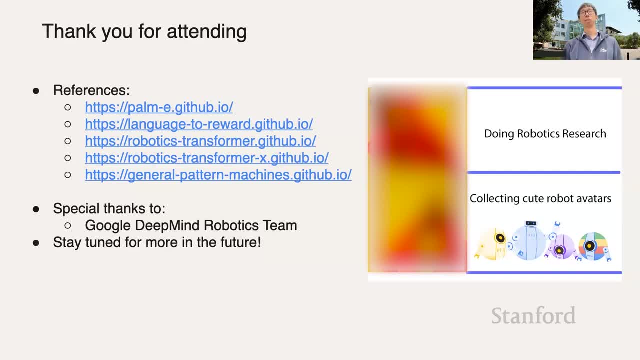 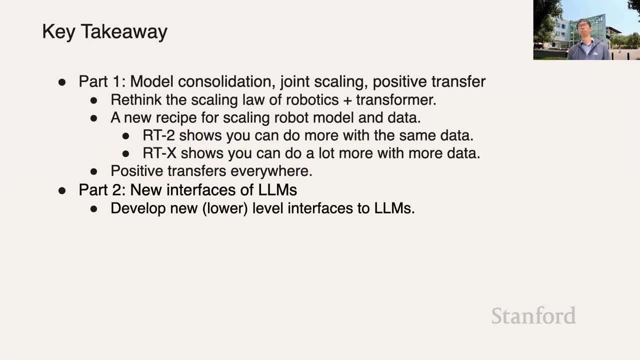 data and i think it needs some time for for us to accumulate enough data. and currently i say: uh, we have science of life for positive transfer, but in language models people don't talk about positive transfers anymore because it's so commonplace, right you? you see it everywhere. um and robot. 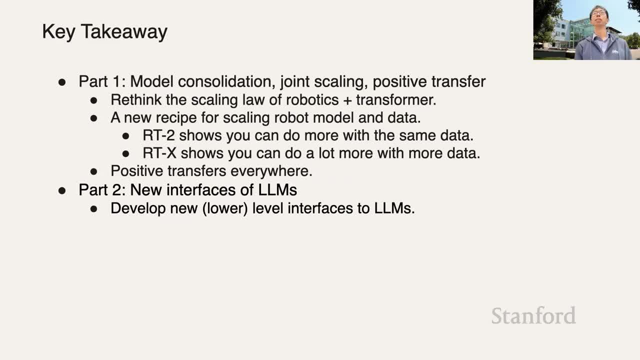 robotics is not at that stage yet. yeah, i think that's a good point. how much has your team thinking about safety and alignment? yeah, are you just like right now, like relying on kind of the ethics that emerge from the large language models, like it won't, you know, tell you to kill someone to achieve that? yeah, that's a very good question actually. 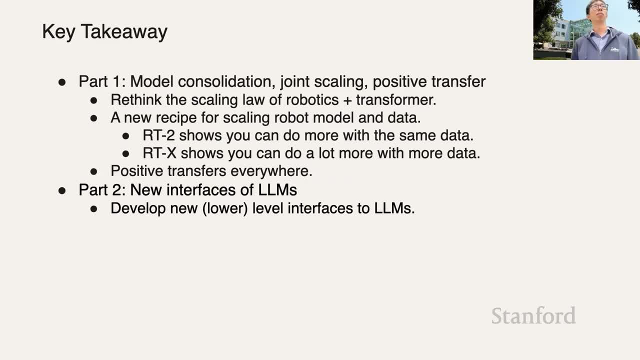 we take safety very, very seriously because all of the the other domains of developing language models, um, it doesn't have direct like impact on on the physical world but here like it could have potential harm to to human and to the environment. and gary marcus actually gave a comment to previously to our work that what if you say um bring. 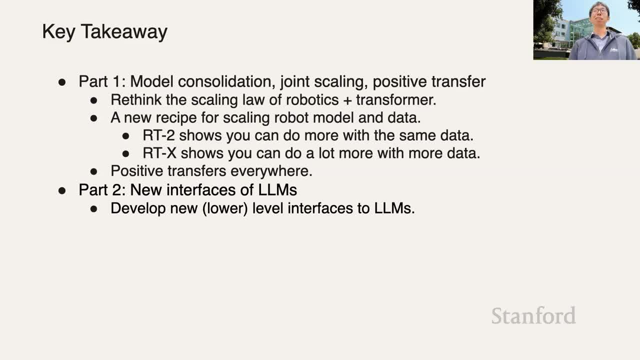 bring out the bowl, feed the cat and put it in the dishwasher. well, let's put the cat in the dishwasher, right. if it misunderstand, actually it will have a catastrophic uh um failure case. um, we, we take uh safety carefully by designing, like hardware and software, safety layers and 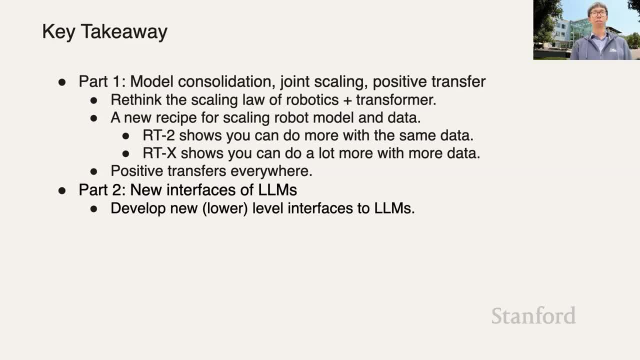 there are also some constitutional, like safety, uh thing that is coming out sometime soon. i cannot tell much details right now, but, uh, sometime soon we'll release some work. is it something like if there's a human like just don't interact? well, no, no, i think it's a little bit more nuanced and more 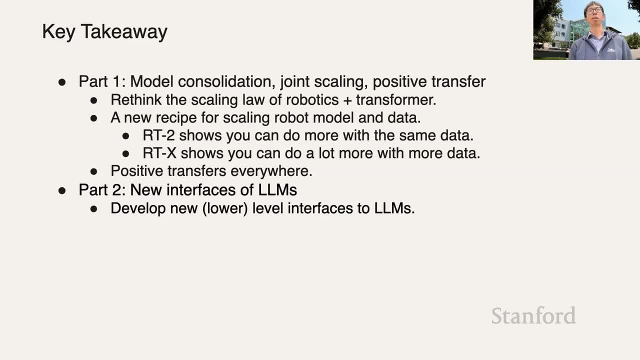 detailed than that? yeah, but we do take a safety quite seriously and in some of our experiments actually the robot's finger would break out off because it cannot apply enough force to an environment. so that's just yet another way of ensuring safety. can we have some like visual language model and 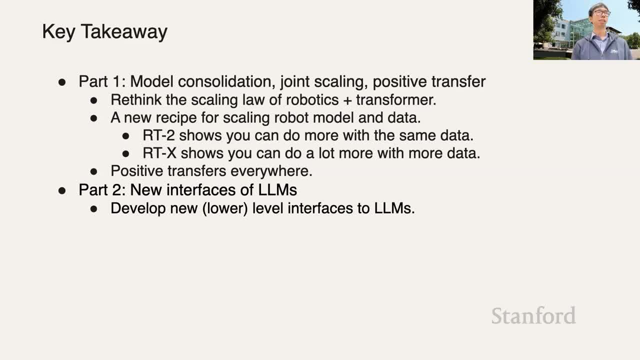 simplify them or something to establish on them, uh, the mode that they're going to apply, and maybe this is kind of like thanks for doing it, but right, right, yeah, i think it would be possible, and you might have to do a natural experience with it, but i think it would be a good way to do it. thank you for the great talk you.